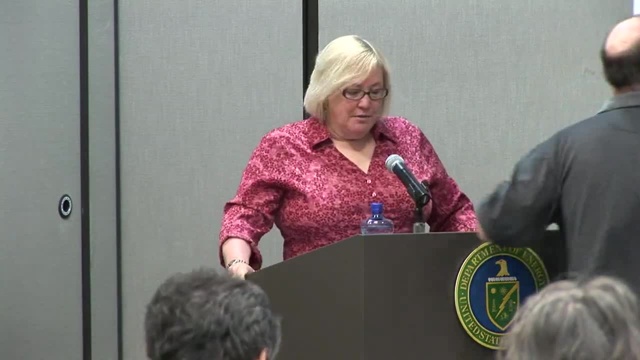 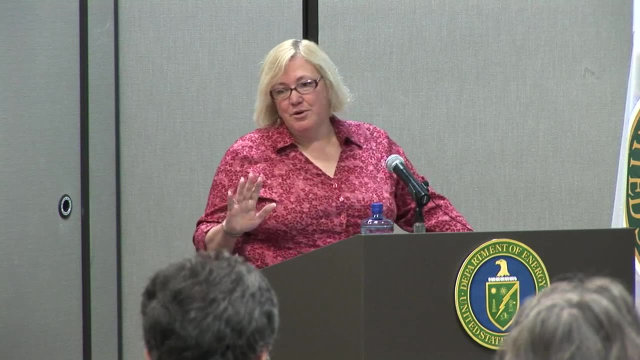 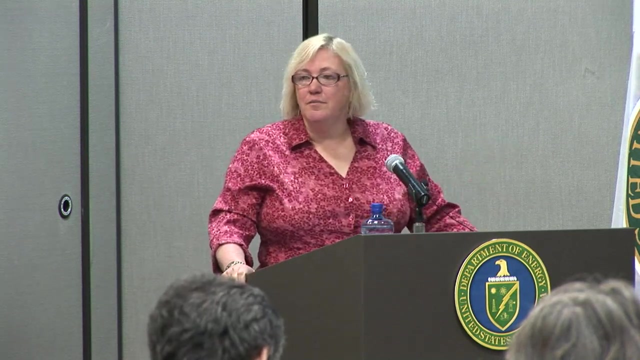 is some educational information about the topic of nuclear non-proliferation. It's a deeply rich field and we can only go through an overview here and give you some pointers to other references, And I'll try to tie back some of the comments that I make to some of. 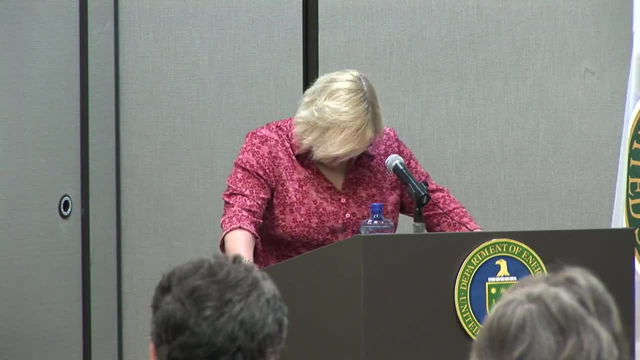 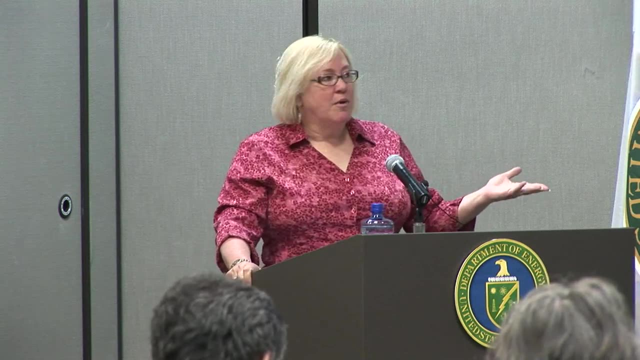 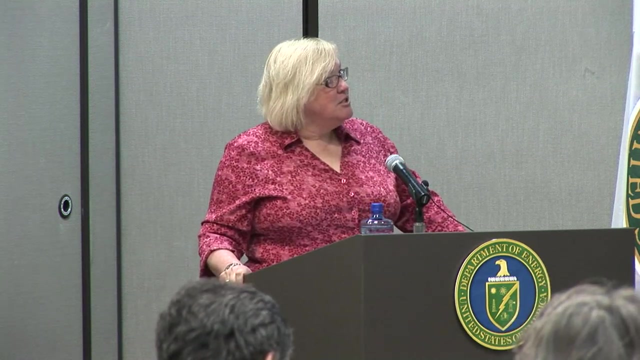 the other talks that we've heard in the past two and a half days. In preparing this material, I've relied heavily on open, available information from government type organizations, NNSA, Department of State, Nuclear Regulatory Commission, the United Nations and the International Atomic Energy Agency. There is no end to other information. 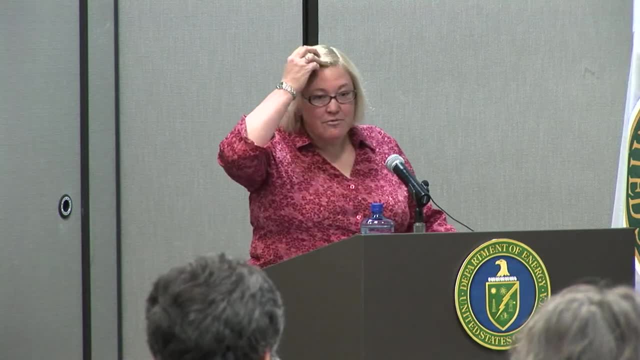 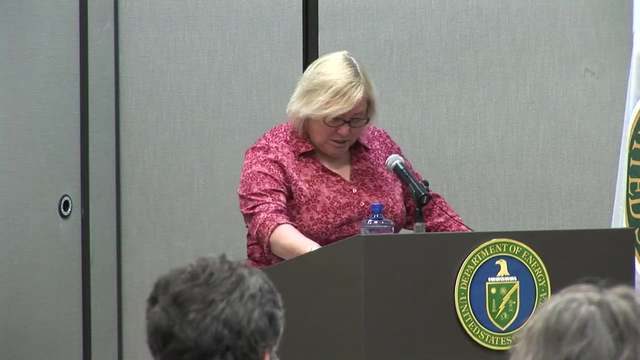 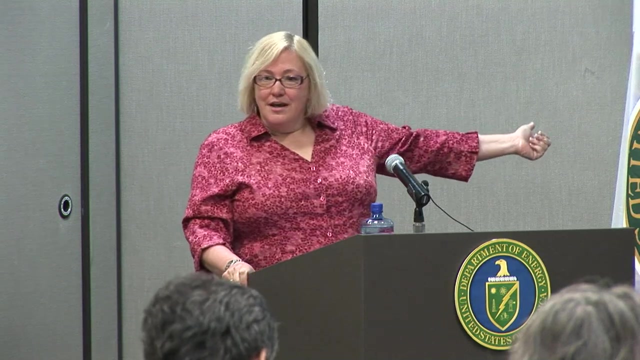 out there on the internet about nuclear non-proliferation and I'm not going to rely on any of that for my comments and I won't make any comments about other information that you might have from those sources. My presentation is completely unclassified, both in written content and 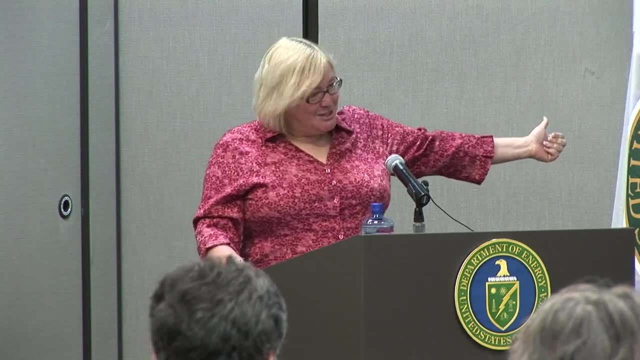 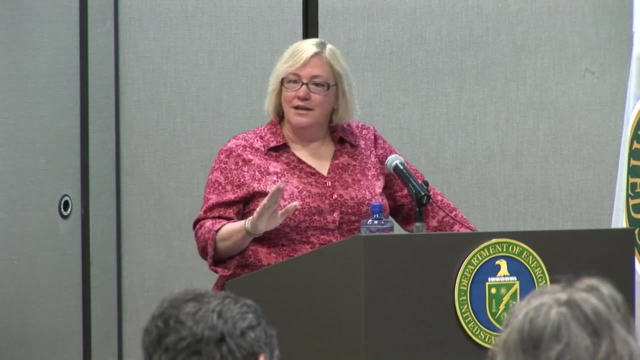 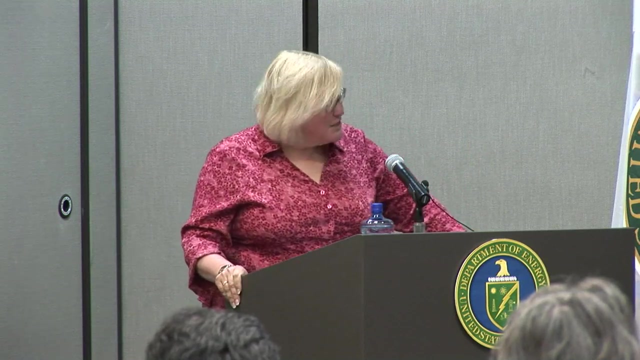 verbal content, and so will be my answers to your questions and we'll take it from there. I've tried really hard to clean up the jargon in here. If I missed something and you hear something you don't understand, call me on it and we'll take a minute and explain And 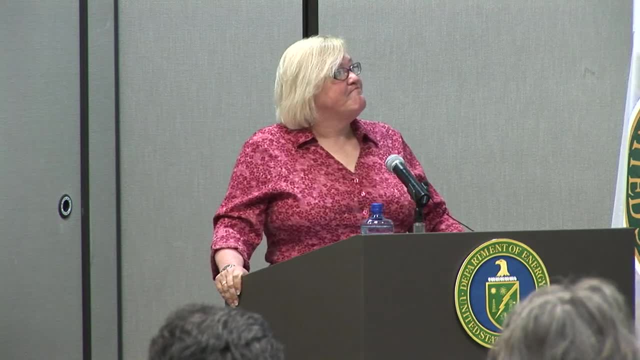 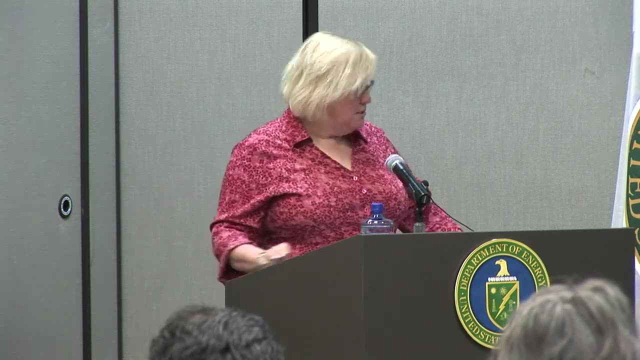 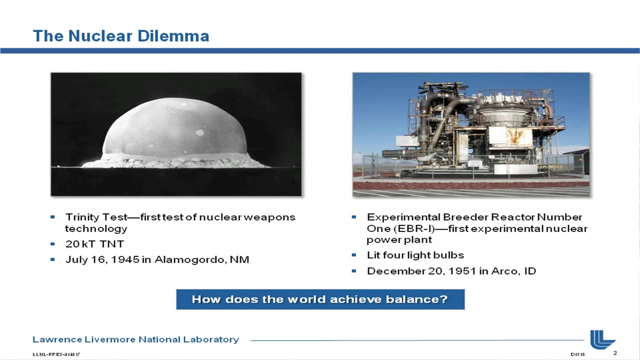 I'd also like to upfront acknowledge that I have borrowed a large number of these slides from other people, from other organizations. They're all acknowledged in the back of the talk, but we might as well do it right up front. Sixty-five years ago- last week in fact- in Alamogordo, New Mexico, the United States. 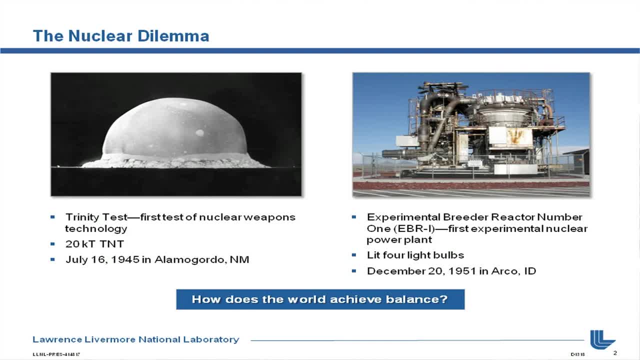 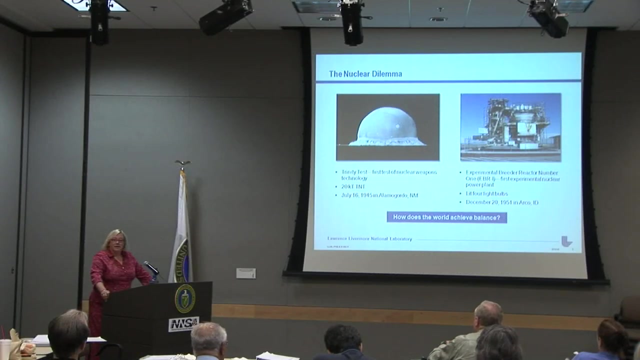 detonated the Trinity test, which was the first test of nuclear weapons technology here. It had the equivalent of 20 kilotons of TNT. Six years later in Arco, Idaho, EBR-1, Experimental Breeder Reactor Number One demonstrated the first use of nuclear power plant lighting. 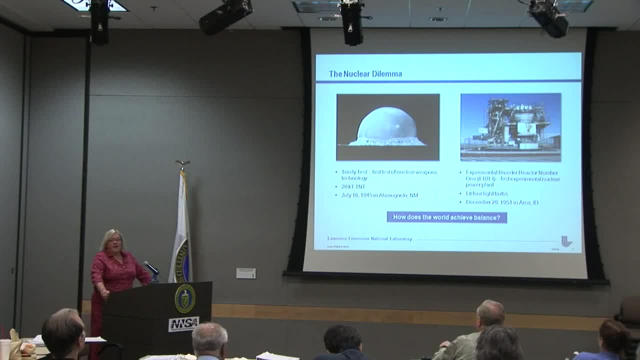 the equivalent of four light bulbs. And then, from that time, the world- and the United States- has sought to understand: how do you achieve a balance between the incredible destructive forces of nuclear fission and the incredibly benign uses of nuclear fission? That's the nature of what we're going to discuss today. I think you've seen over the past. 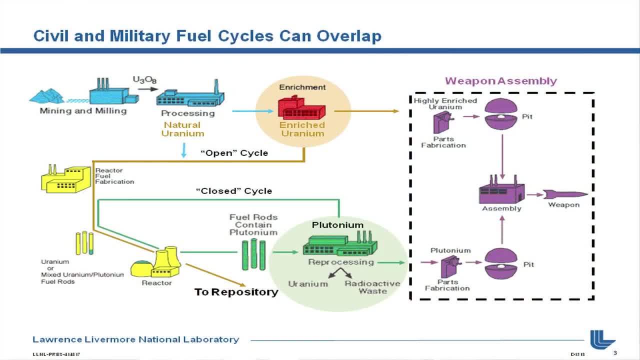 couple of days this chart before perhaps not what the civilian and the military fuel cycles overlapped onto a single diagram. We see over here the part that's specific to the nuclear weapons process, and then we've seen talks in all of these different areas over the course of the day and how we relate. 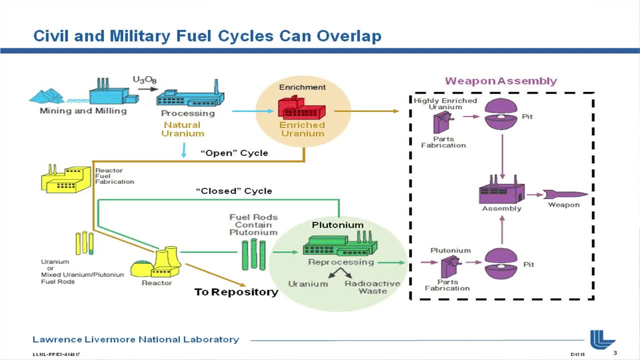 all of this to nonproliferation is what we're going to discuss this afternoon, Pointing out that the areas of isotope separation and spent fuel reprocessing- two topics that we've spent quite a bit of time discussing- are the ones that are the most sensitive areas. 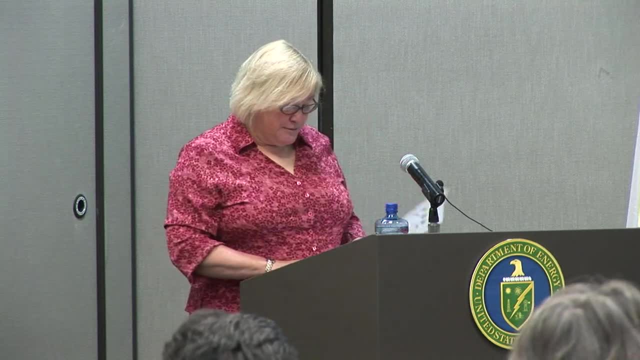 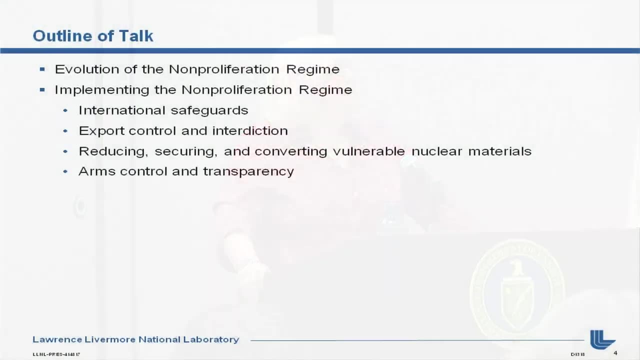 in our understanding of nonproliferation concerns. I've broken the talk into two parts. The front end is mostly, I would say, policy, and that is the evolution and development of the nuclear nonproliferation regime, both within the United States and in the United 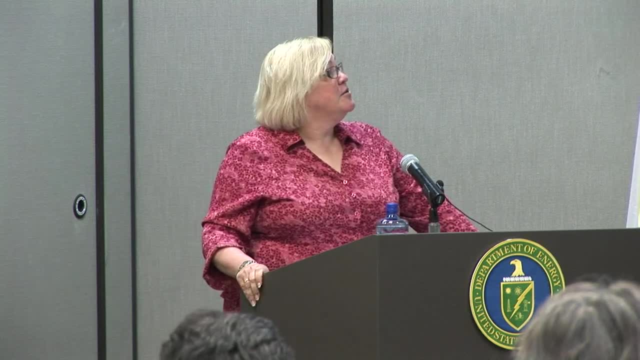 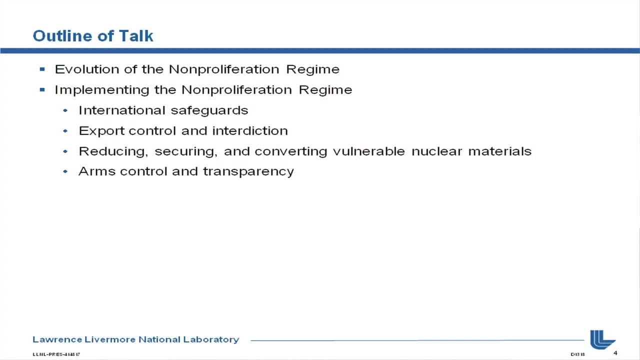 States and globally, and the role that the US plays in that regime. The second part of the talk, which will expand or contract depending on time, talks about some of the technical aspects that one would need to consider in implementing this regime. 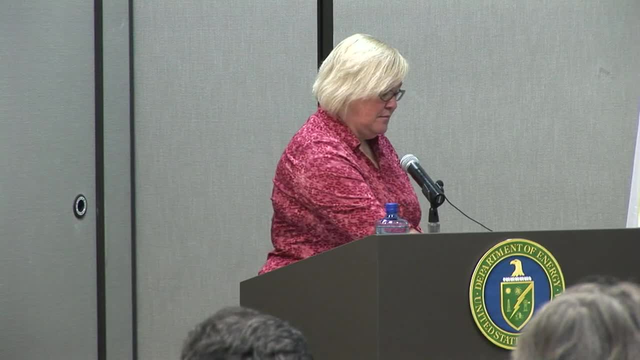 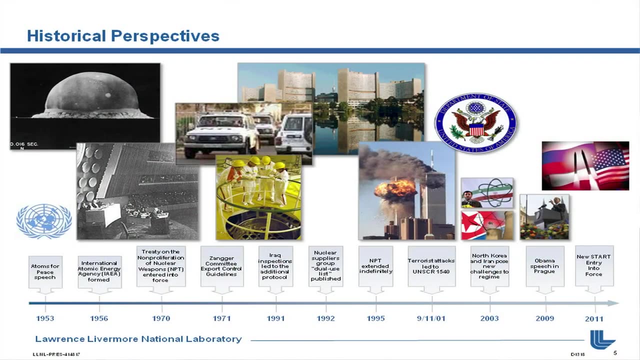 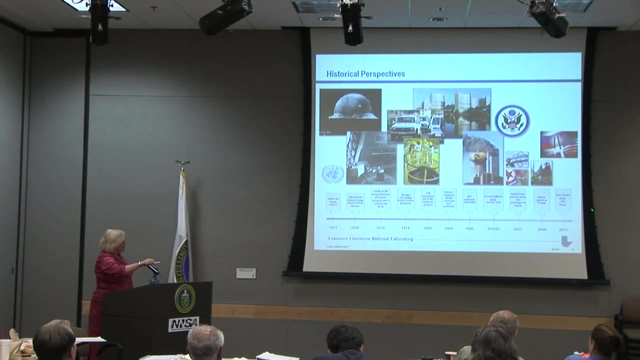 that we will define in the first part of the talk. This is the closest thing to a graph, It's a timeline. This is the organization of the policy part of the talk, and you can see here, spanning from the left, From 1953 out to as recent as February of this year. we're going to step through this. 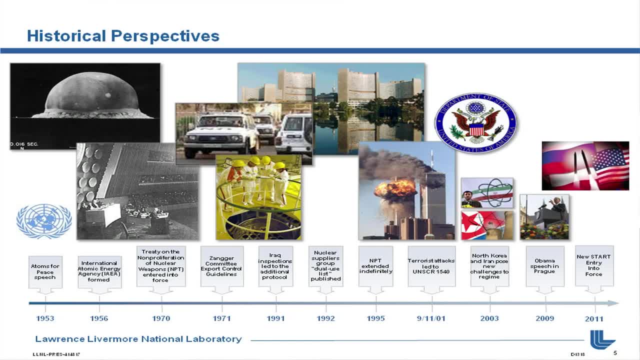 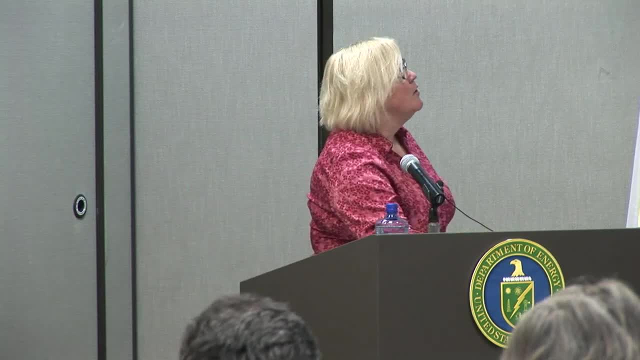 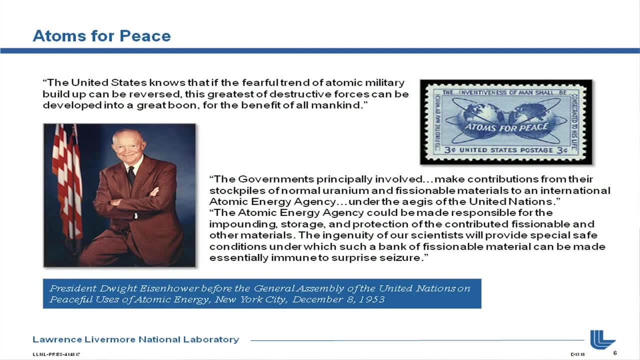 series of actions and reactions in both the US and in the global context. We've heard reference to this talk earlier in the short course. In 1953, then-President Eisenhower presented to the General Assembly of the UN a talk referred to now as the Atoms for Peace talk. 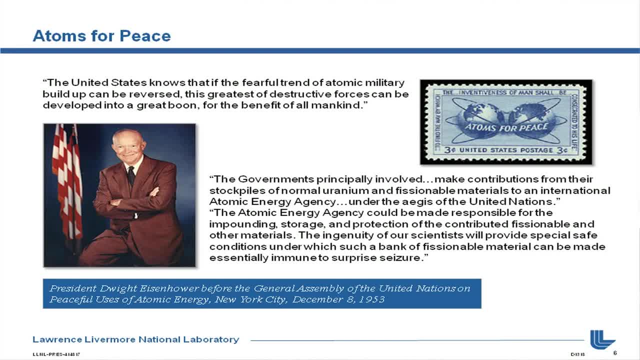 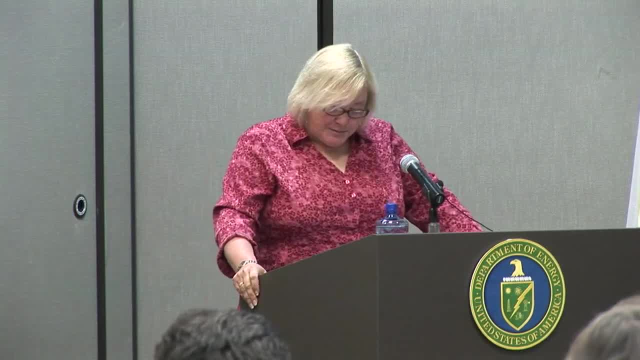 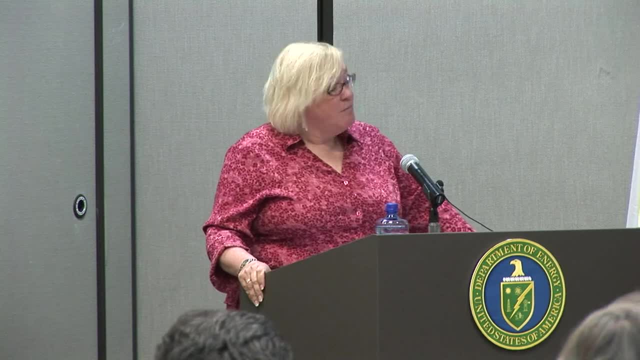 And in that talk he first addressed the fearful atomic dilemma that is, the balance between the peaceful use and the military uses of nuclear materials. And he talked about the United States knowing that if the fearful trend of atomic military buildup could be reversed, that this greatest of destructive forces could be developed for. 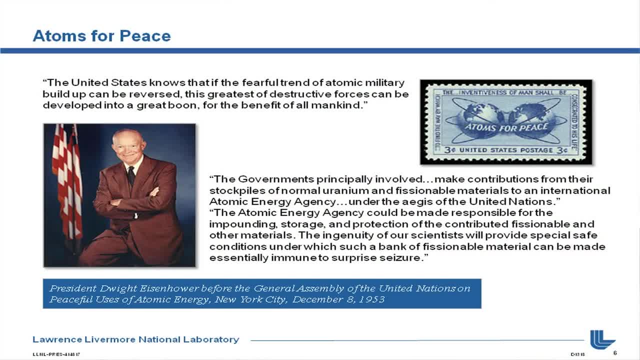 great boon for the benefit of all. He went on to say in this actually pretty short talk of, if you go back and read it, that the governments involved in the military aspects of nuclear material could make contributions from their stockpiles of the normal uranium and fissionable material to an international 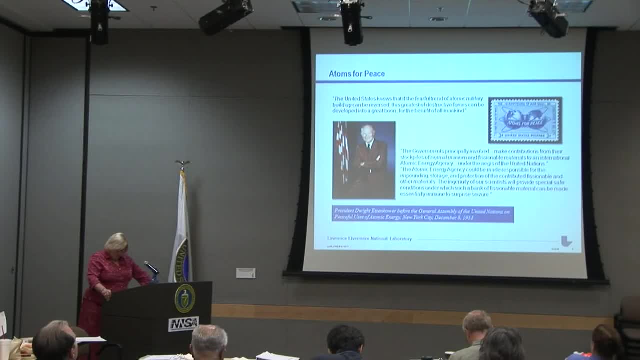 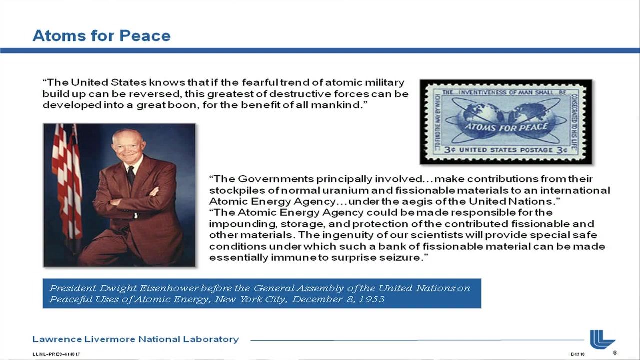 atomic energy agency that could be made responsible for impounding the storage and the protection of the contributed materials And that the- The ingenuity of the scientists in the indigenous countries could provide safe conditions under which such a bank of fissionable material could be made available and immune to seizure. 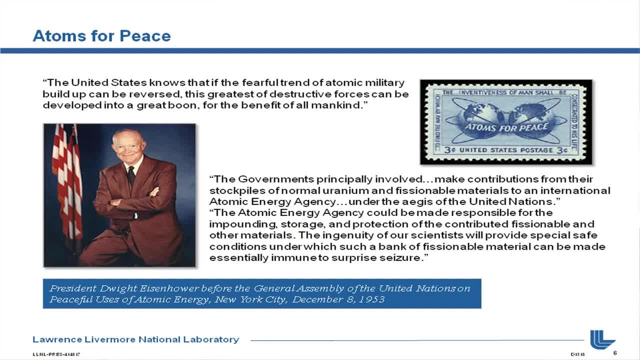 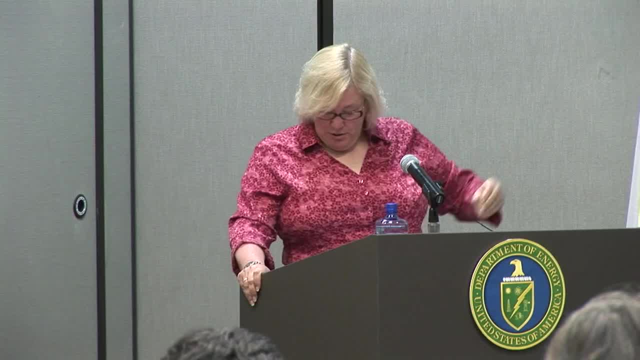 That paragraph there was the first and early suggestion of the formation of what became the international atomic energy and the concept of safeguarding nuclear materials. So in fact, following the President's talk, I'm going to turn it back over to you, Thank you. 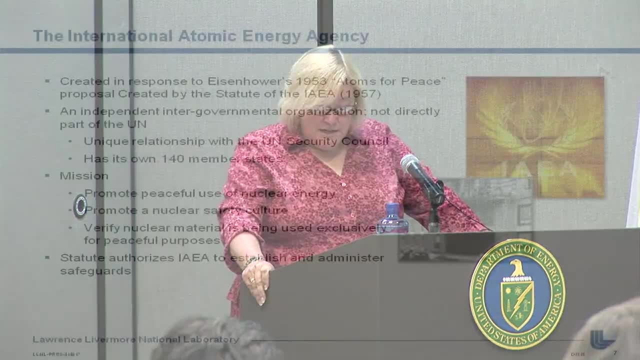 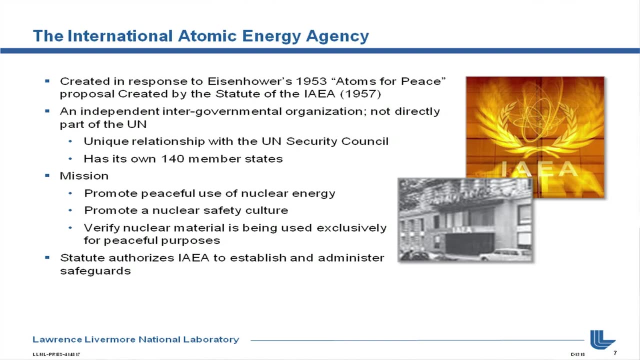 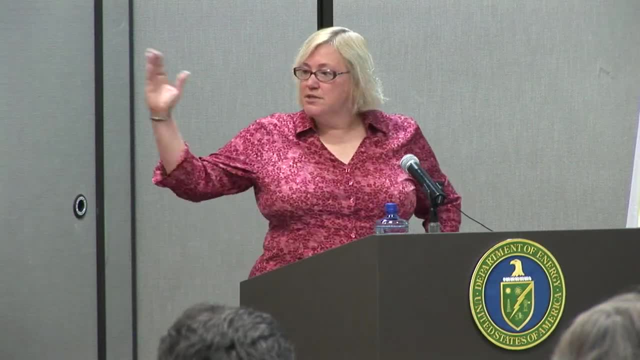 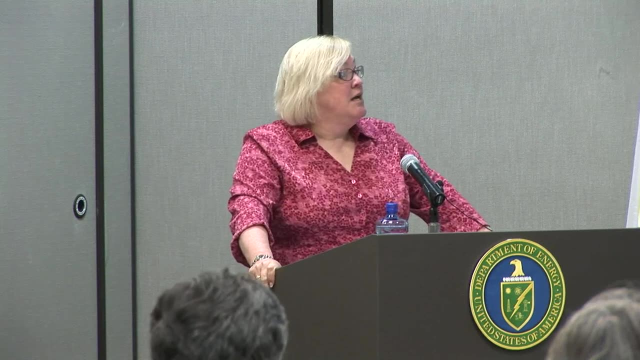 really directly tied to the UN but has some special links to it- And you'll see that at the very end of the policy piece of the talk. in terms of its relationship with the Security Council, It has its own 140 member states, separate from the UN. 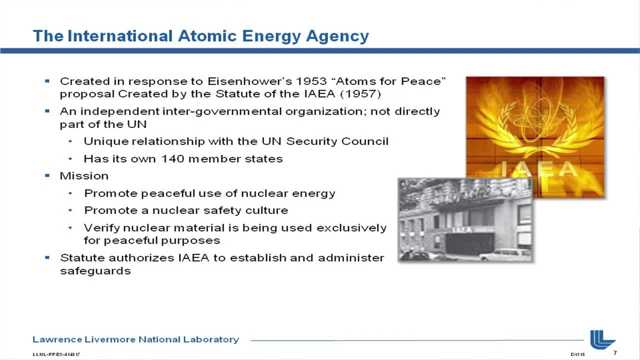 It's much more than just a single member state. It's a multi-state organization And it's very similar to the UN. Its mission is to promote the peaceful use of nuclear energy, to promote nuclear safety culture and to verify nuclear material that is being exclusively used for peaceful purposes. 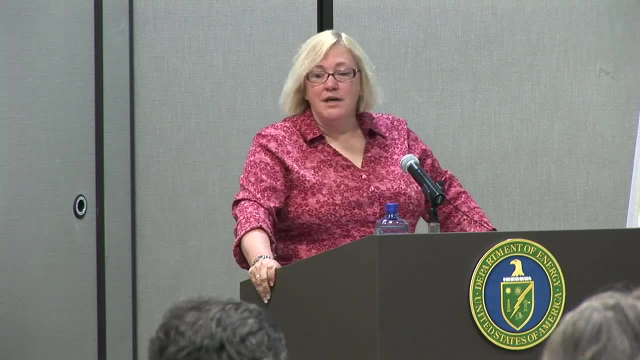 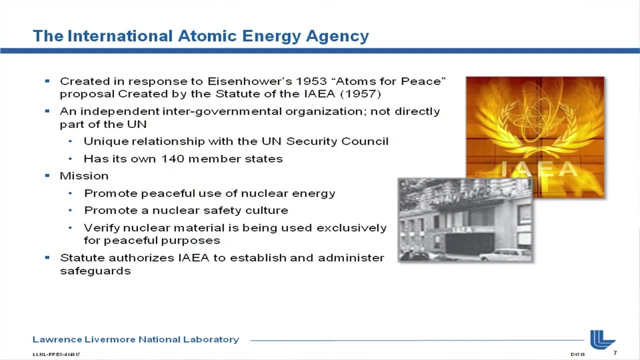 Statute authorizes the IAEA to establish and administer safeguards, the concept that President Eisenhower had laid out. You can see here in this pretty fuzzy picture this was the original IAEA headquarters in Vienna. They have a much more substantial organization and complex there now, but they still remain. 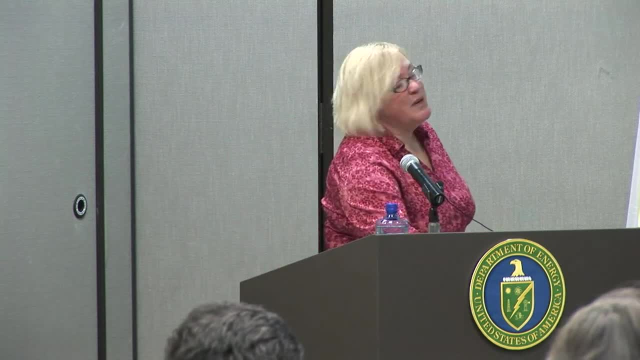 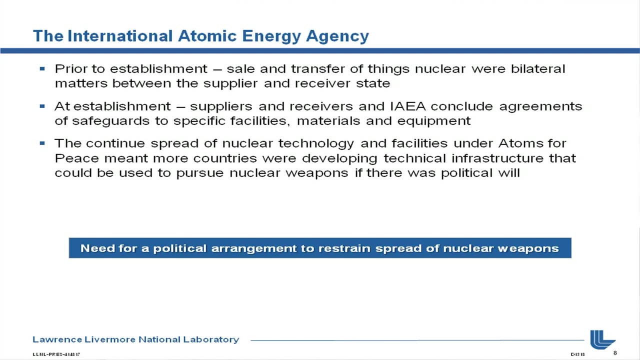 in Vienna. So let's spend a minute looking at what the impact of the formation of the IAEA had on things nuclear. Before the stand-up of the IAEA, the sale and transfer of things nuclear were a bilateral agreement between supplier and receiver. 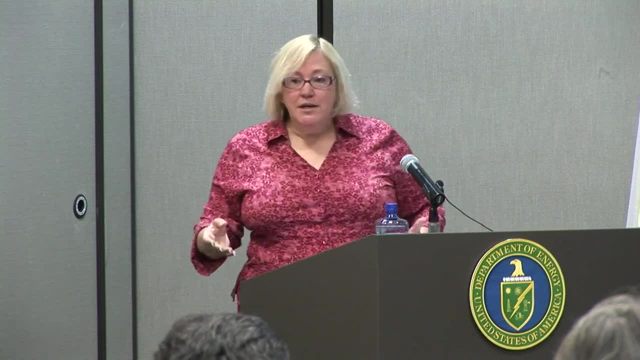 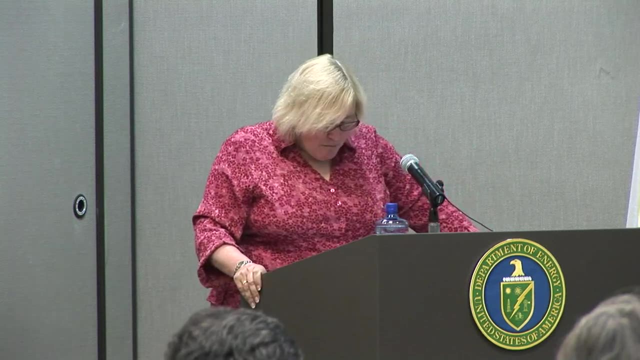 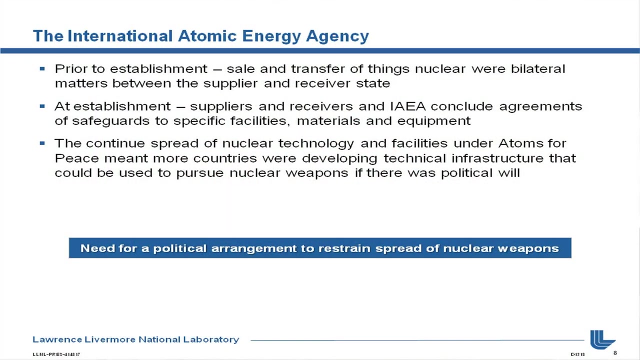 Country A wants to sell fissionable material to country B, They make their agreement, the materials transferred, compensations received and that's all that had to happen. Upon the establishment of the agency that now became a trilateral agreement, The IAEA necessarily had to be involved in those agreements and the transfer of equipment. 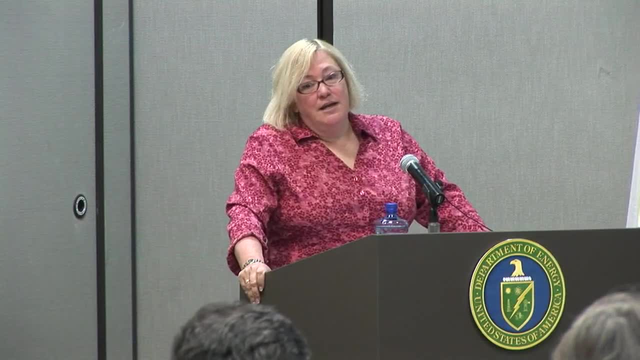 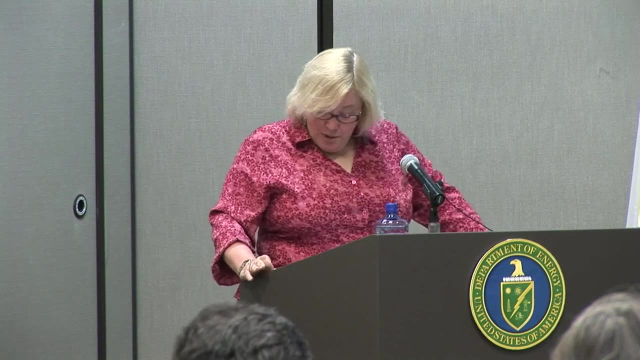 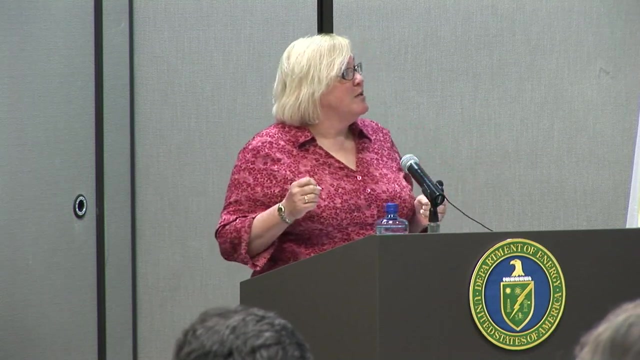 and materials. Although the establishment of the IAEA did not oblige either the supplier state or the receiver state, They had to comply with safeguards. So while the IAEA was there, there was no teeth in the sale and transfer of nuclear materials and nuclear equipment. 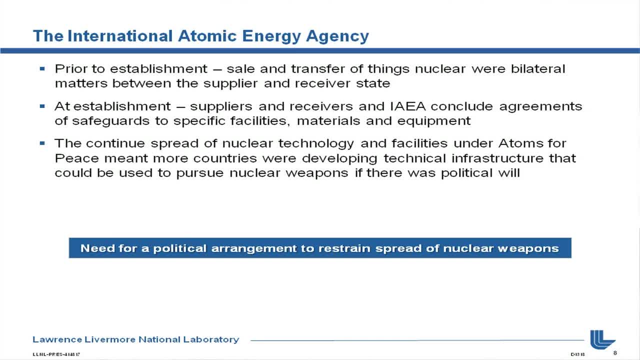 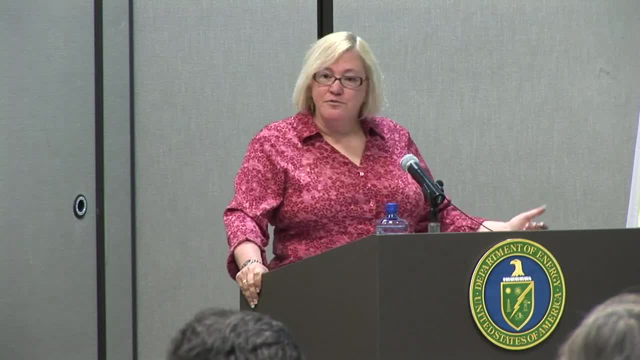 So that was going on at the same time of the Atoms for Peace movement, in which the US participated quite heavily in supplying research reactors and research fuel to any number of countries in the world. So while more things nuclear were being moved around the world, 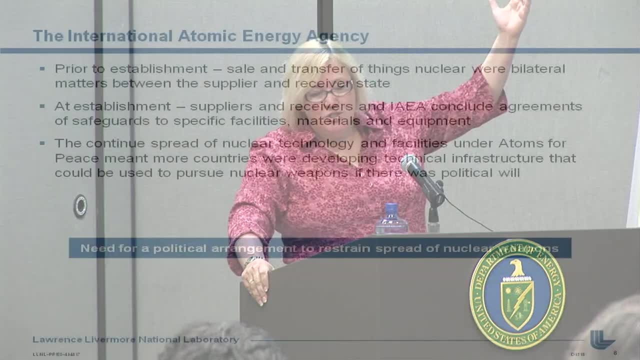 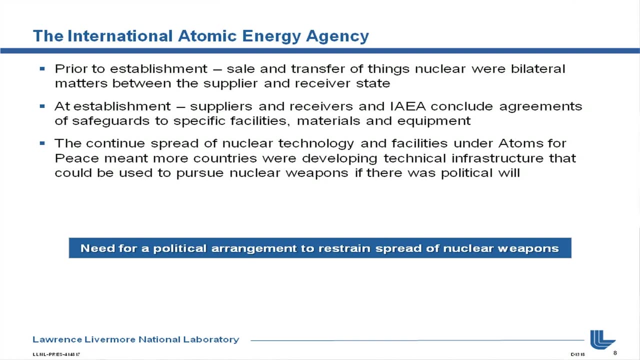 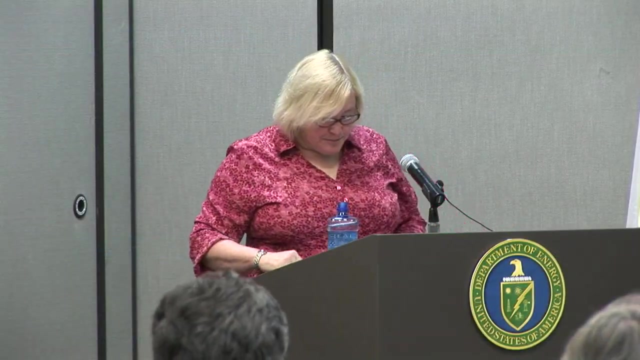 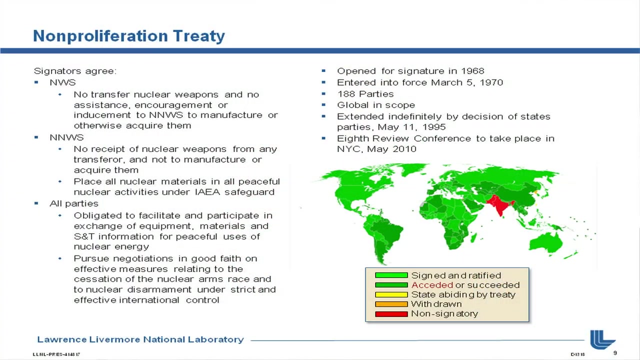 We had a sort of a partial implement, a partial fix on nuclear safeguards. So at this point in time it was realized that there was a need for some further political arrangement to restrain the spread of nuclear weapons. Hence the advent of the Non-Proliferation Treaty, which turned out to be the teeth of 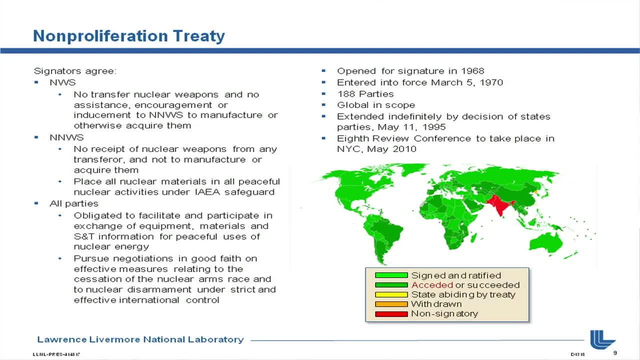 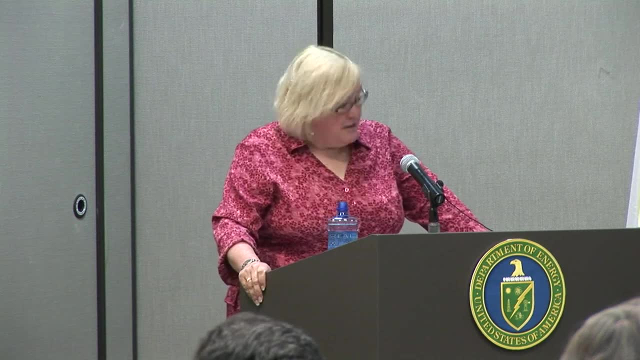 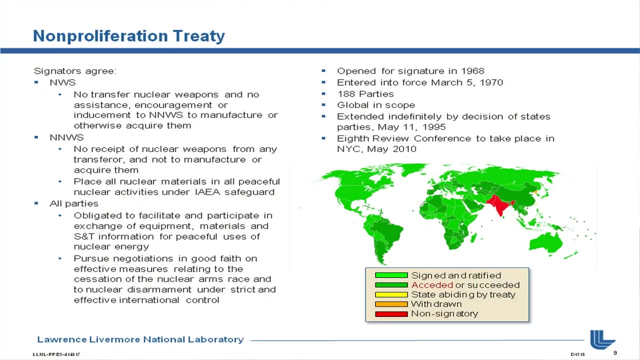 implementing safeguards throughout. The treaty was opened for signature in 1968 and entered into force in 1970. There are now 188 parties to that treaty, which is completely global in nature. In 1995, the member's signature states expanded that treaty indefinitely into time. 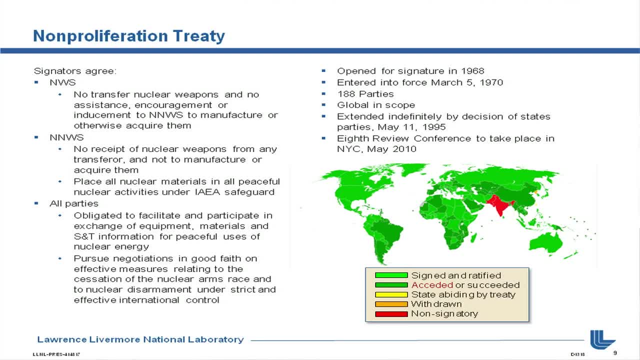 It's a little hard to see, so let's go over this. This is the map of the world. All the countries that are green are either signatures or have ratified, acceded or succeeded to the Nuclear Non-Proliferation Treaty. 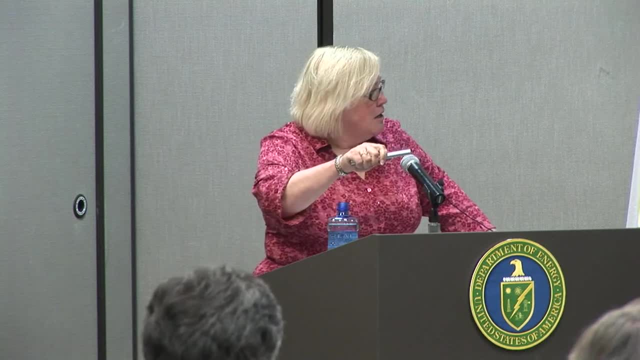 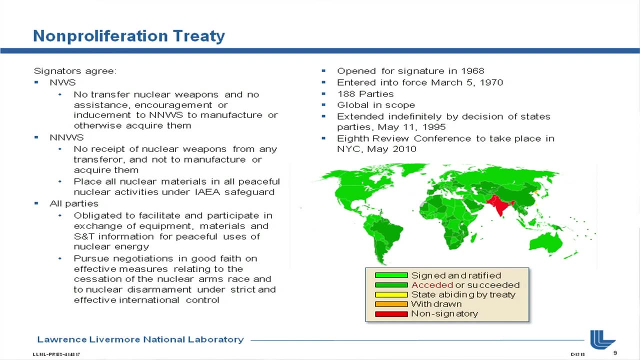 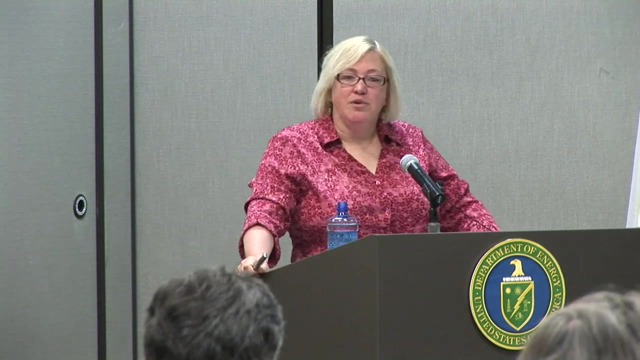 You can see, it's a fair fraction of the world. There's a yellow country, and that happens to be Taiwan, who voluntarily abides by the regulations and the implications of the Non-Proliferation Treaty without having signed it. The orange is North Korea, who originally signed the Non-Proliferation Treaty, but then 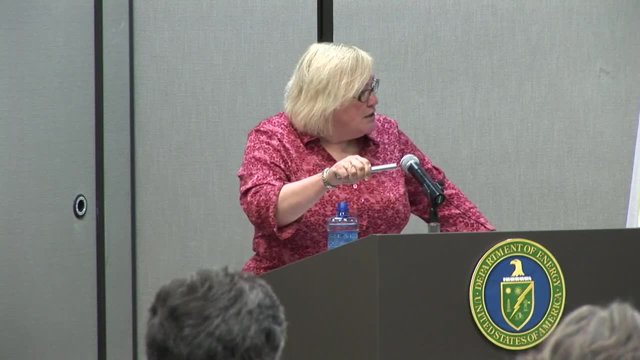 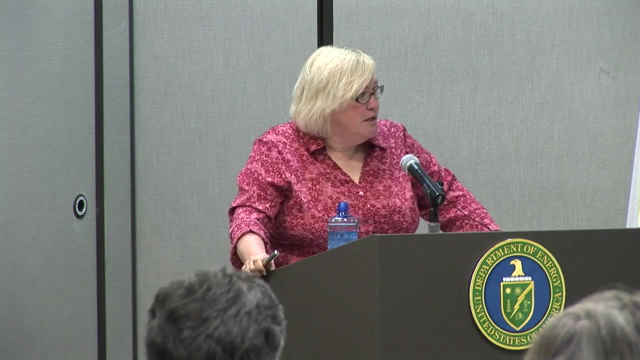 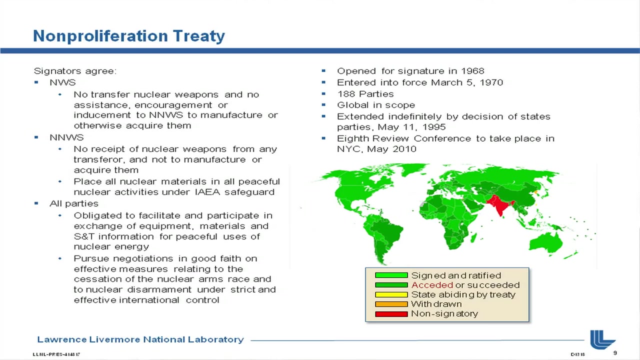 withdrew. Importantly, here are the red countries, and those are non-participants, non-signatories, of the Non-Proliferation Treaty. They're India, Israel and Pakistan. so they are free to buy and sell nuclear materials, particularly amongst themselves, but with no conditions at all. 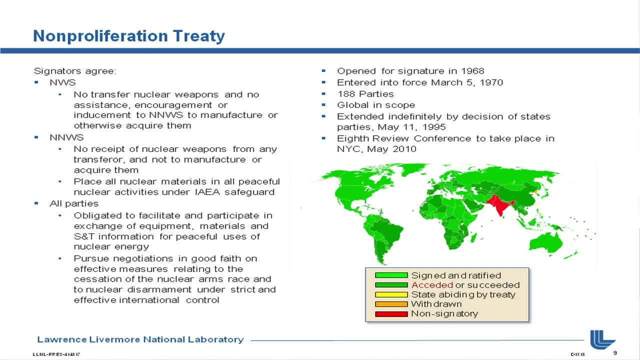 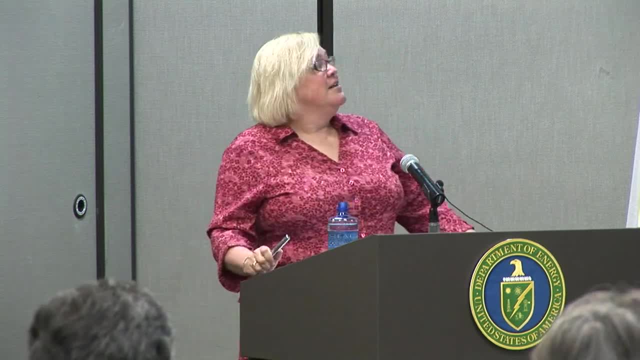 As an example. the Cold War area was able to longer back then and the world ended up in a cooperative contention of the treaty. The treaty set up what some people refer to as the haves and the have-nots. the haves: 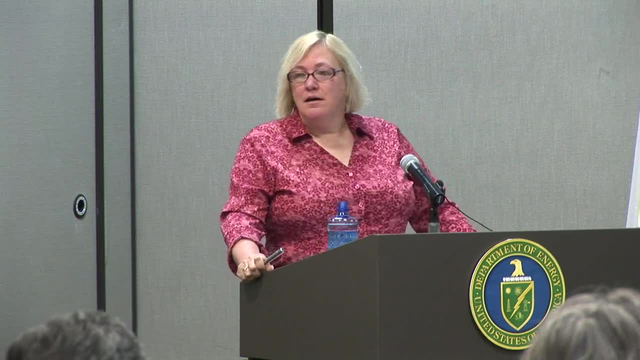 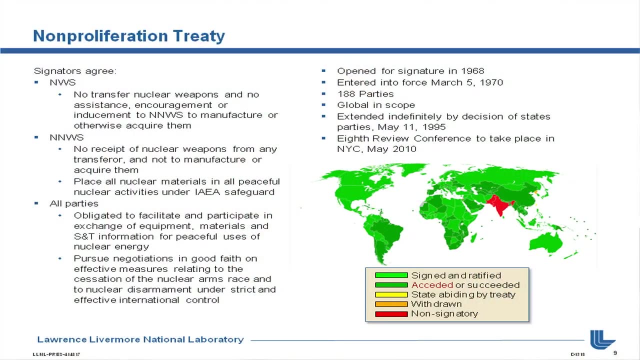 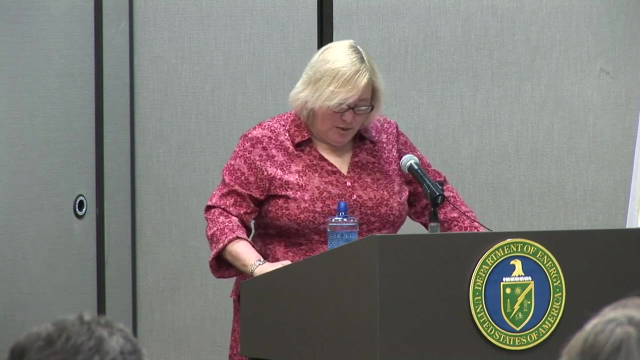 being the nuclear weapon states, the NWS, of which obviously the US is one, and those countries agreed that there would be no transfer of weapons, nor assistance or encouragement or inducement to non-nuclear weapon states to manufacture weapons or to try to acquire them. Non-nuclear weapon. 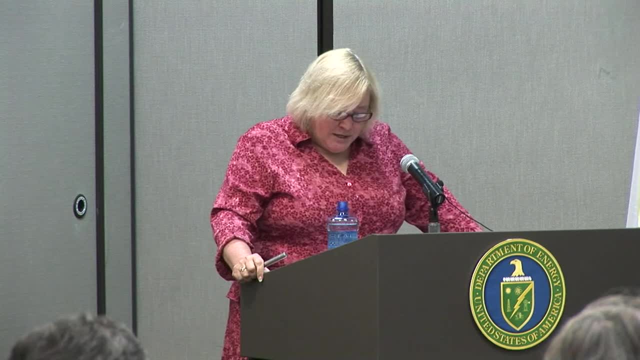 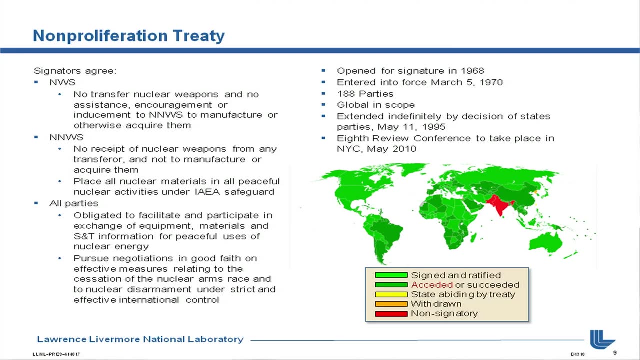 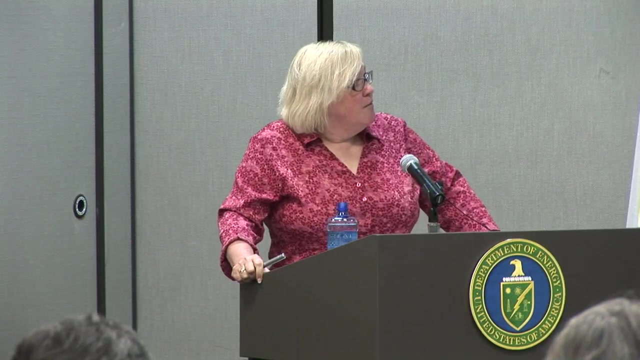 states received not to receive nuclear weapons from a country, nor to try to transfer them, nor to try to manufacture them or to try to acquire them, And they agreed to put all their nuclear materials, which was by definition for peaceful uses, under IAEA safeguards. 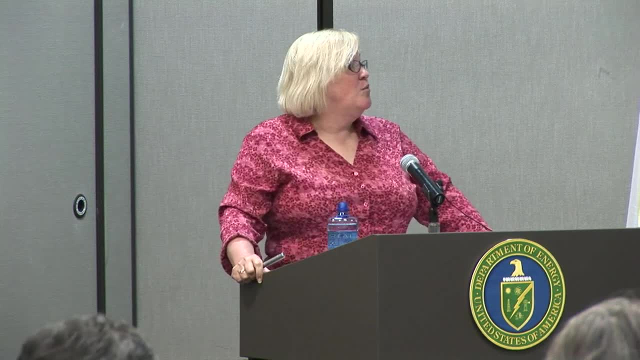 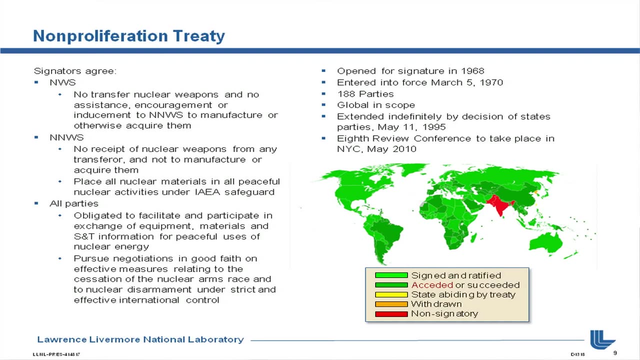 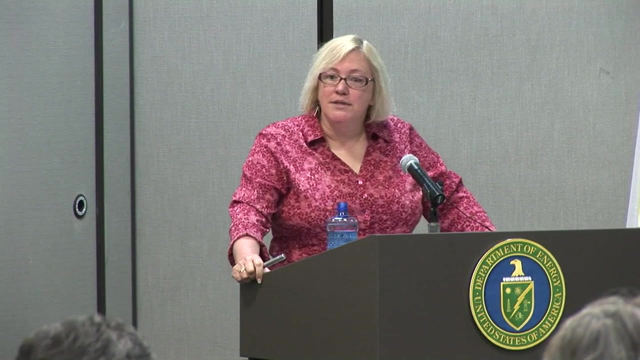 All parties- the nuclear weapon states and the non-weapon states- were obligated to facilitate and participate in the exchange of equipment and materials and S&T information for the peaceful uses of nuclear energy. That's considered an inalienable right of the parties signing the treaty that you. 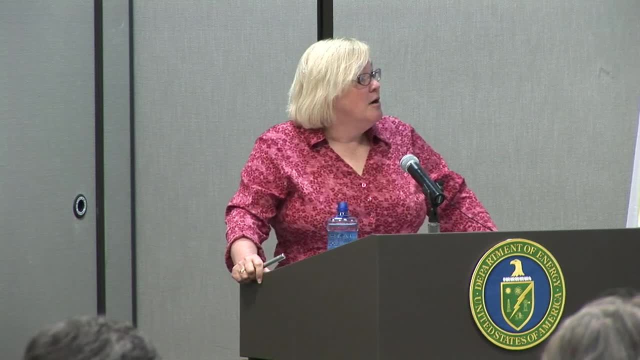 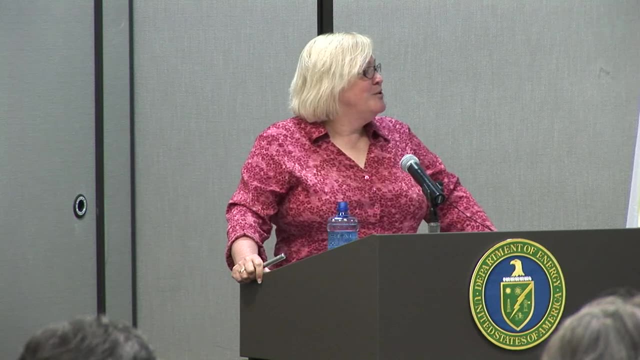 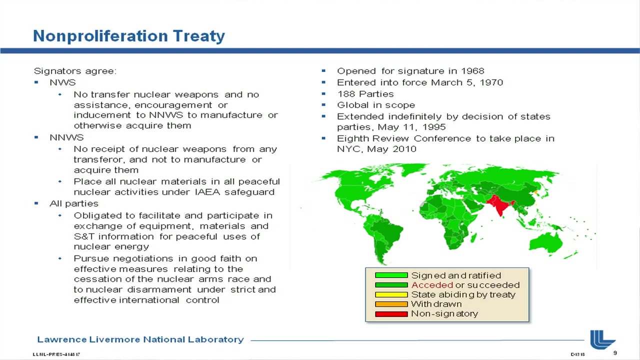 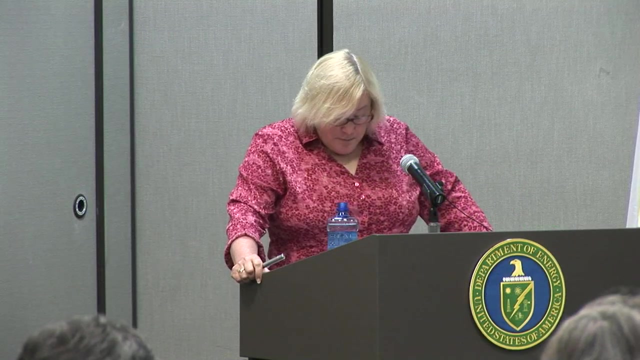 may pursue and share information related to the peaceful use of nuclear energy. And all parties again agreed to pursue negotiations- And there were negotiations in good faith- on the effective measures related to the cessation of the nuclear arms race and to pursue nuclear disarmament. A further requirement was that the non-nuclear 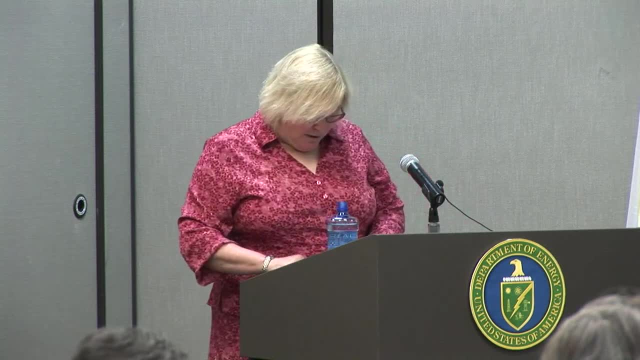 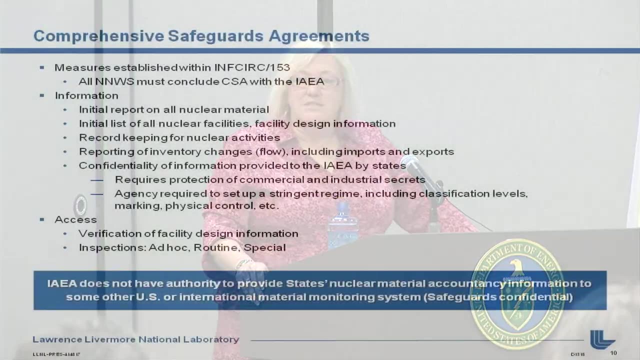 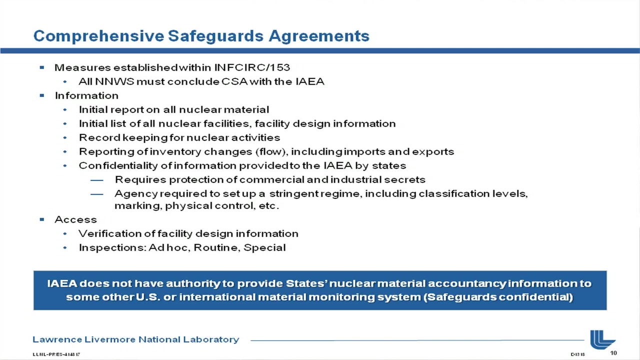 weapon states would comply and provide what's called comprehensive safeguards agreements. Consider comprehensive safeguards agreements to be your implementing strategy for the non-proliferation treaty. The country that signed filed a comprehensive safeguards agreement to say how they were going to implement safeguards in their country. 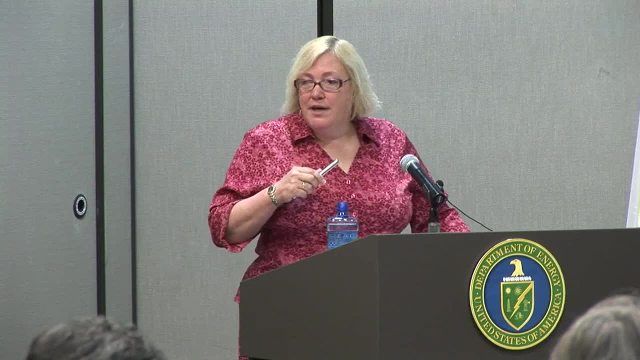 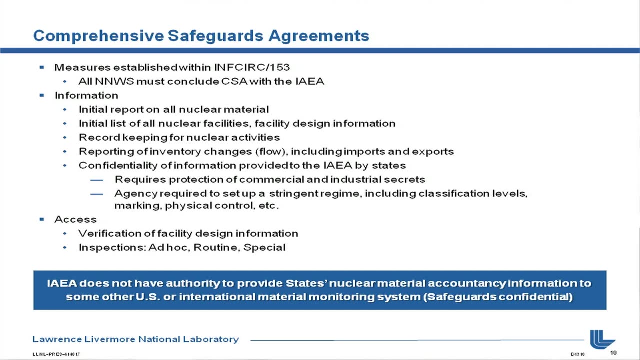 The states agreed to provide information- and how they will do that is detailed in this document- about their initial report of what they have for nuclear material in their country, an initial list of facilities and facility design information. We'll see in a few minutes why the design information is important. They would provide information on how they 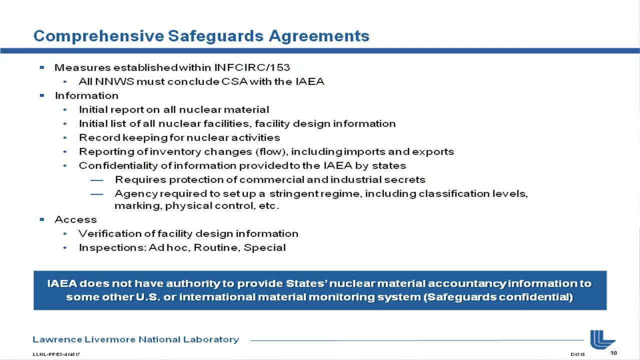 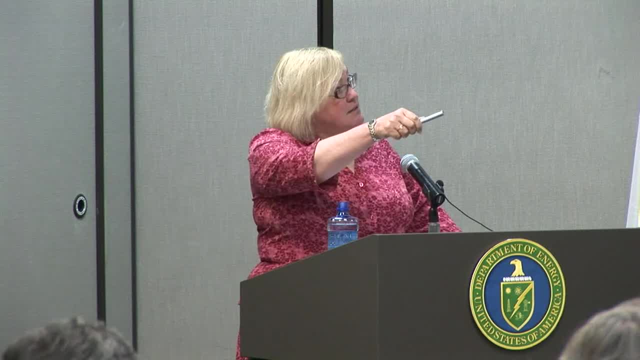 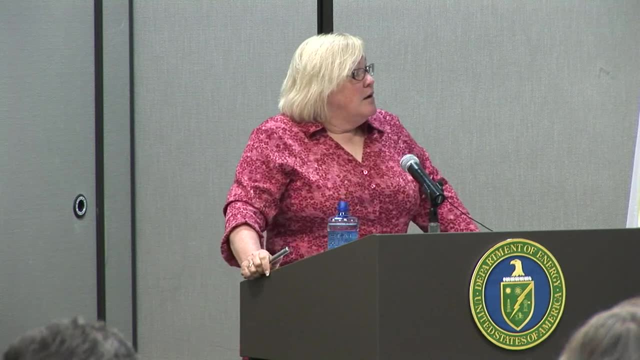 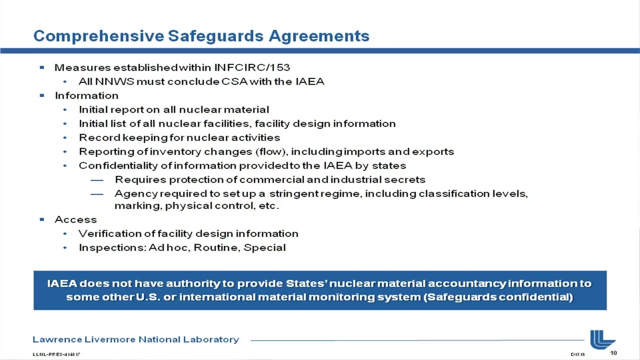 keep their records related to their peaceful nuclear research and they would show their reporting of inventory changes, that is, flow within their country as well as exports flow into their country and flow out of their country. The IAEA provides confidentiality of all that information that's provided to them by individual. 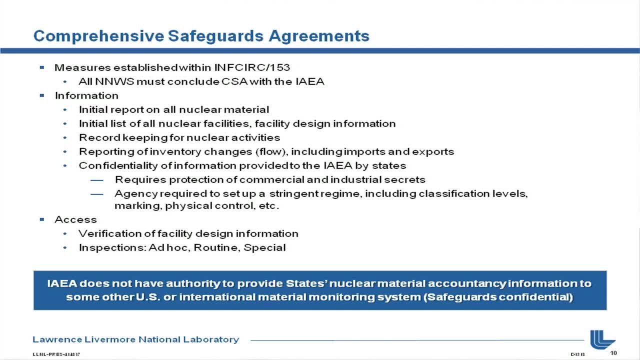 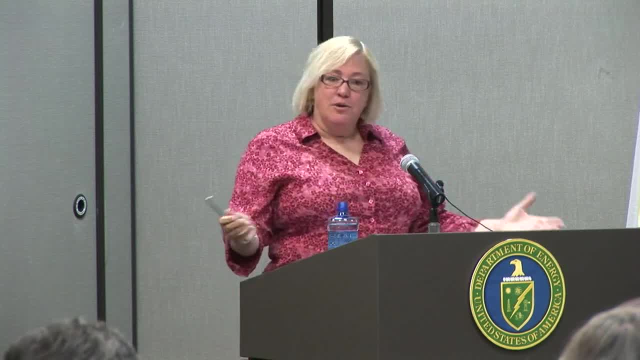 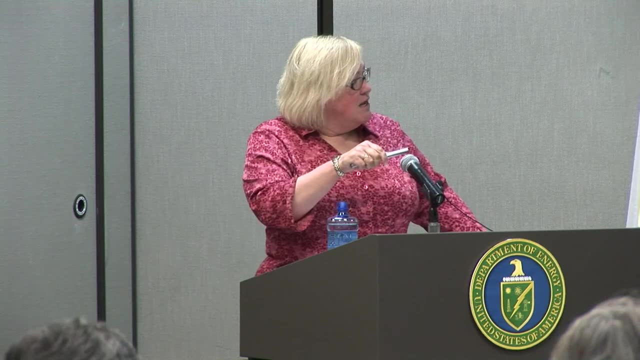 – by the individual states and they are required – the IAEA is required to – to protect commercial and industrial secrets. So you're working on your peaceful nuclear power, but some of it has commercial value. That information is not to be made available to any other state. 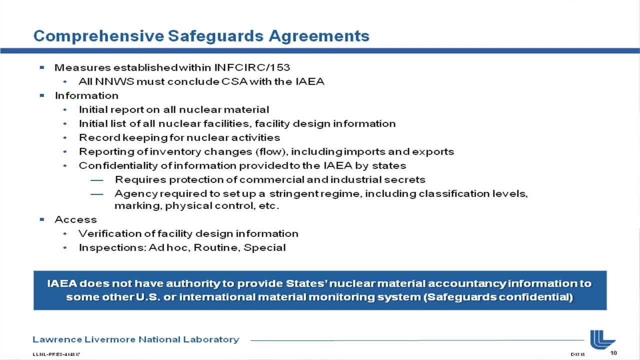 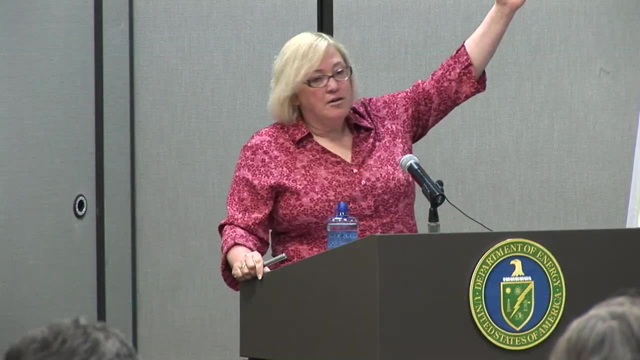 to the US or any other kind of international organization. That material is protected by a category of classification called Safeguard Confidential. The IAEA then is granted access to your facilities, to your information, to verify all of that information in your report. 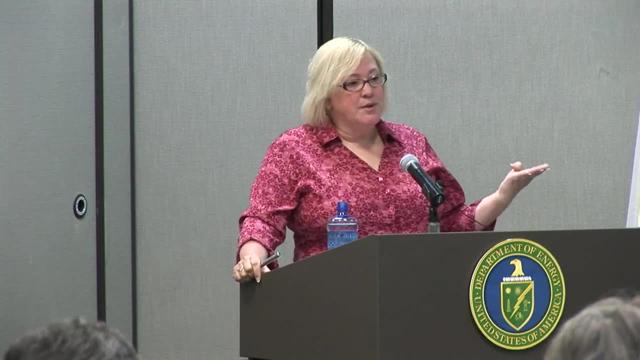 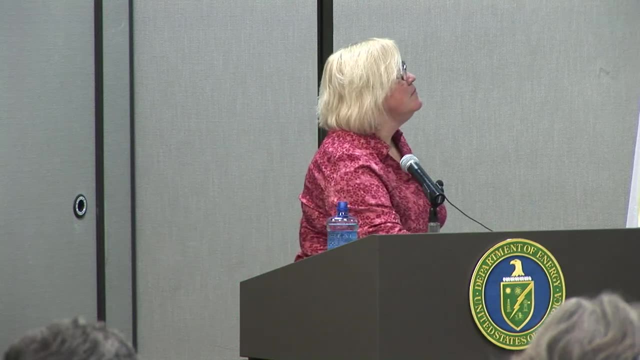 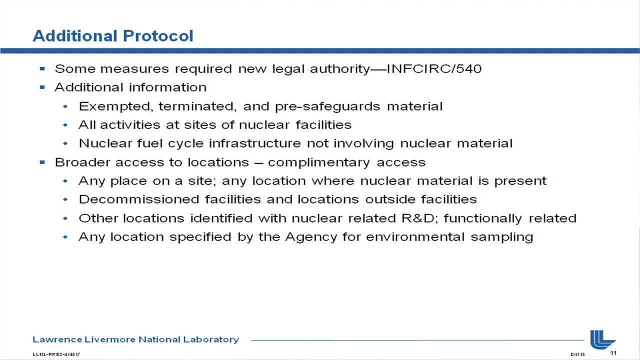 and it defines an inspection regime with three levels of inspection: ad hoc, routine and special. Over time it became clear that you could pursue quite a bit of nuclear-related R&D or upstream R&D. whether that's nuclear-related R&D or upstream R&D. 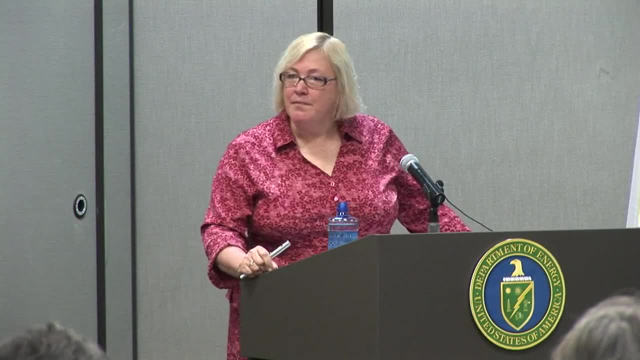 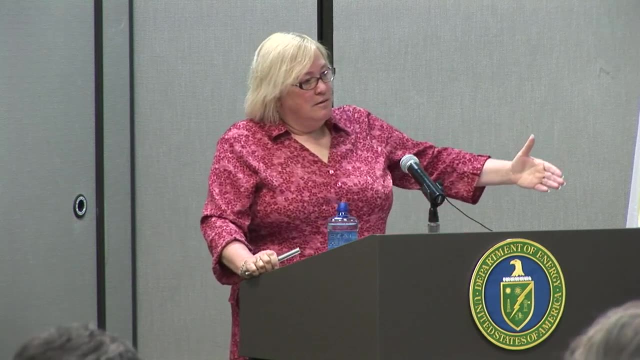 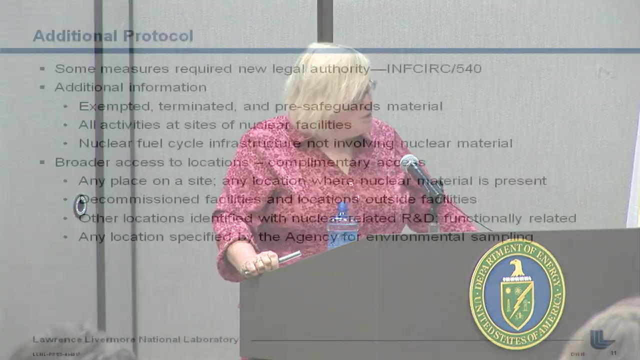 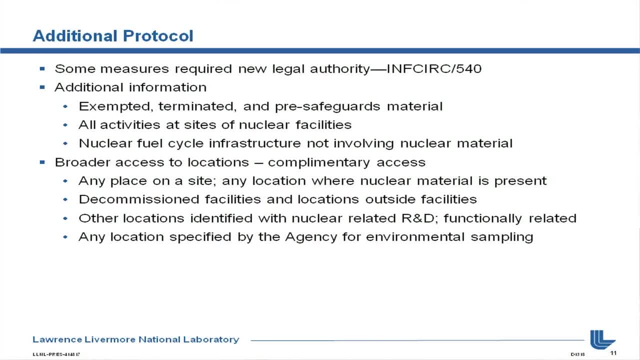 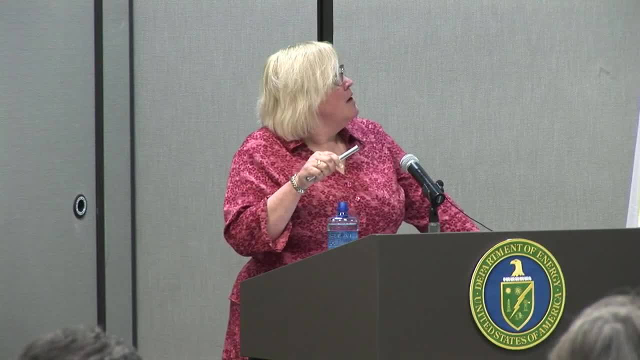 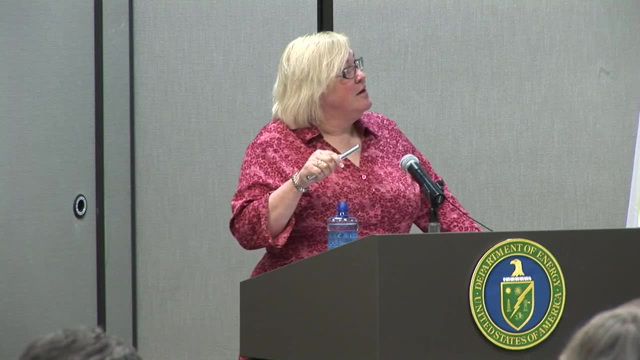 It grants the IAEA broader access on sites and a broader access to information about what's going on in those sites. So we've now added to the information that states report to the IAEA information about exempted, terminated or pre-safeguarded material. 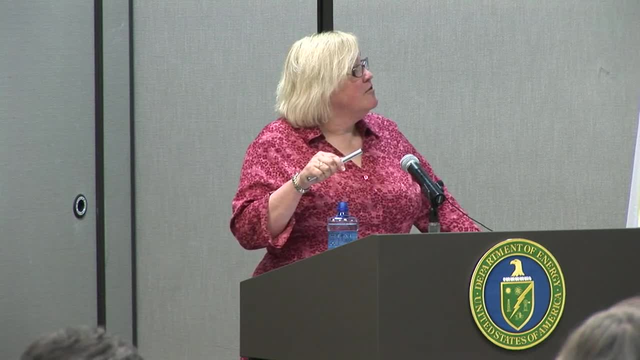 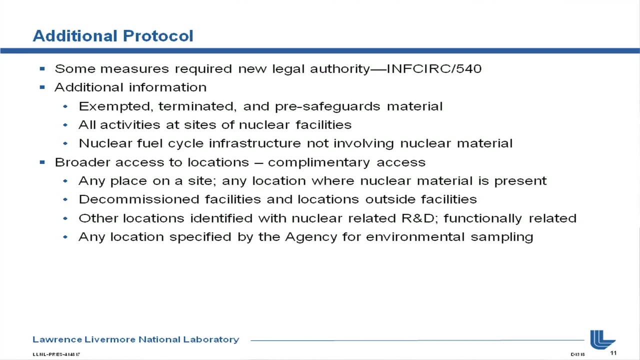 all activities at the sites of nuclear facilities and nuclear fuel cycle infrastructure that doesn't involve nuclear material. The IAEA is granted broader access to locations. It's referred to as complementary access to any place on a site and any location where nuclear material is present. 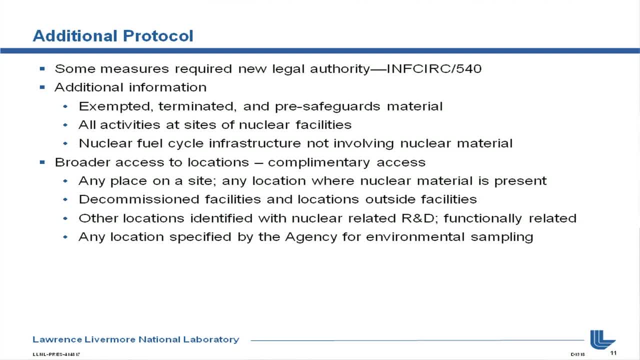 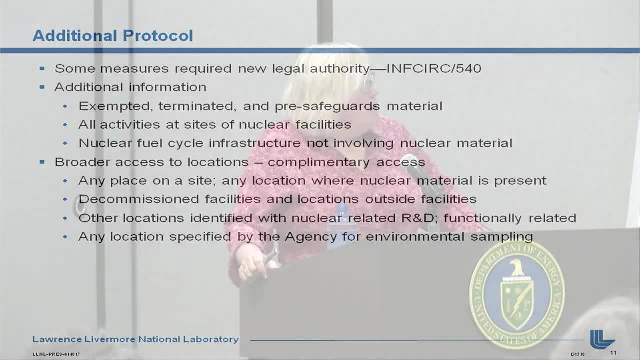 to decommissioned facilities and locations, as well as to other sites. It's referred to as complementary access to any site outside of facilities and any other locations with identified nuclear-related R&D. The United States, as a nuclear weapons state, is not required to have a complementary safeguards agreement. 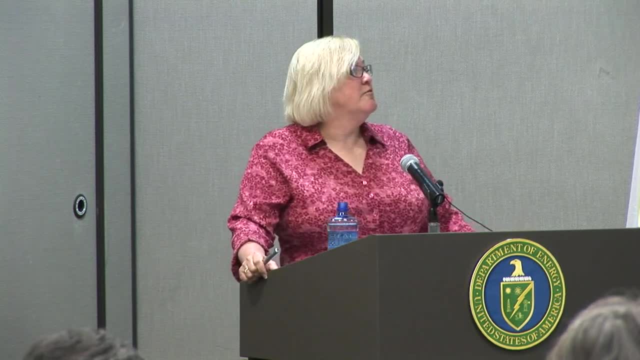 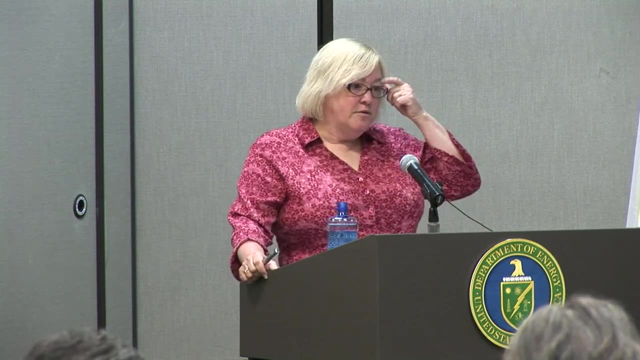 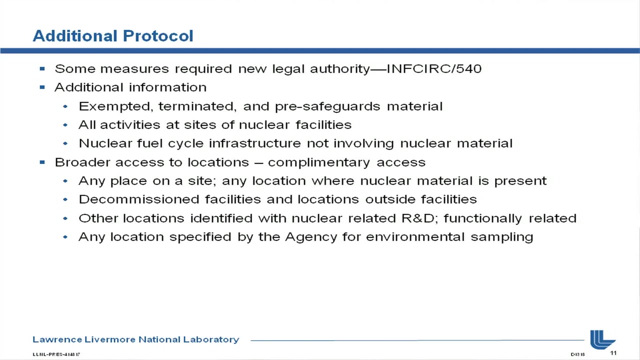 nor is it required to have additional protocol. That's a requirement only for the non-weapons states. The United States has agreed to voluntarily comply with the complementary safeguards agreement as an additional protocol. The additional protocol was, just as I said, signed and the articles of enforcement. 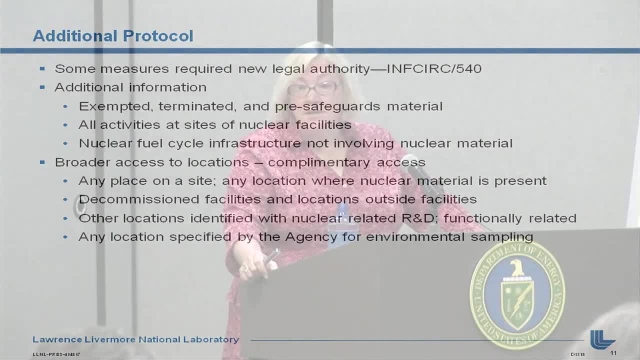 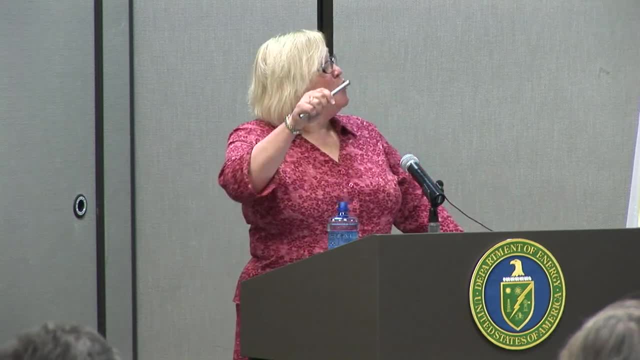 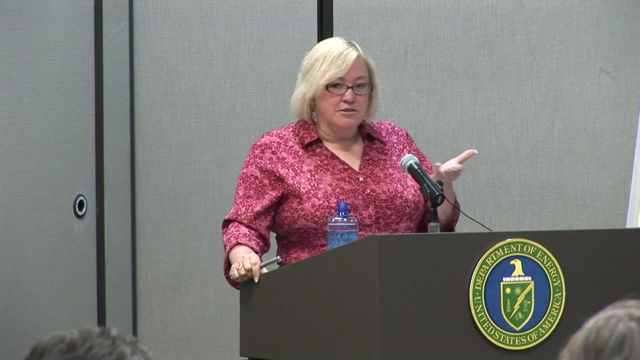 were deposited in Vienna and it went into force for the United States in January of 2009.. That means annually. the United States voluntarily reports on all of this information to the IAEA. Many of you may be involved with this at your various sites. 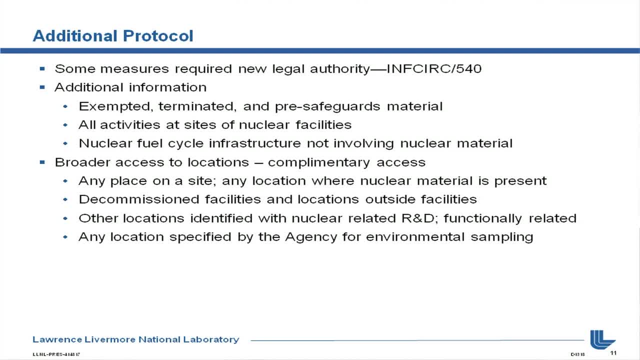 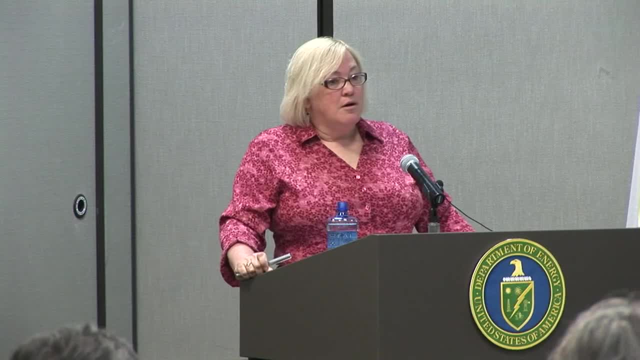 For example, when we filed it at Lawrence Livermore, it involved some of our laboratory-directed R&D. it would involve some different- you know lots of kinds of preliminary or studies you might do on the modeling like David DiPaolo talked about. 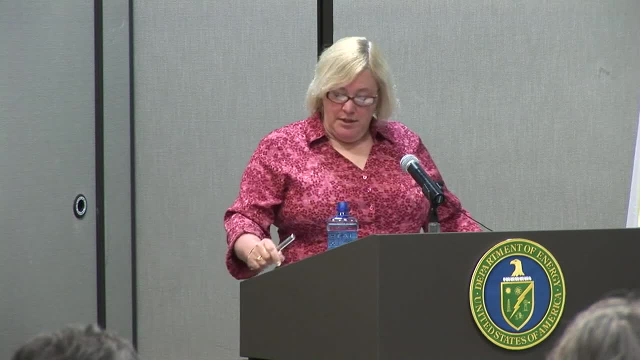 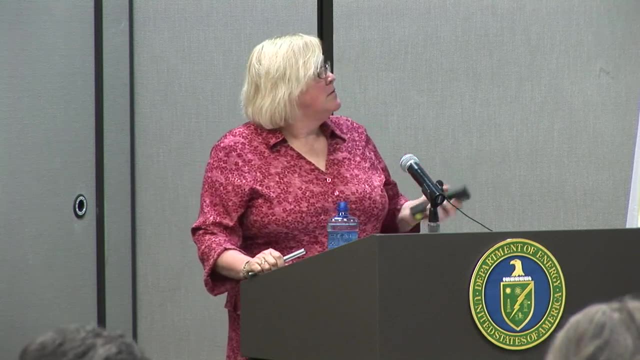 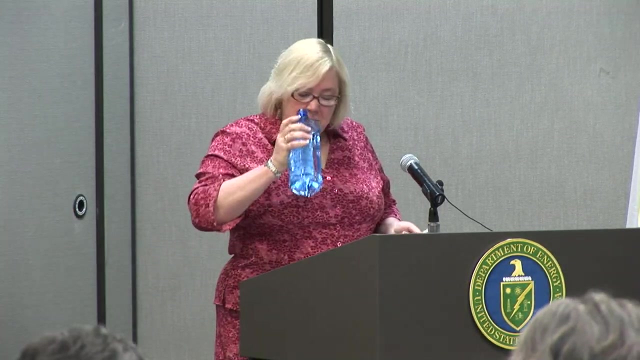 that don't involve nuclear materials directly but are related to pieces of nuclear energy. I think the additional protocol really came about because of the RAC when we first filed for it, whether there was a deal in it. They had things that really did fall in at the 3 to 6 agreement. 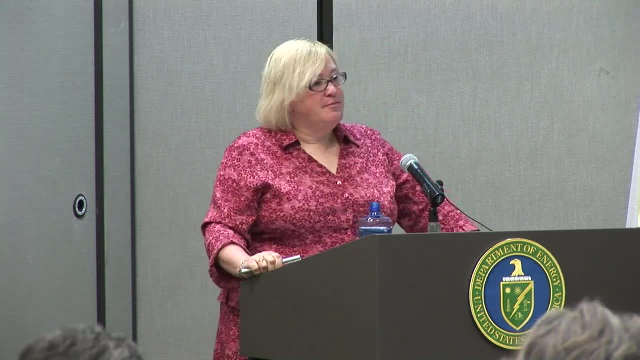 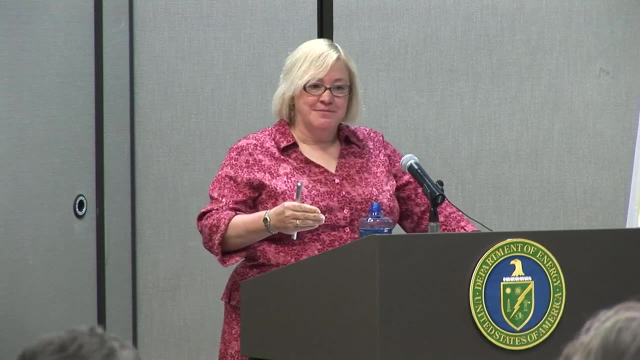 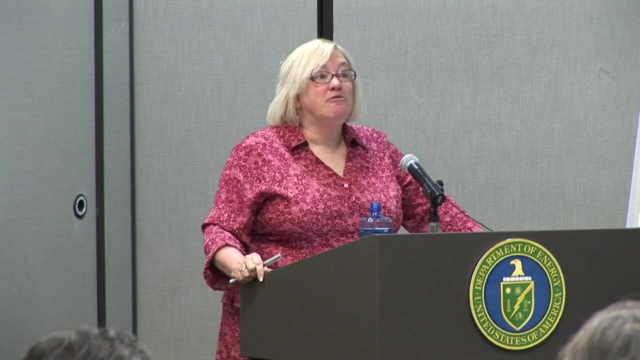 so it had to be expanded. So I think it gets expanded and I think the US signs up for it voluntarily, because it does alter your ability, your negotiating stance. I mean, we are providing information voluntarily as a good-faith measure. 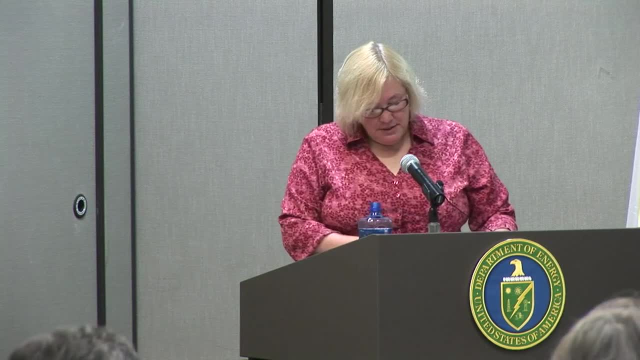 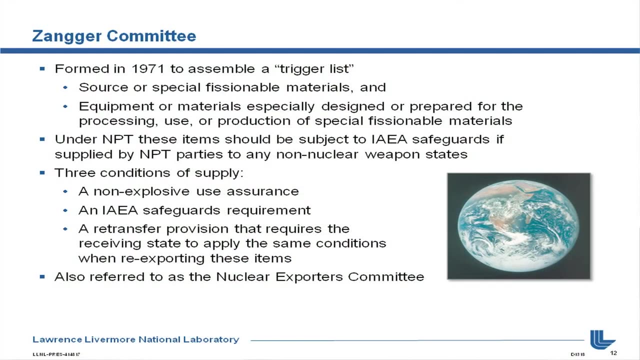 So we've talked about material. Let's talk a moment about equipment that's specific to the IAEA. We've heard several talks about processes. You've seen some of the equipment. You've seen pictures of it. The Zanger Committee was formed in 1971. 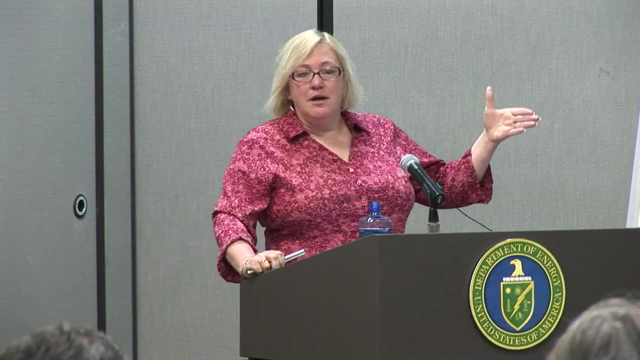 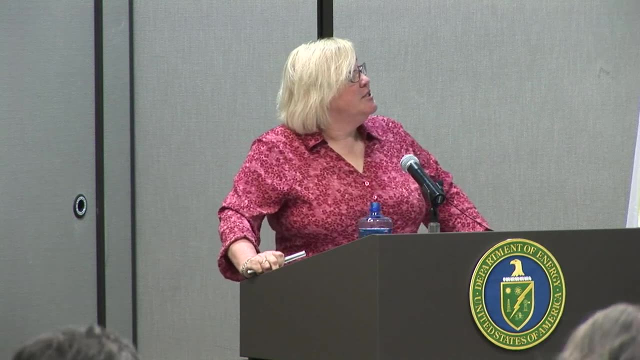 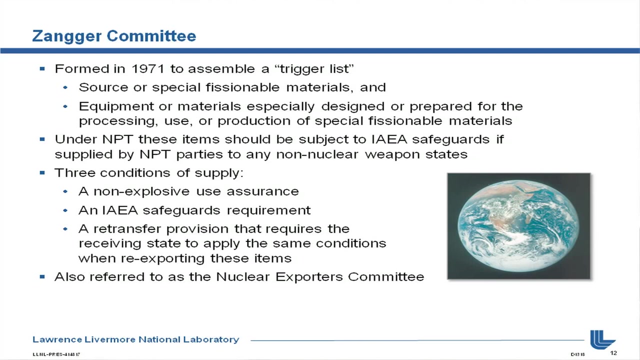 to assemble a list, called the Trigger List, of equipment that would trigger safeguards, documentation and validation under the Non-Proliferation Treaty. So that's sources or special fissionable material and equipment or materials especially designed and prepared for processing use. 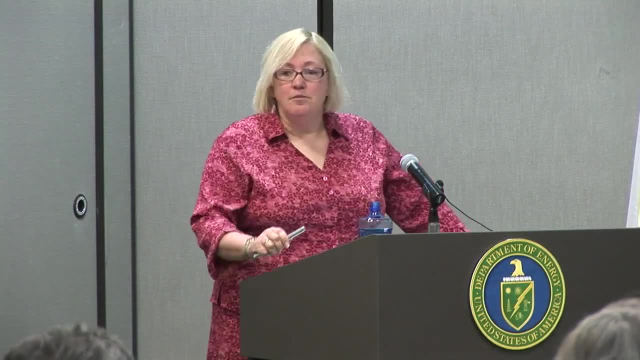 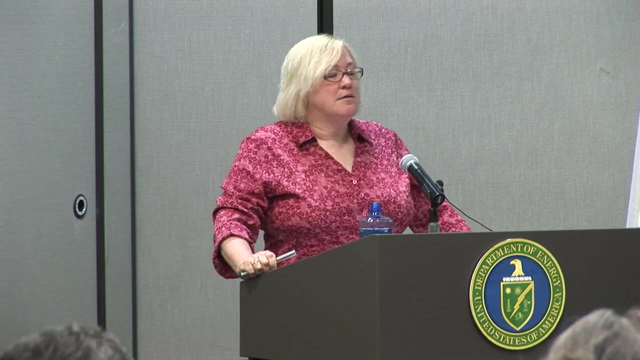 or production of special fissionable materials. What's the most important words in that sentence? Are especially designed or prepared for, and we'll see in a minute why. that's the important part of that sentence. Under the treaty, these items were agreed to be subjected. 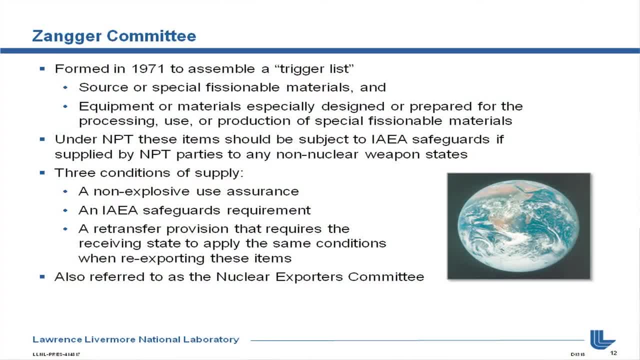 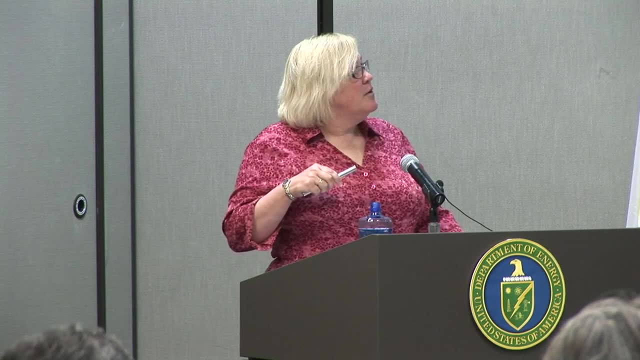 to safeguards if they were supplied by other treaty parties to non-nuclear weapons. So this refers to the transfer of equipment from one state to another. Three conditions have to are sufficient for that transfer. There has to be a non-explosive use assurance. by the receiving country. The IAEA safeguards must apply to both the sender and the receiver, and the re-transfer provision requires that the receiving state, if it turns around and sells it to a third party, transfers the safeguards requirement to that country. 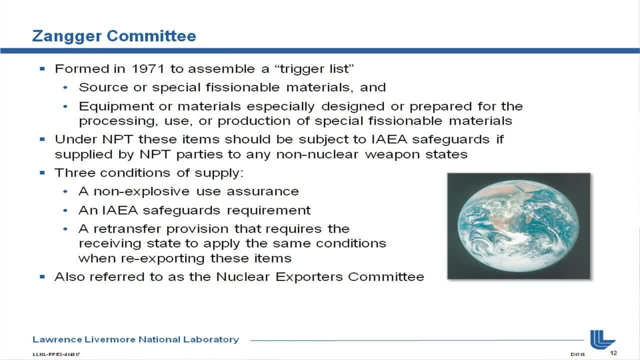 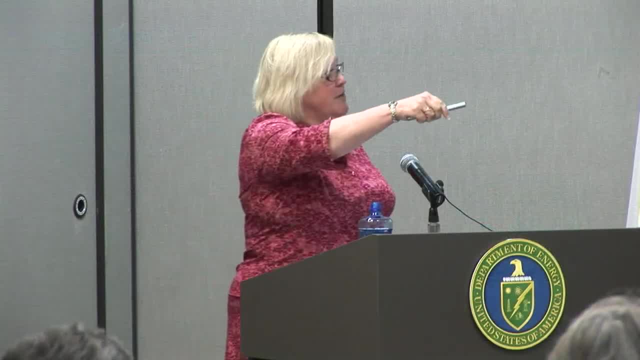 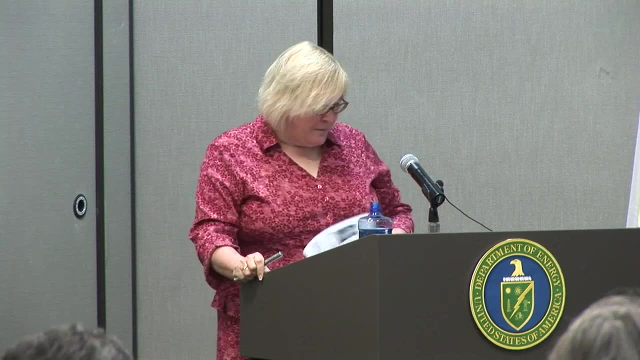 So this was specifically aimed at people being middleman transfers from a non, from a weapon state to a, even to a non-signature, by limiting, by having that requirement on the transfer of the safeguarding equipment. Similar is a group called the Nuclear Suppliers Group. which was found in 1974.. This now refers to listed items that could only be exported to non-nuclear states if certain safeguards were agreed to or if there were exceptional safety circumstances. So the there had been the observation. sorry, this was driven by an observation. 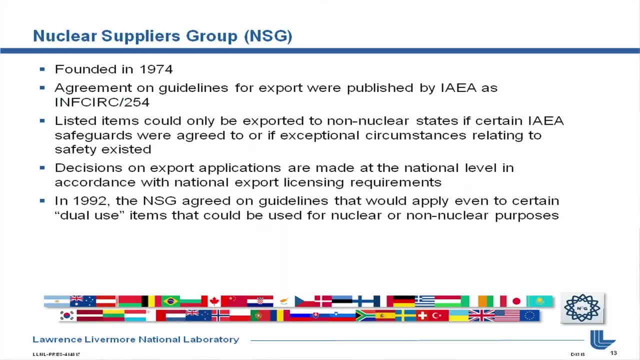 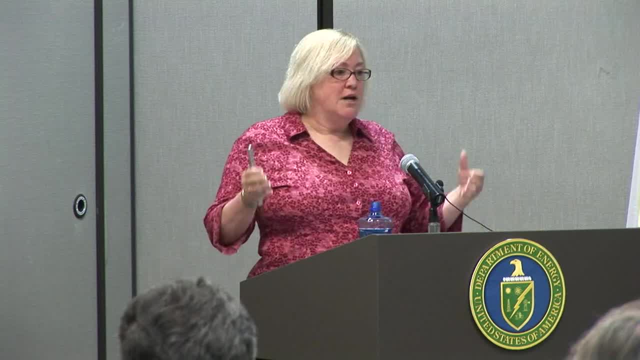 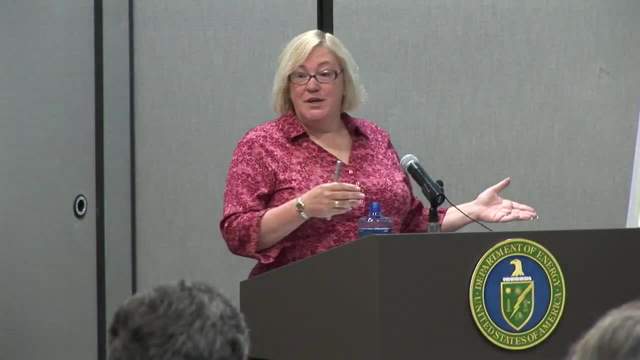 that non-weapons specific nuclear technology could be readily used for weapons development. Let me say that again. So this, So we now refer to this as dual-use equipment. There's equipment that you could use in peaceful uses of nuclear energy that could easily be adapted, or not even really adapted. 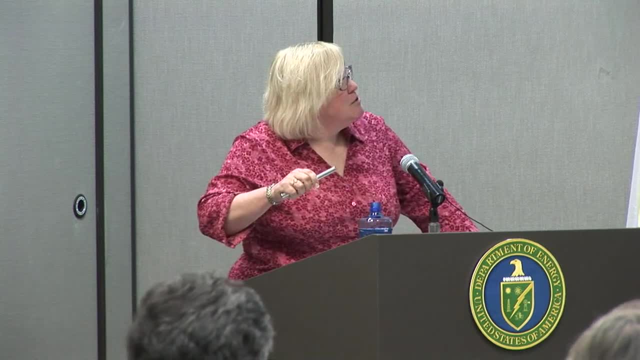 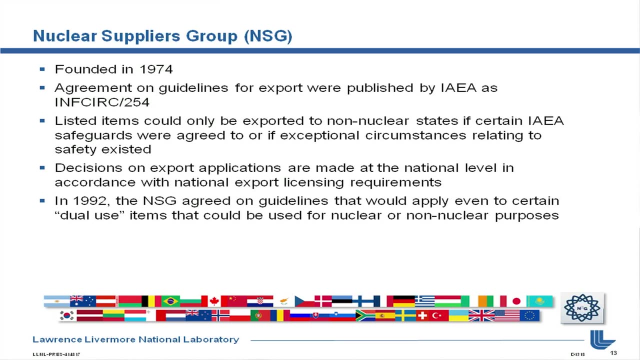 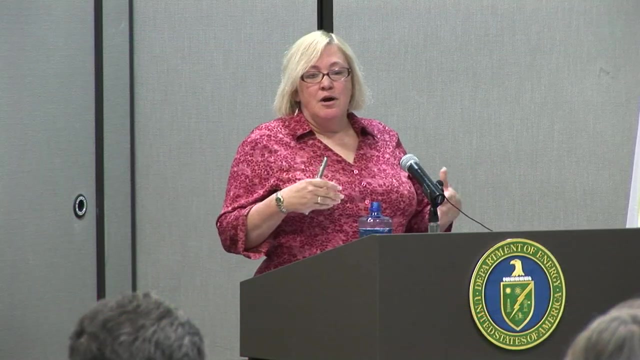 just directly used for weapons production. Those pieces of equipment were felt need to be tracked as well. It talks about listed items only being able to do subject to certain transfers, And then what it says is that each country itself will make and enforce the exporting of those pieces of equipment to another country. under their own internal laws. If you would like to entertain yourself sometime, you might want to consider why it's necessary to have two groups and what is the difference between those two. I will give you a hint. It would be poke around That when France signed the Non-Proliferation Treaty, which was in 1992,, 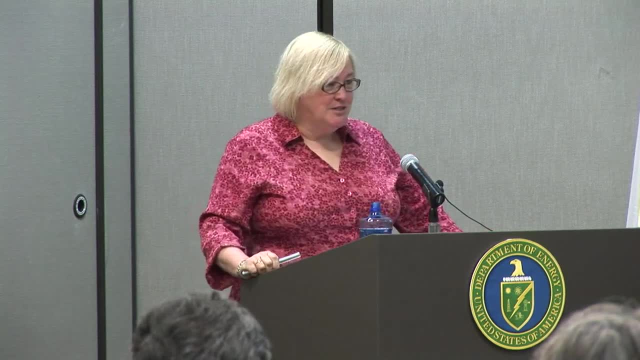 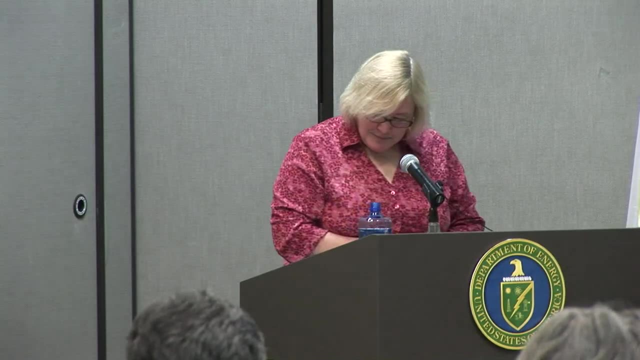 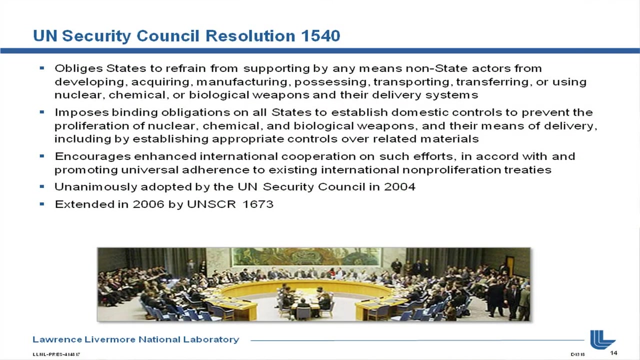 so prior to 1992, they were not subject to any of the regulations of the Non-Proliferation Treaty- Makes for some interesting reading. In response to 9-11, the UN Security Council passed Resolution 1540.. And the basic concepts that get introduced during this process. 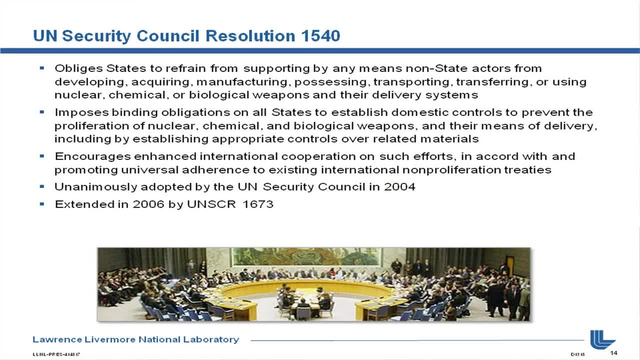 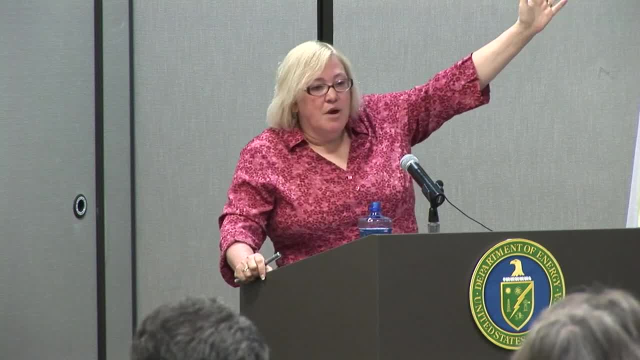 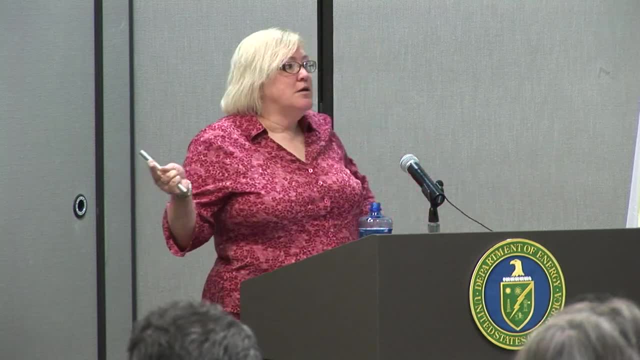 are. we now start to see the language relating to non-proliferation, non-state actors, that is, subnational groups or terrorist cells, coming under some type of regulation and some type of observation, And we start to see the introduction of a broader suite of weapons. 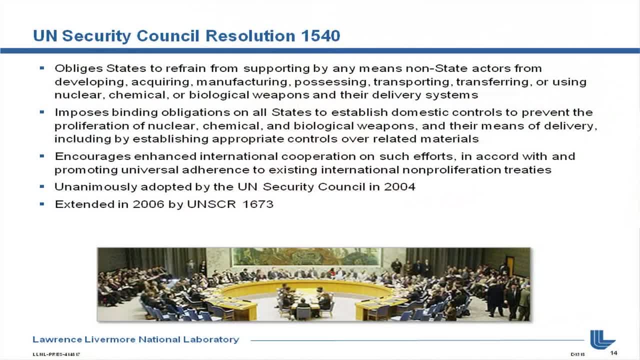 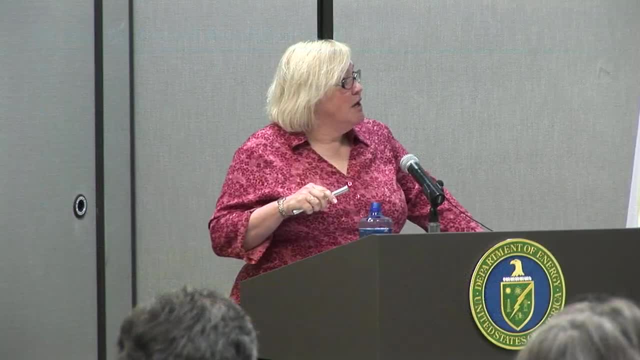 of mass destruction beyond nuclear weapons. So this particular resolution obliges states from refraining to support non-state actors in anything related to all forms of nuclear, chemical and biological weapons. This was unanimously adopted by the UN Security Council in 2004,. 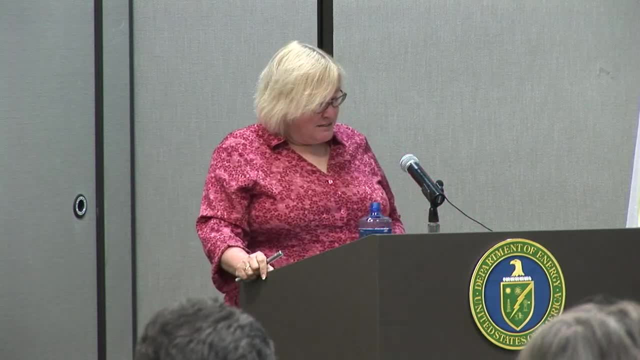 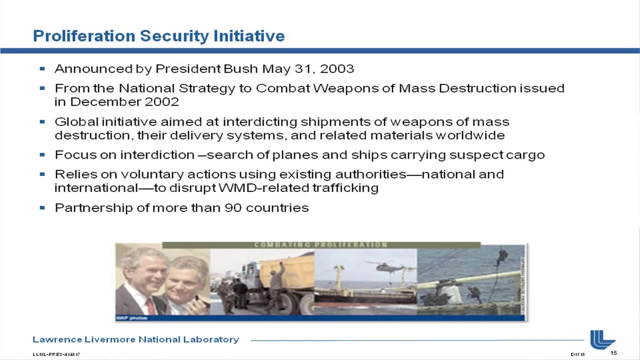 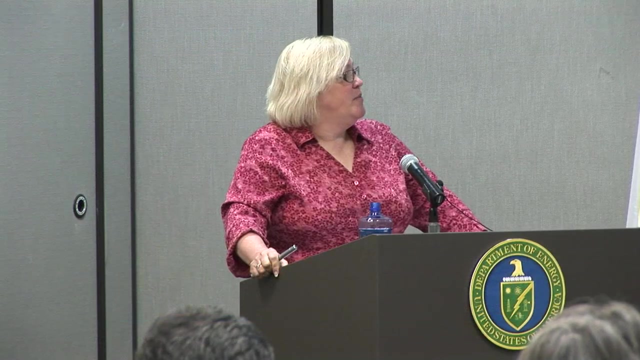 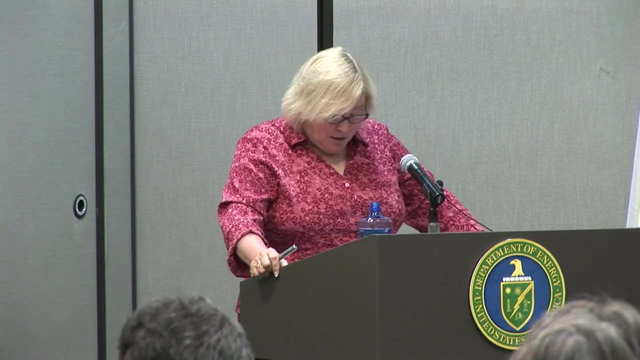 and extended in 2006.. In support of 1540, President Bush announced in 2003,, based on the National's strategy to combat weapons of mass destruction, the proliferation security plan, Security Initiative. This is a global initiative implemented by a series of bilateral agreements. 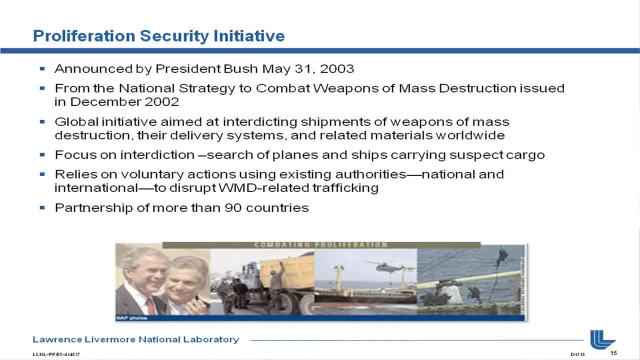 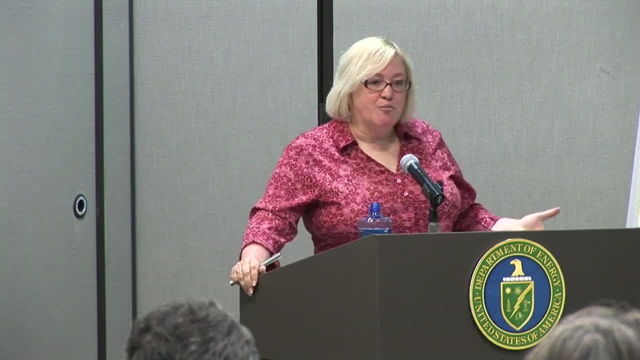 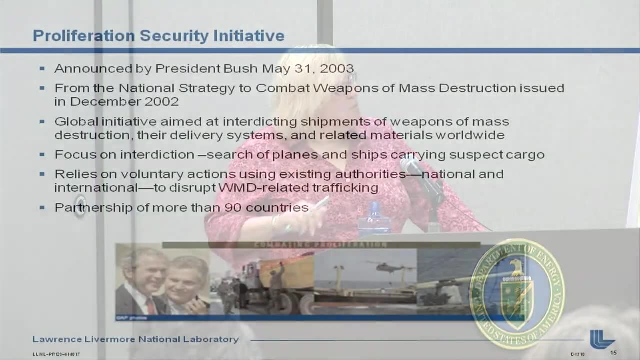 aimed at stopping the shipment of weapons of mass destruction, delivery systems and anything related worldwide. It's focused on interdiction. It's largely focused on the search of planes and ships that are suspect of carrying cargo that would support weapons of mass destruction. It relies on voluntary actions of existing authorities. It doesn't 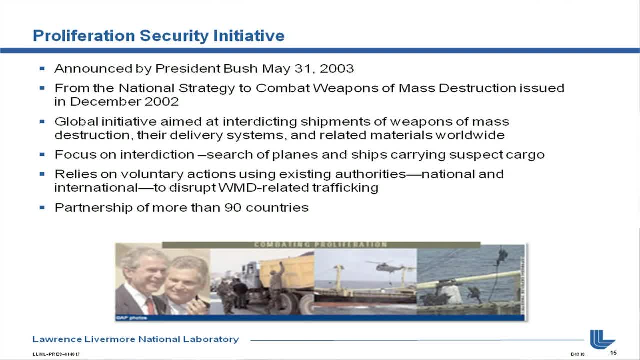 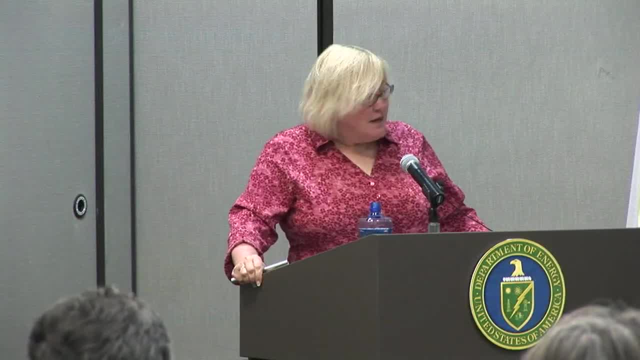 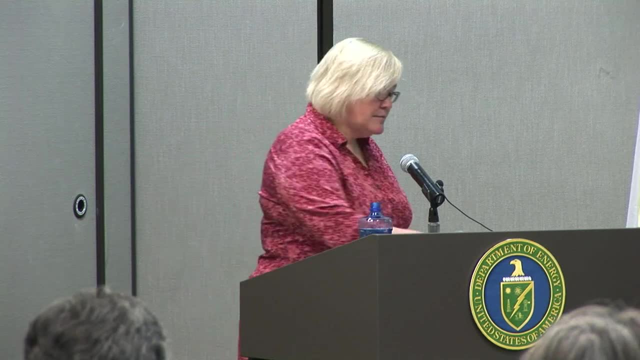 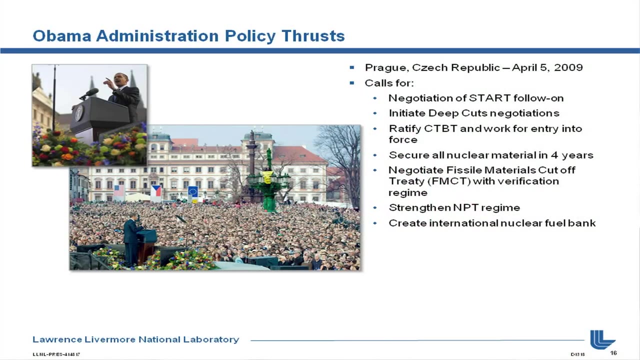 extend any law. It doesn't extend any legal domain. It relies on national and international laws. Think of it largely as a partnership that participate in law enforcement. Early in his administration, President Obama announced his administration's policy thrusts in the area of nuclear nonproliferation In Prague. he called for the negotiation. 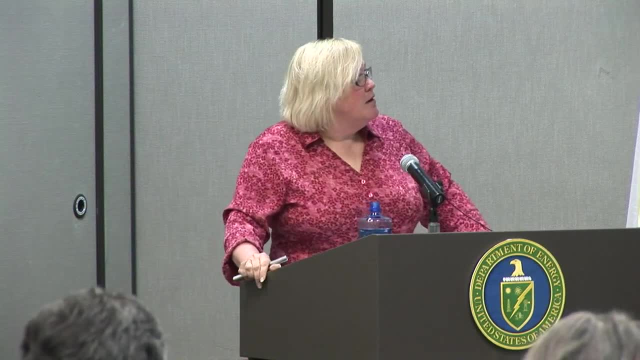 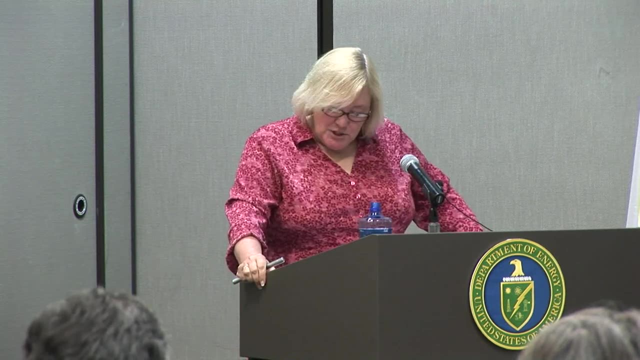 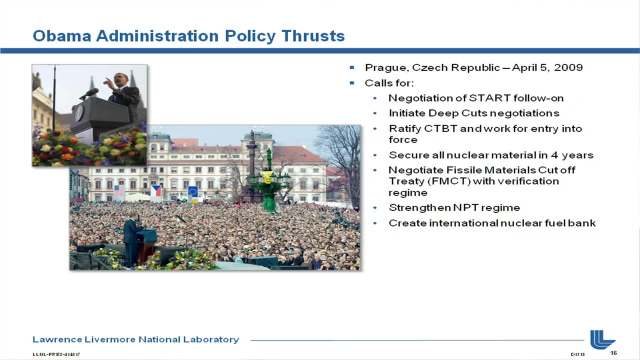 of a follow-on to the START treaty. initiation of deep-cut negotiations. ratification of the Comprehensive Test Ban Treaty and the subsequent work to bring it into force in the US and around the world. the securing of nuclear material around the world in four. 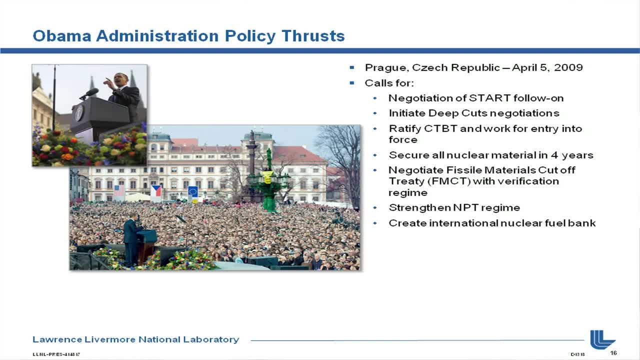 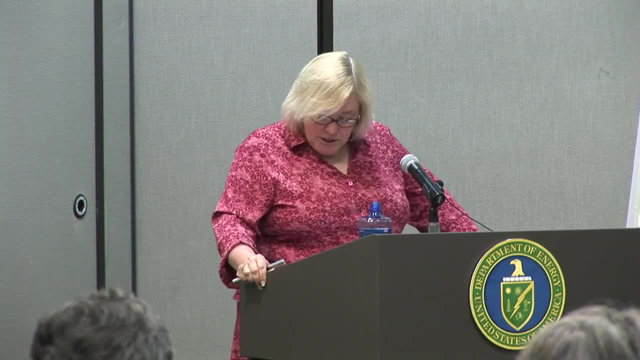 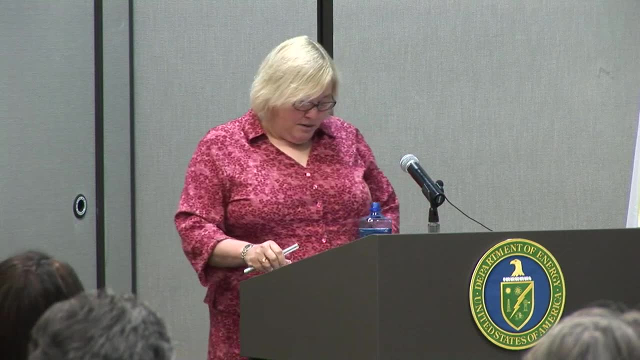 years, The negotiation of a fissile material cut-off treaty with its own verification regime, further strengthening of the nonproliferation treaty regime and the creation of a nuclear fuel bank, hearkening back to Eisenhower's request and concept in the Atoms for Peace talk. 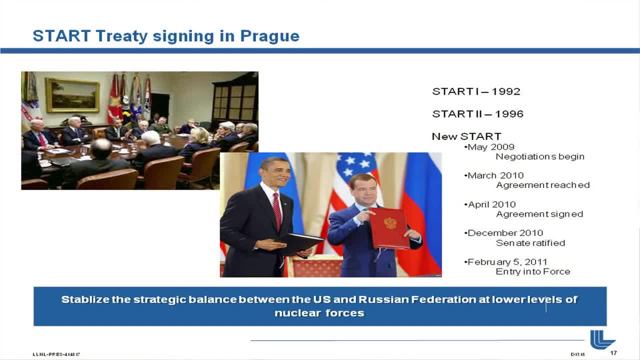 In fact, in the current administration, START now, START III, referred to as New START, is the first of its kind. In fact, in the current administration, START III, referred to as New START, is the first of its kind. The New START treaty was signed in April 2010.. The US Senate ratified it in December of that year And it entered into force in February of this year. You can see here Presidents Obama and Medvedev with their signed copies of the START New. START treaty. The pursuit of the New START is to stabilize, as it says here, the strategic balance between the United States and the Russian Federation at lower levels of nuclear forces, with both countries backing off on the size and scope of their nuclear stockpile. 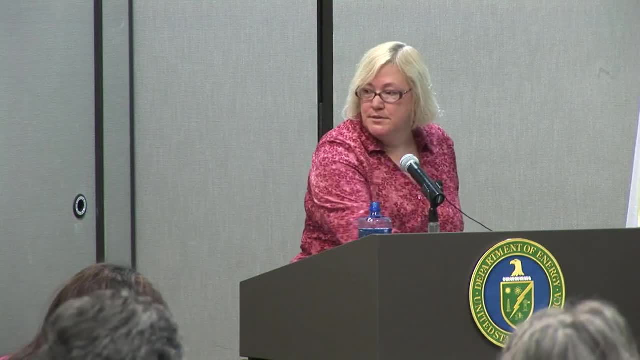 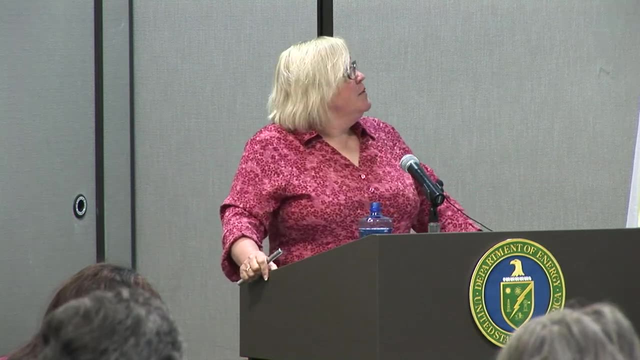 That's only between Russia and the US. That's only between Russia and the US. China's not involved. China's not involved. So we've talked about the regime. We now need to focus for a couple of minutes here, quickly, on what happens with the people. 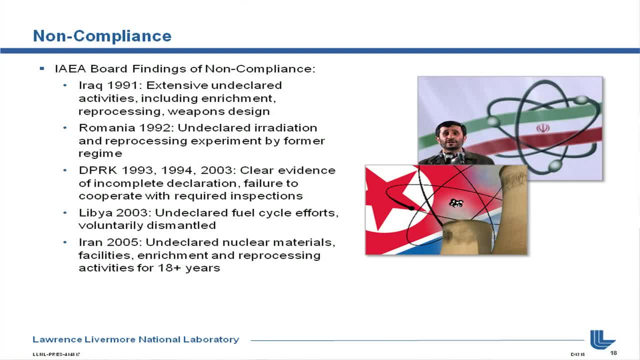 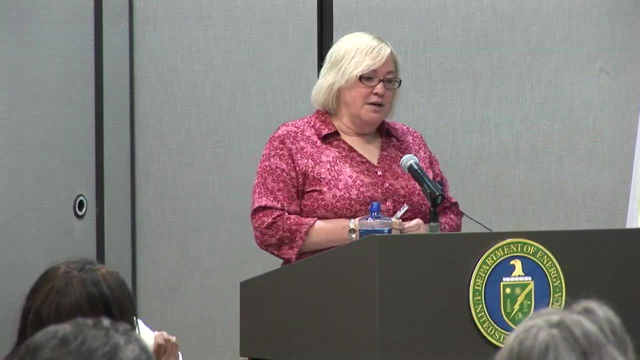 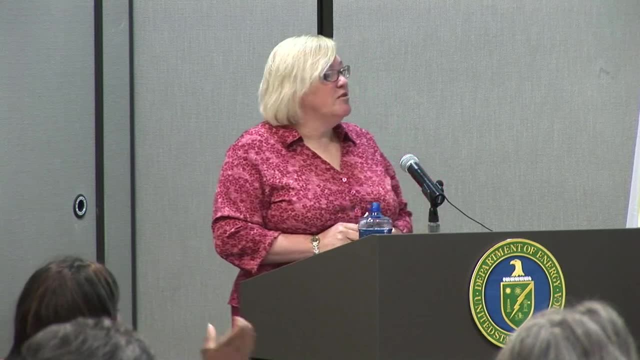 who aren't following the treaty that they've signed up to. We've heard one comment that's related to that. You can see here, in the process of the inspections that we outlined, that the IAEA is allowed to permit, allowed to undertake under the Non-Proliferation Treaty and the complementary 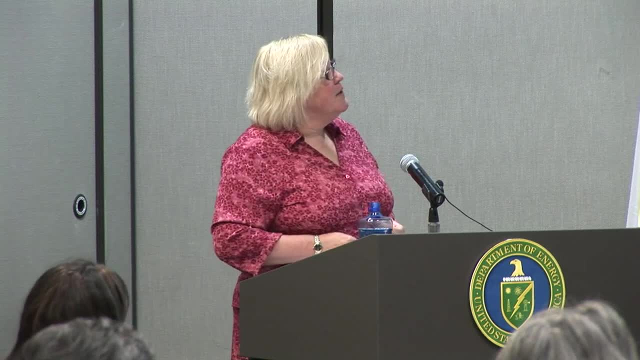 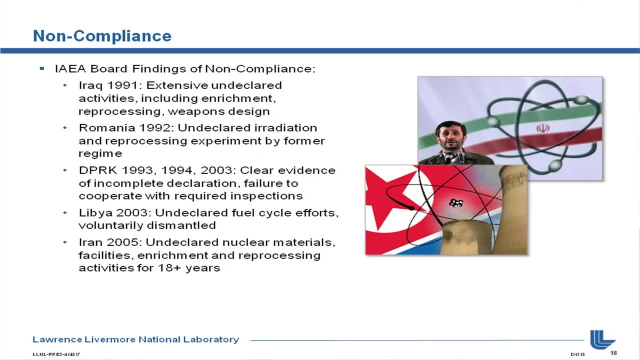 access and the additional protocol findings by the IAEA of non-compliance with the articles of the treaty. So what happens here? as I said, remember that the IAEA has a lot to do with the IAEA. IAEA has a lot to do with the IAEA. 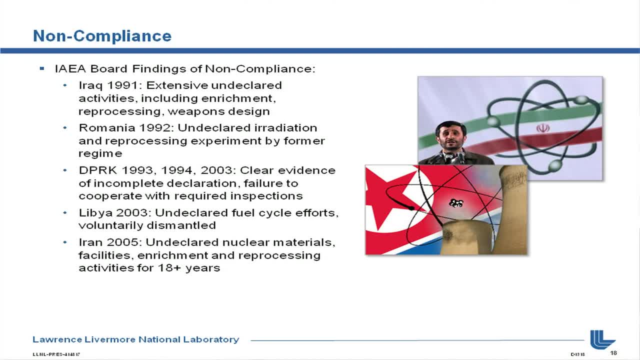 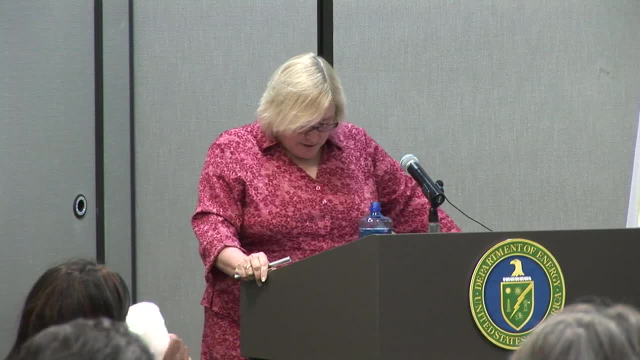 IAEA has a special relationship with the UN Security Council. This is where it comes in, So when the IAEA Board of Governors has a finding of non-compliance, something that's well specified what it is, they are obliged to report it to the UN Security Council. 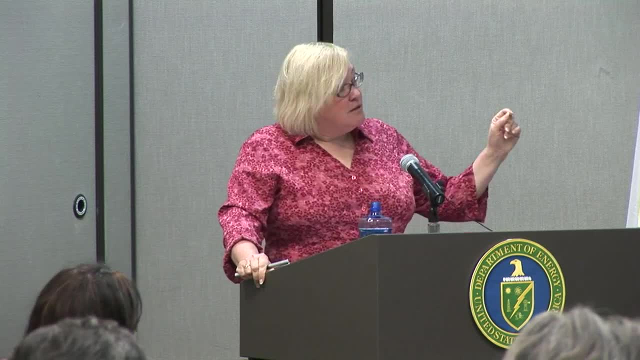 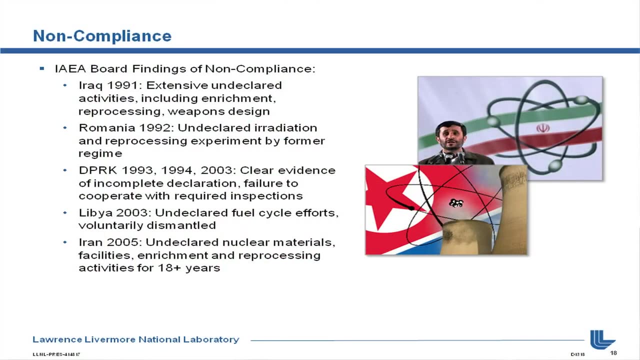 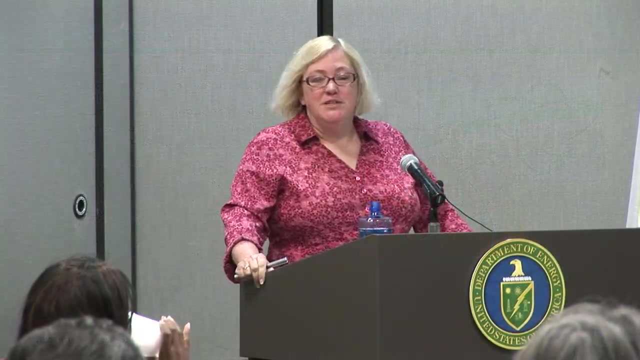 and to the UN General Assembly, And it is then that the UN is empowered to impose penalties and to use this as a carrot, if you will, to incentivize. And it is now that the UN is able to use this as a carrot, if you will, to incentivize. 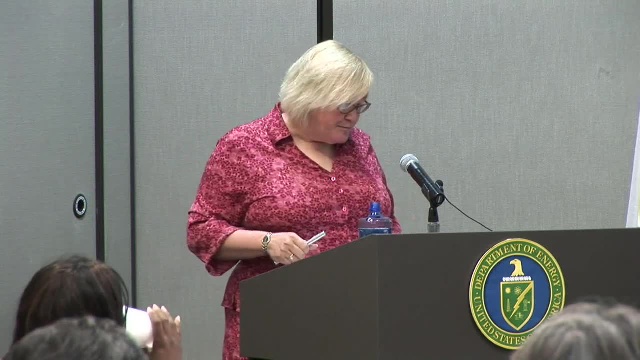 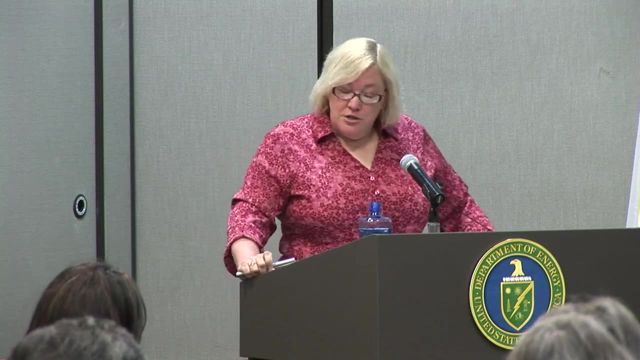 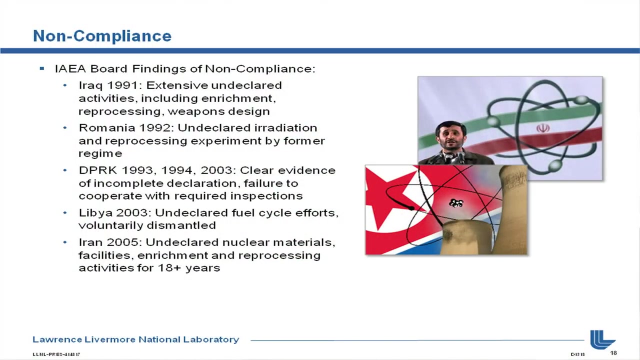 countries to comply with peaceful nuclear assistance. So that's the mechanism by which non-compliance is handled. So that's sort of the end of the policy piece of this talk. So let's just kind of do a quick review here. So there are three things that a state needs if they want to have a nuclear device. the 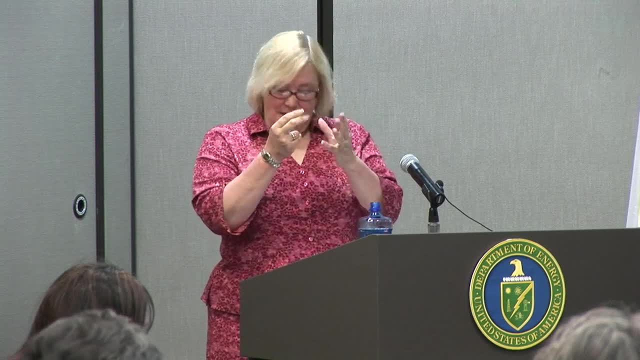 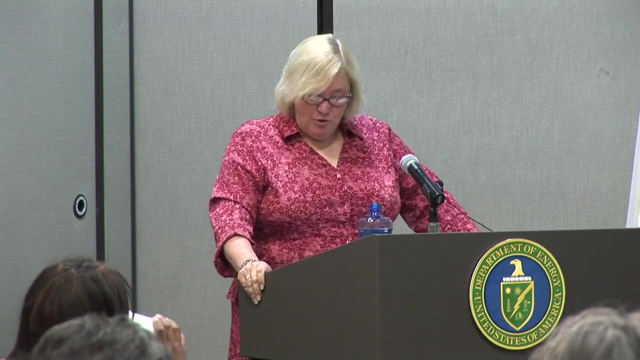 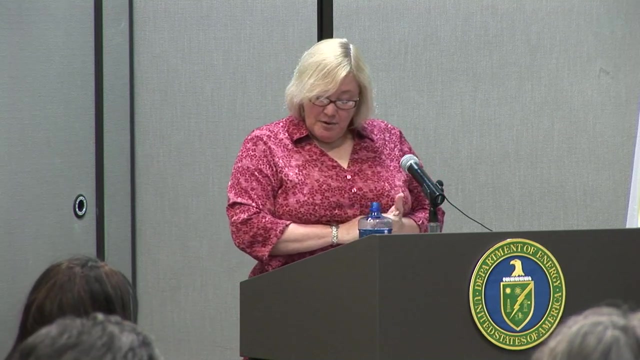 political will to make it so, the nuclear material to make it so and the technology to wrap all of that together. So, in terms of nonproliferation tools in the political will, we've talked about the nonproliferation treaty, we've talked about the complementary safeguards agreements and we've talked about 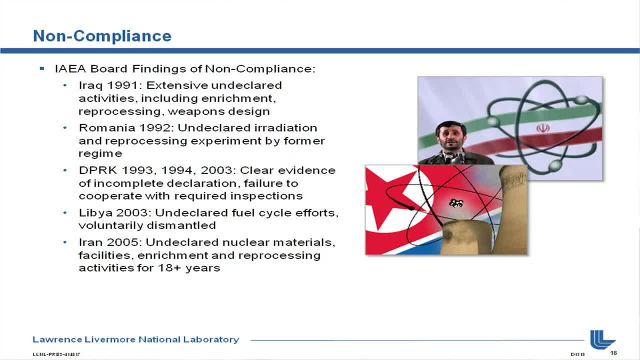 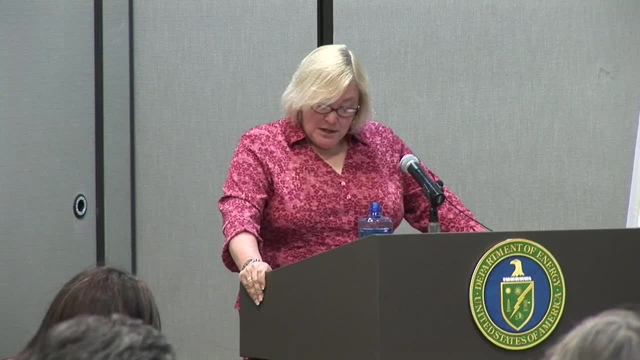 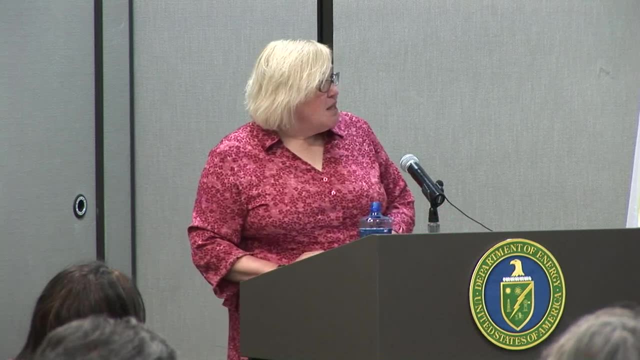 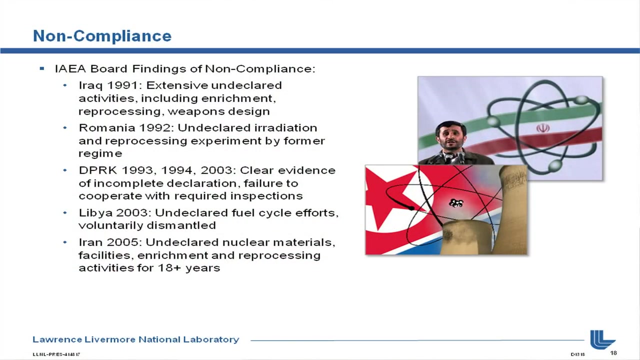 additional protocols. We've talked about non-nuclear weapons states foregoing any desire to have nuclear weapons, their right to be able to pursue peaceful nuclear activities themselves, and we've talked about everyone agreeing to pursue good faith negotiations on disarmament In terms of nuclear materials. we talked about states assuring the international community 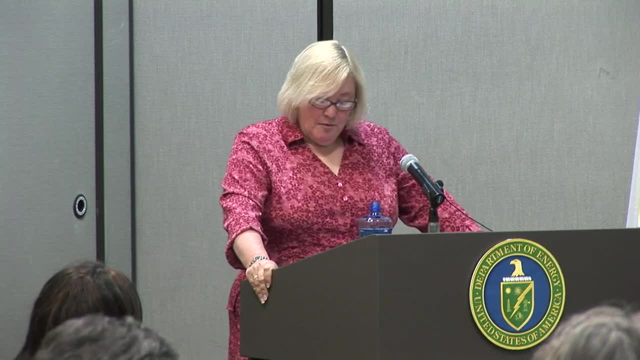 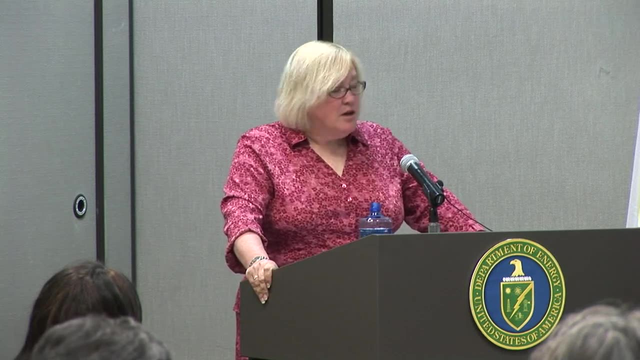 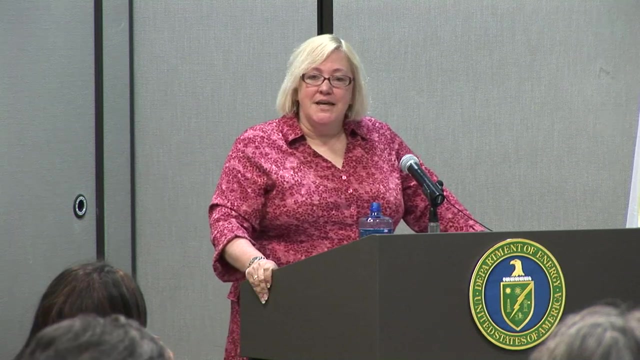 that they are good citizens of the nonproliferation treaty, using the concept of safeguards As a measure to verify that nuclear materials and facilities are in fact not being used for diversion purposes of nuclear material And the assurance of individual states that non-state actors are not having access to. 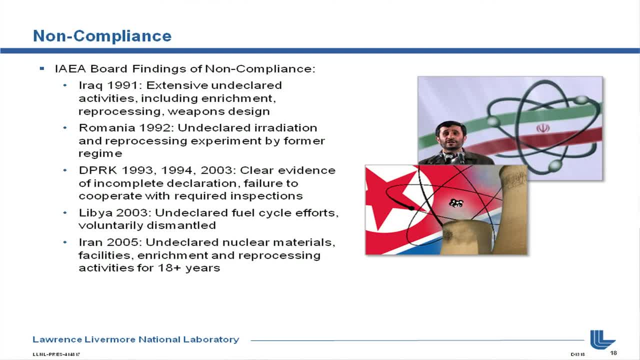 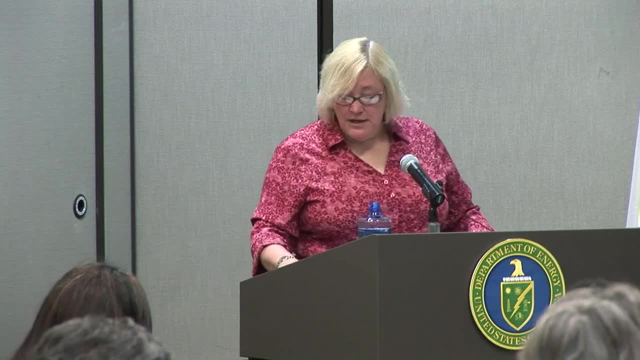 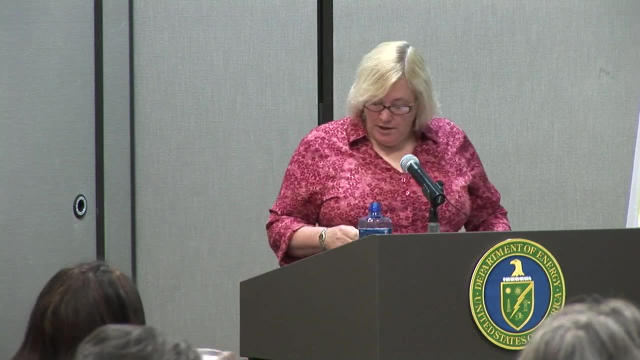 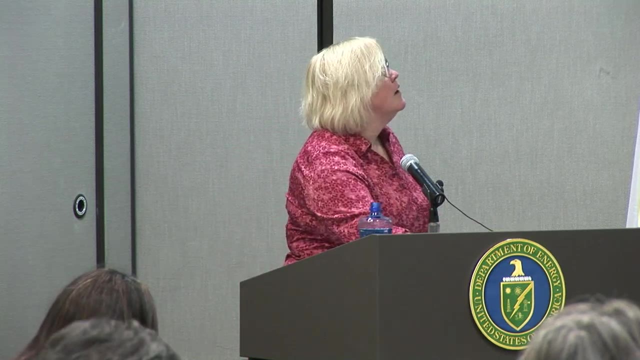 nuclear material through the use of security and physical protection measures, And we've talked about the limiting of nuclear technology spreads Through export controls. that is what the Zanger and the Nuclear Suppliers Group are charged with monitoring. So what I'd like to do now is transfer to what do you do to verify all of this right? 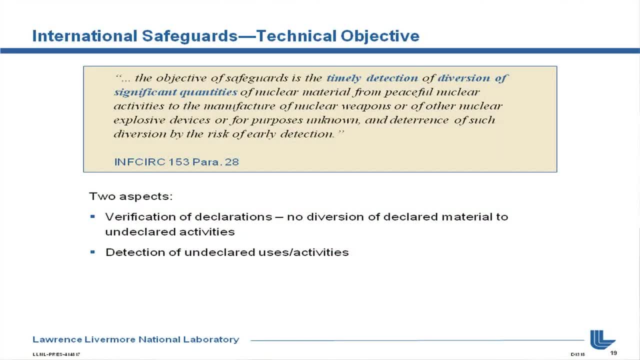 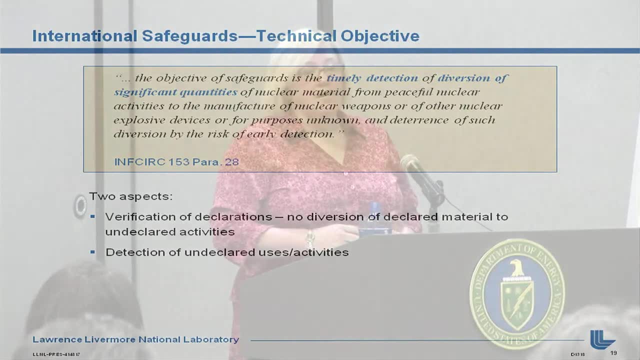 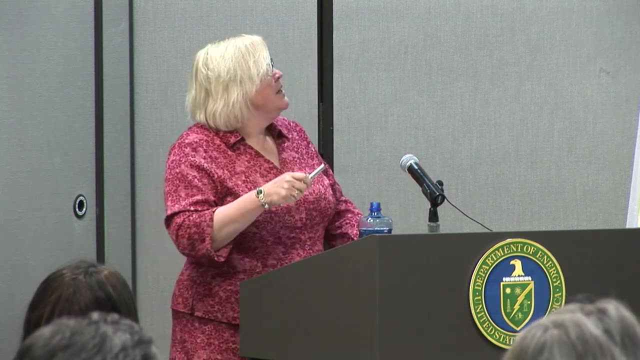 So that's the words, that's the policy, that's what everyone's agreed. So what are the tools that people use, countries use the IAEA use to demonstrate that they are Are compliant and acting in good faith. You see here the technical objective of international safeguards and I've highlighted the words. 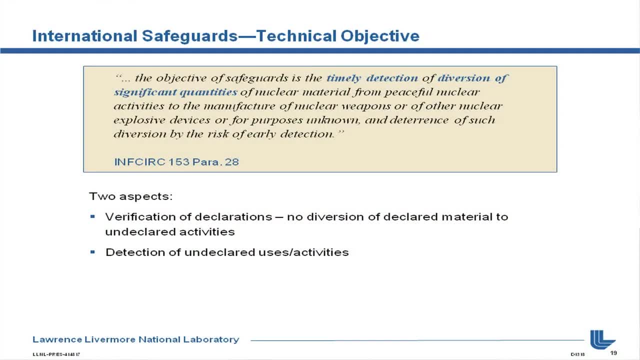 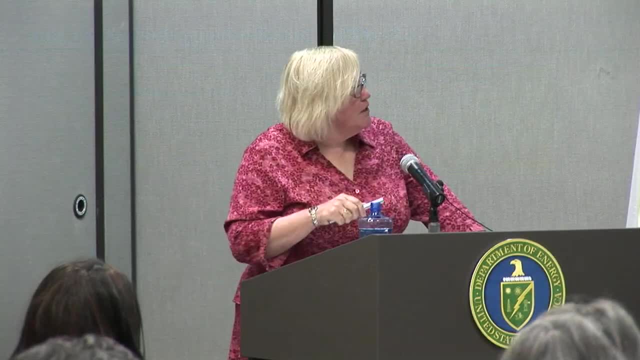 that are important here, that is, the timely detection of diversion of significant quantities of nuclear material. We'll get to the definitions of those here in a minute, But it's important to point out that there's two sides to this diversion of nuclear materials. 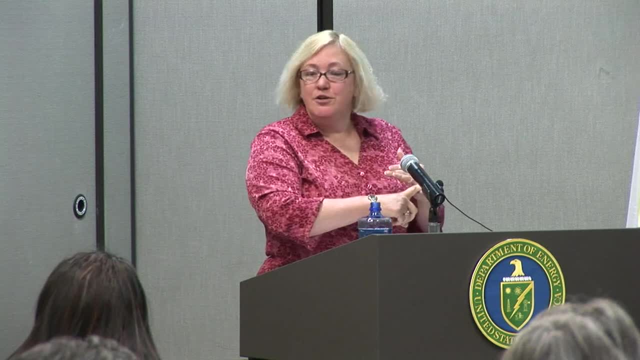 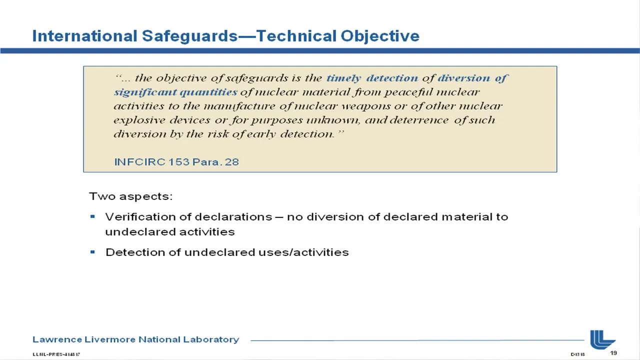 One is: You want to verify that you're doing what you said you were going to do with the material that you declared, that none is being diverted for undeclared activities. On the other side of the coin, you want to be sure that everything that people 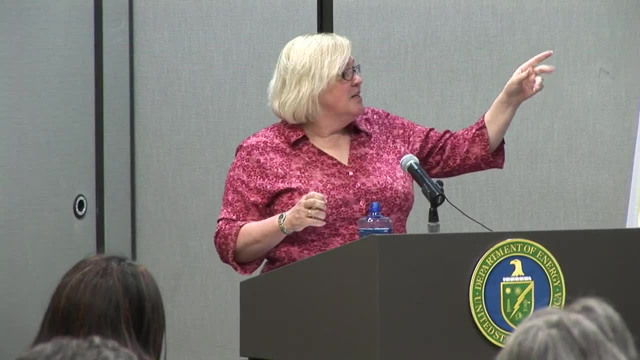 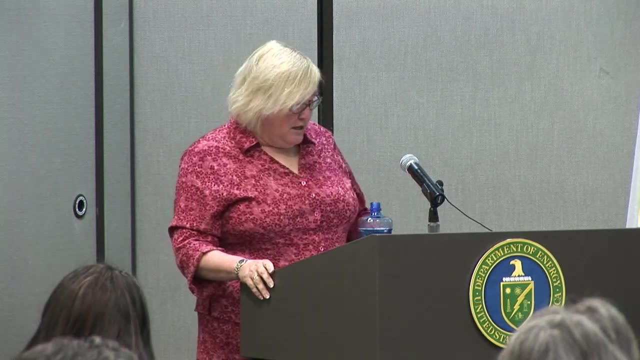 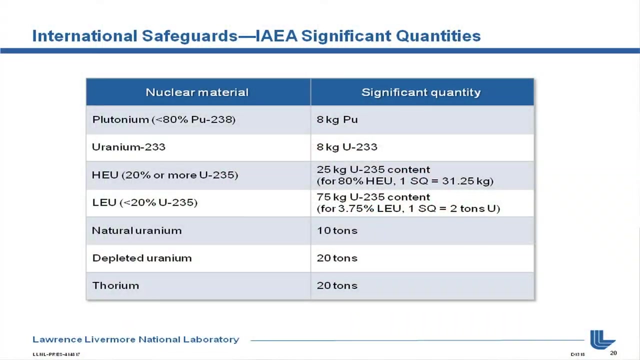 That they are not doing nuclear activities that they haven't declared. So both of those are the subject and the concern of the IAEA in their inspection processes. So here you see a table. This is the closest thing to chemistry, I think, in the talk. 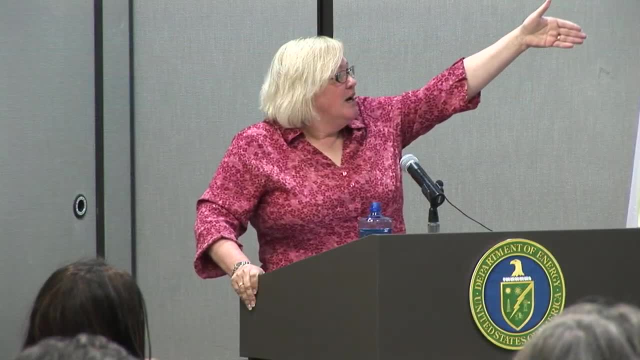 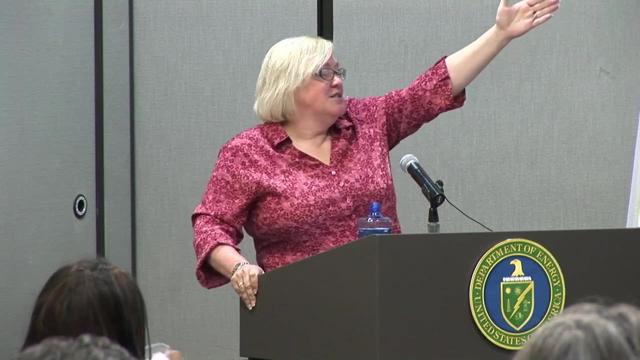 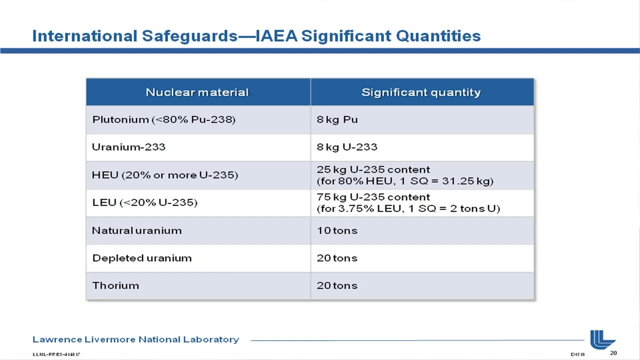 And you see here that nuclear materials of interest to the IAEA and you see what's called a significant quantity, That is the quantity of that isotope or that combination of isotopes that the IAEA is interested in. And you can see that it varies depending on the material. 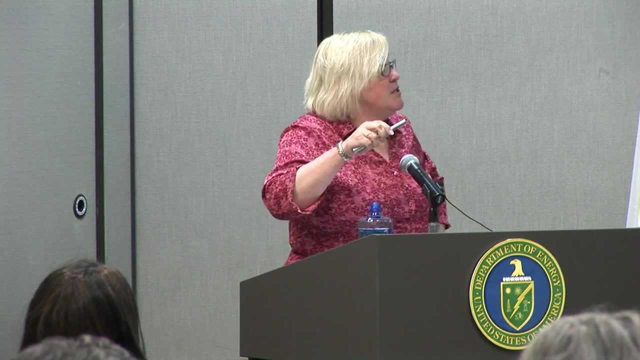 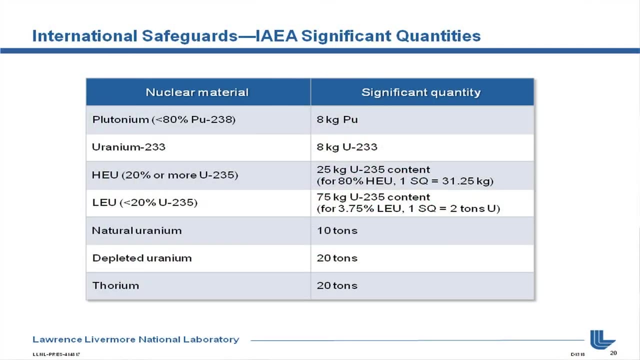 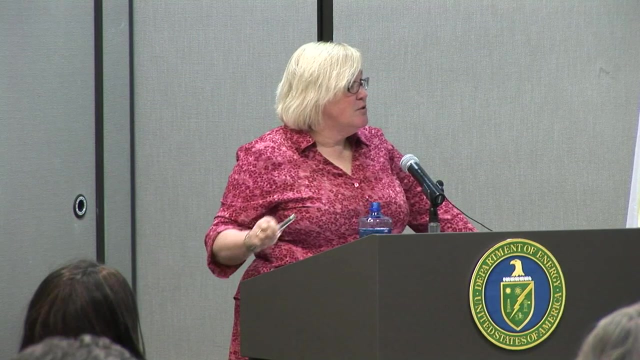 So here we have less than 80% plutonium as PU-238.. The IAEA is interested in tracking it down to essentially the 8-kilogram level And that goes up in quantity, for example down to thorium at 20 tons. 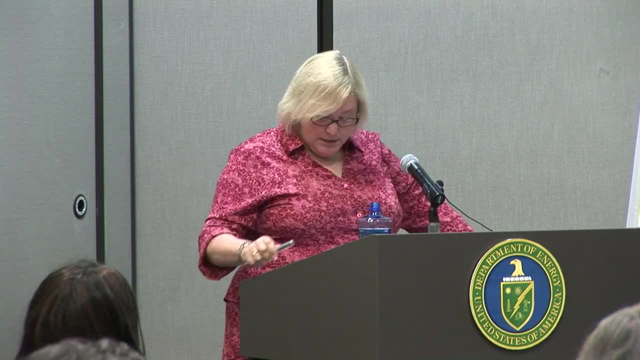 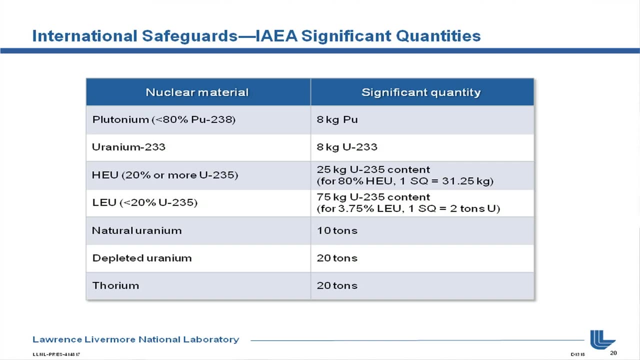 And you can see the highly and low-rich uranium in here and the quantities that attract attention. We also mentioned timeliness goals. that is, how soon do they want to know that quantity of that material is not where someone has said that it's supposed to be? 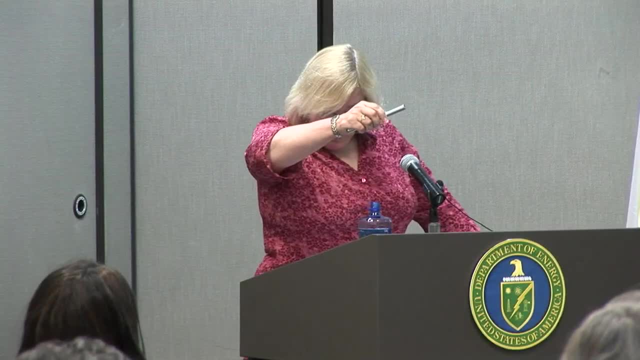 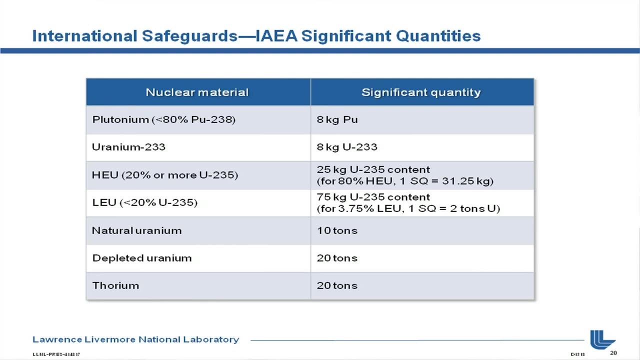 And the numbers. the timeliness goal, for example, for the plutonium is one month. If you're missing 8 kilograms of plutonium, they want to know about it in the month time frame Again and it's largely risk-based down to thorium, where it's one year. 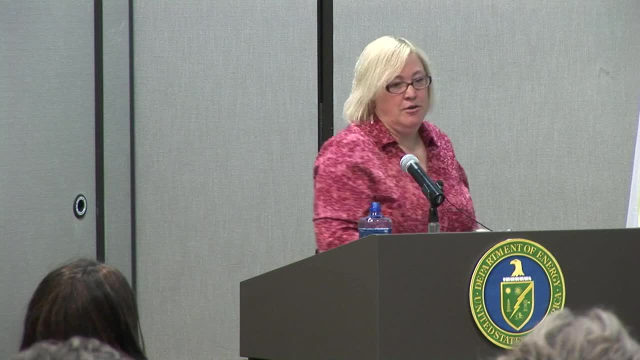 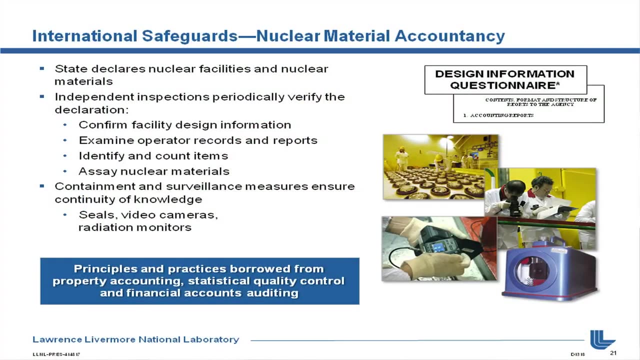 Okay. Well, how do you keep track of all of that nuclear material in a verifiable way That introduces- That's the concept of nuclear materials accountancy? Think of it just as bookkeeping. Think of it just like a bank keeping track of their money. 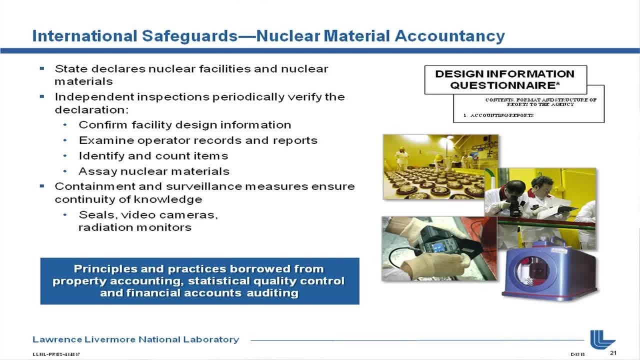 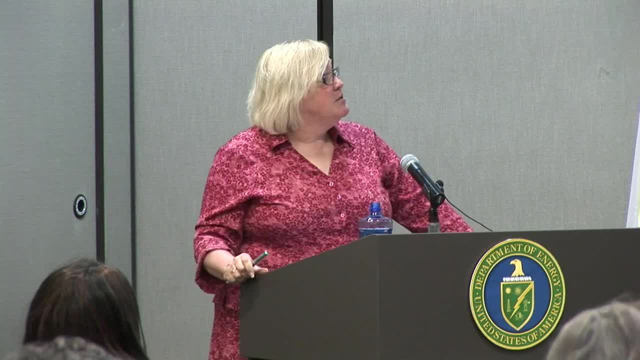 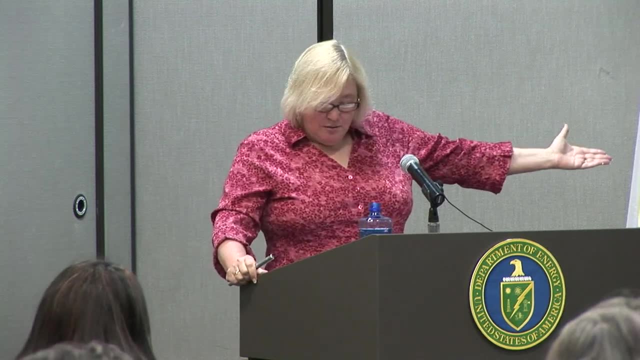 Everybody keeps track of their nuclear material in the same fashion. So remember, states are obliged to declare their facilities and their material. Independent inspections periodically verify that the building is built and the facility is built the way you said it was. They do that by looking at records and reports. 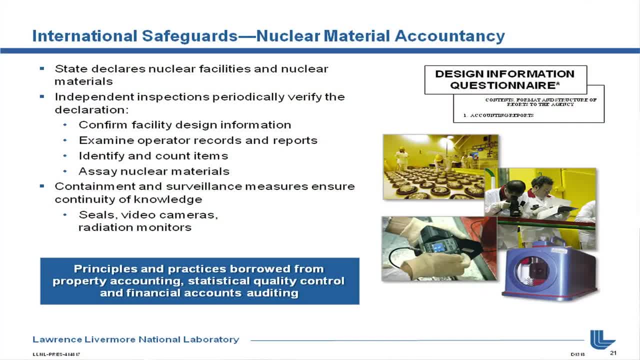 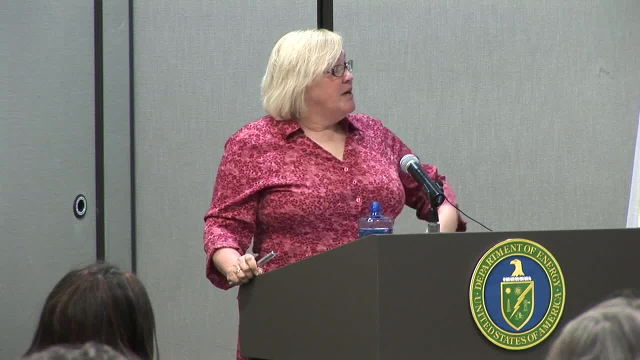 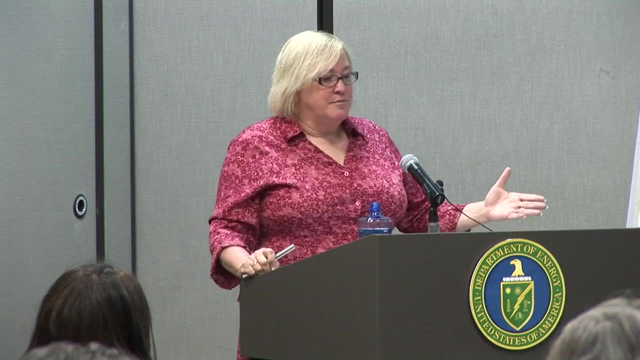 They identify and count items and then they assay nuclear materials. They monitor the containment and surveillance of materials to ensure that you know the continuity of knowledge chain of possession, if you will- And you can do that with seals, video cameras and radiation monitors- 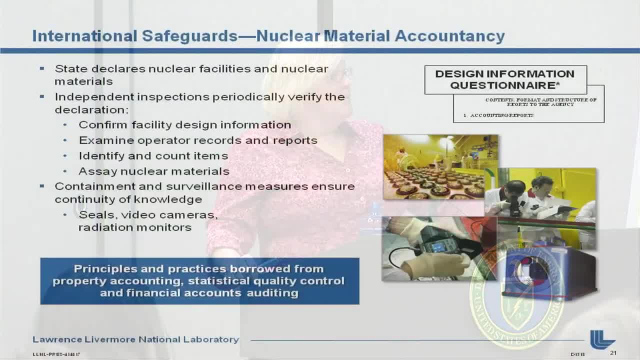 So, as I said, this should come as no surprise. This is, you know, like how anybody keeps track of their money, But they do that, They do that, They do that, And you can actually see here IAEA inspectors counting items. 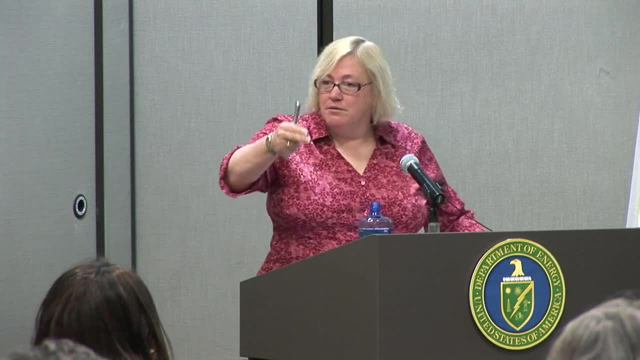 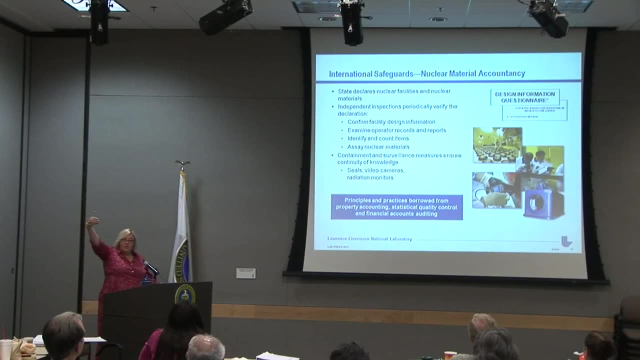 They are in a nuclear facility and they're counting bins or they're counting barrels And you can see them assaying material. This is, I believe, a Los Alamos-designed video camera. You can keep things under surveillance continuously. for video cameras: 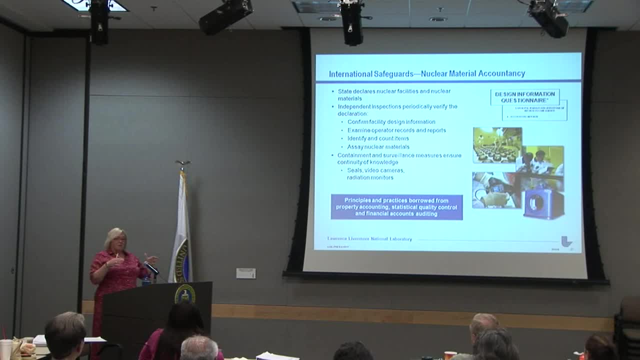 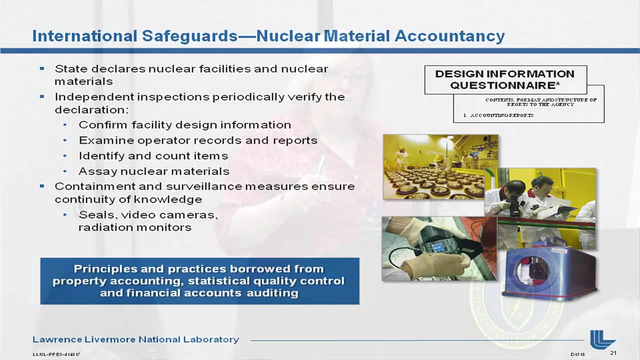 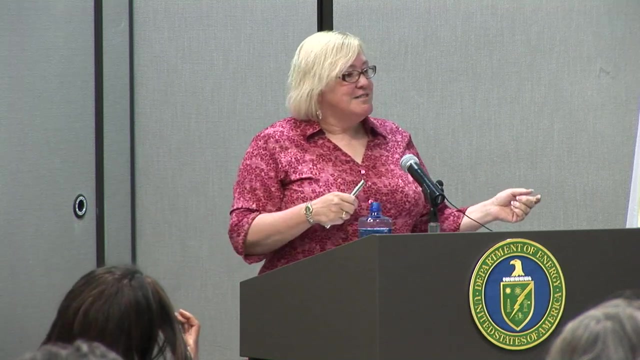 Remember the important thing is IAEA inspectors come from all the other member countries And remember that the IAEA is obliged to protect your proprietary equipment. It's proprietary secrets. So that's why it's often counting items. It's counting drums, not necessarily knowing what's in the drum. 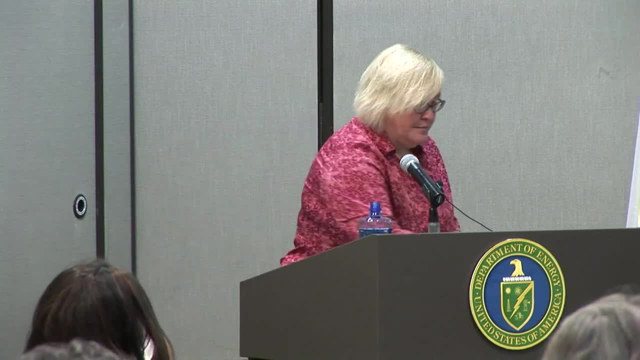 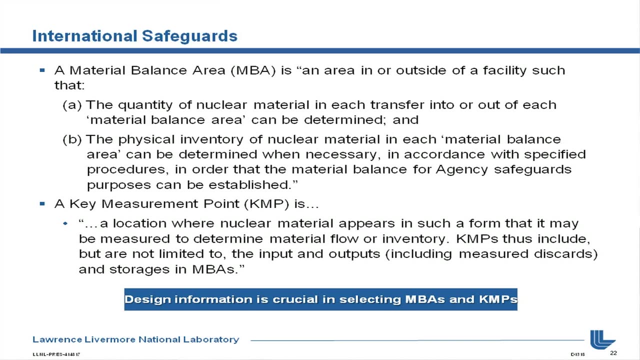 We'll come to that a bit later. Okay, so how do you keep track of all of this? You've got to have some kind of file folder that you keep all your data sorted into, And how do you keep track of all this material moving? 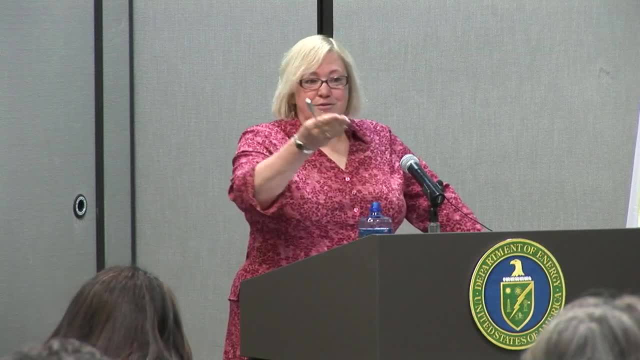 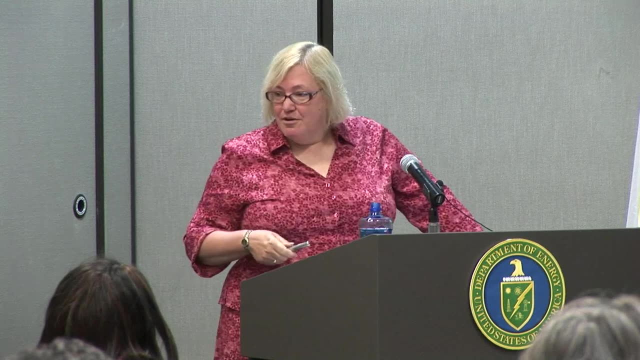 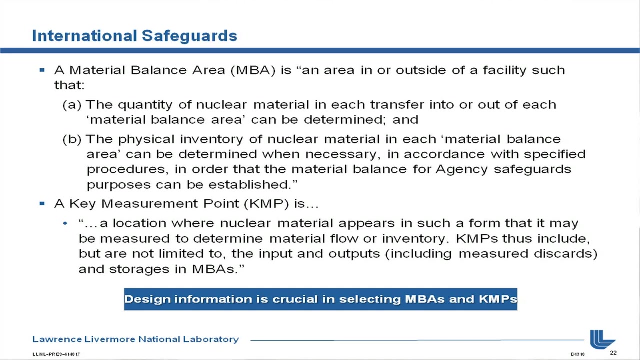 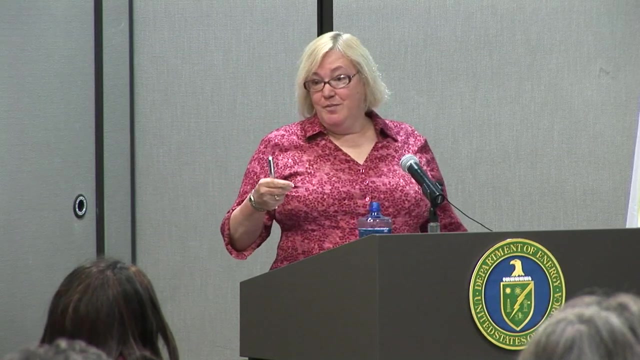 We've seen some pictures of some plants. We've seen both photos. We've seen as-built diagrams. These are not simple buildings to keep track of material flowing, So this introduces a concept called material balance area. It's a subset or an area inside the facility such that the quantity of material in each transfer into or out of that area can be determined. 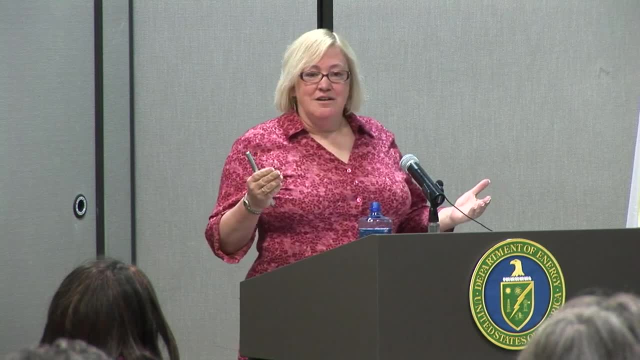 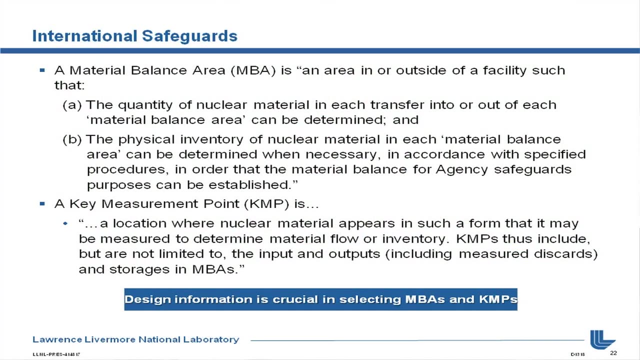 And at any moment in time, you can take a snapshot of what you think is in that material, what you are declaring is in that material balance area At any given time. The next concept is key measurement point, And that's basically you've got to be able to measure when you go from one subset, one material balance area, to another. 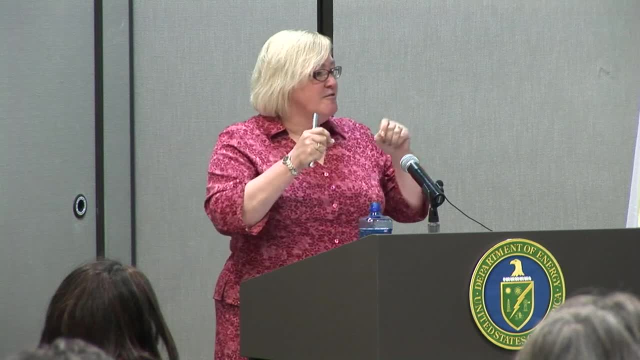 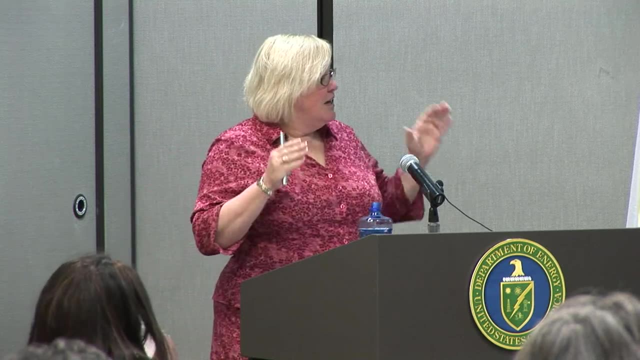 you've got to be able to have some kind of little mini sender-receiver validation that you're going to transfer it from the inventory of one area to the inventory of another. Again, you've got to be able to do all of that, document it and have it verified. 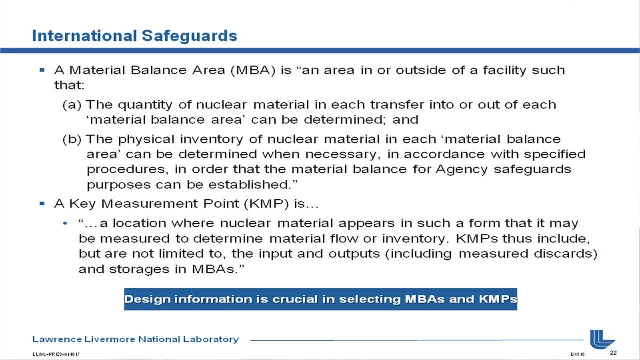 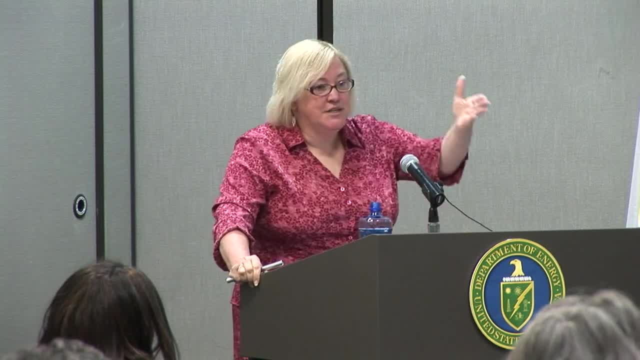 while you retain the safeguards. So that's the confidentiality requirement of the country whose facility that you're looking at. And again, I'll point out, you've seen some of these pictures of facilities. This is not as simple as it might sound. 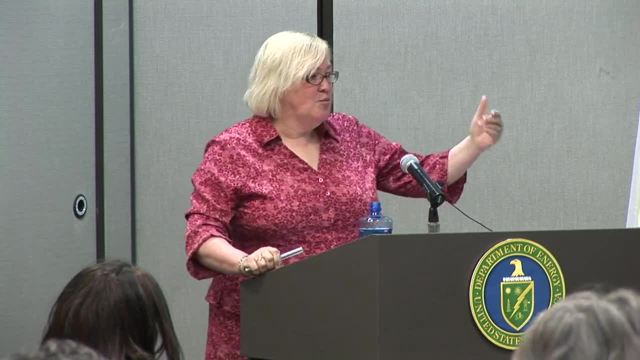 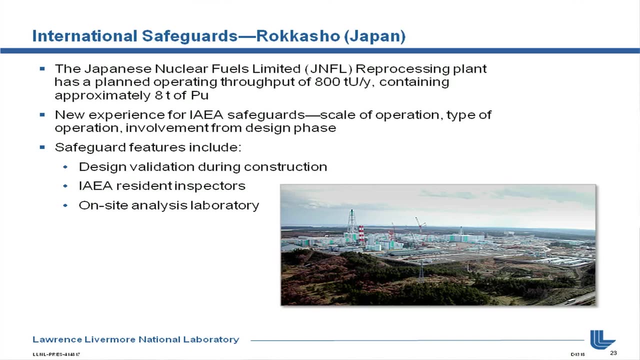 So let's just take Rakosho. We've used this as an example a couple of other times this week. This is the JNFL reprocessing plant. It had planned operating throughput of 800 tons of uranium a year and approximately 8 tons of plutonium. 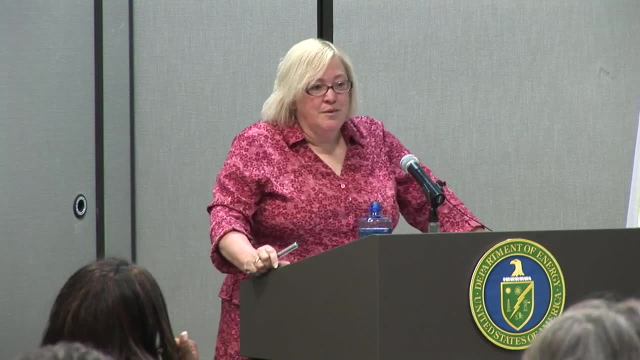 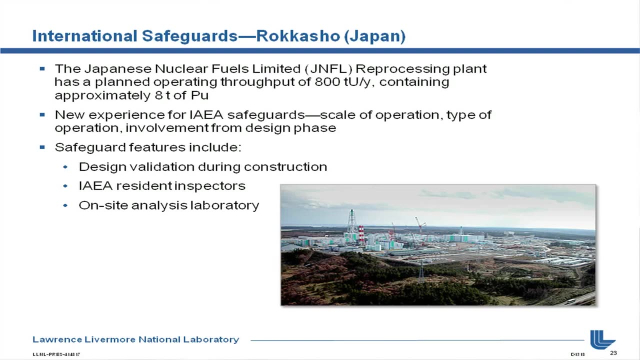 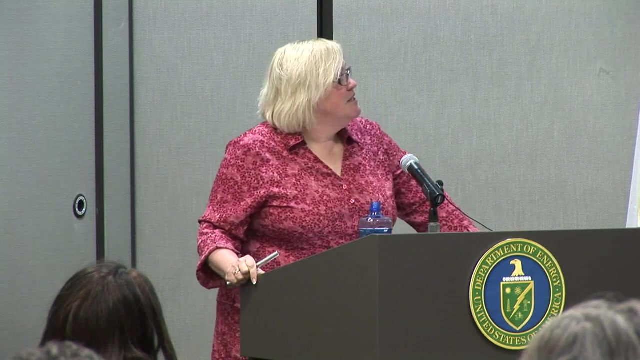 Recall the number that were. the de minimis number of plutonium that we're keeping track of here is 8 kilograms out of 8 tons. So this was a whole new process for the IAEA Safeguards Organization, just because of the sheer scale of this activity. 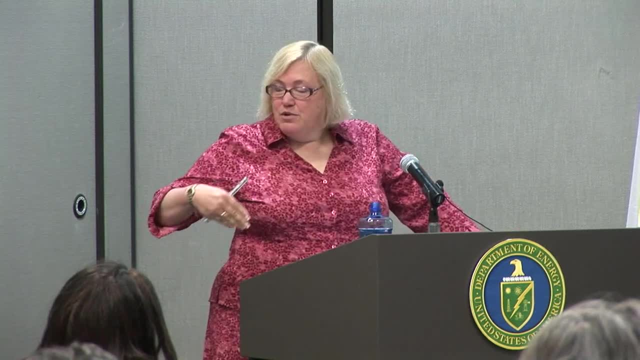 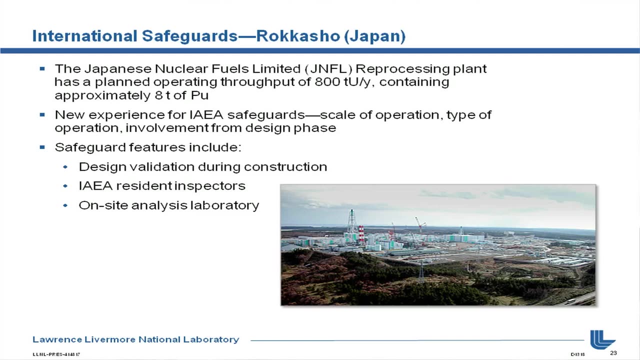 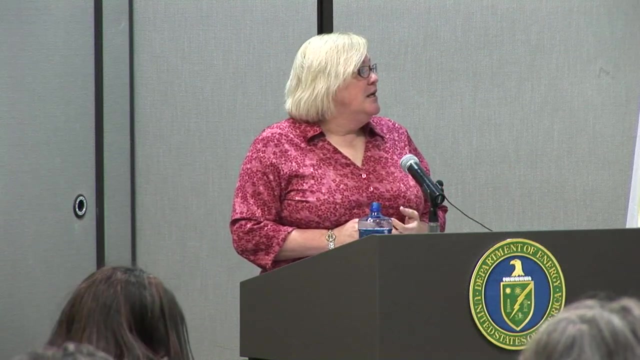 and because they were allowed to be able to be involved in the safeguarding of this plant right from the design and construction. They've been able to do the design validation of the facility as they built it. There are on-site IAEA inspectors. In fact, they've built their own lab right on site as part of the construction of that facility. 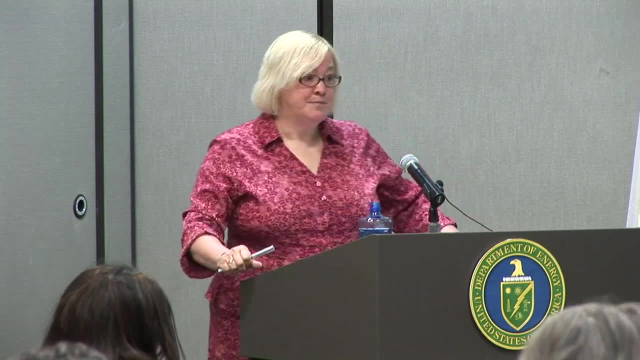 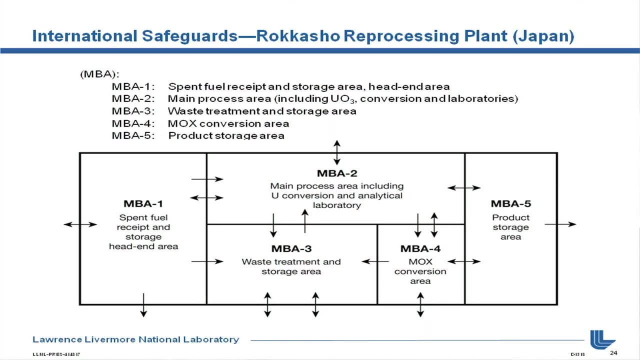 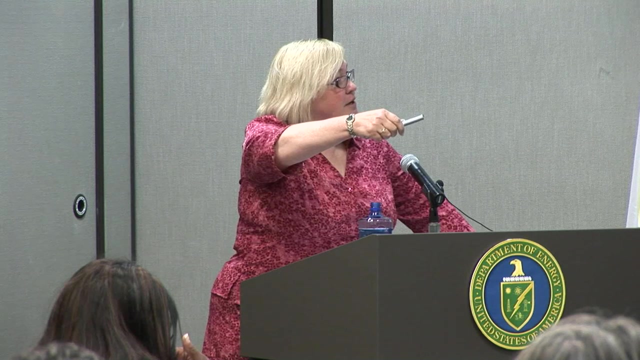 So let's look at how they would lay out, for example, their material balances area in a sort of schematic notional way here. So you can see as the processes we've talked about in reprocessing: spent fuel receipt, storage, head end area, main process area, uranium conversion. 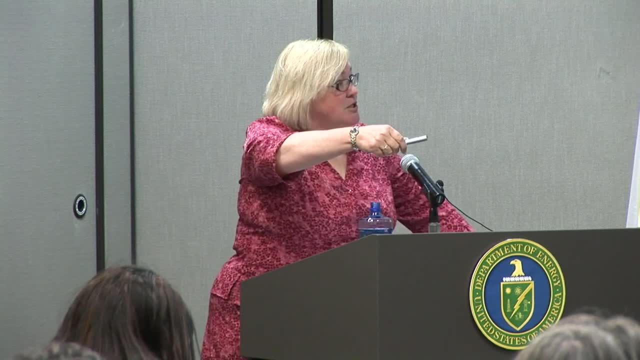 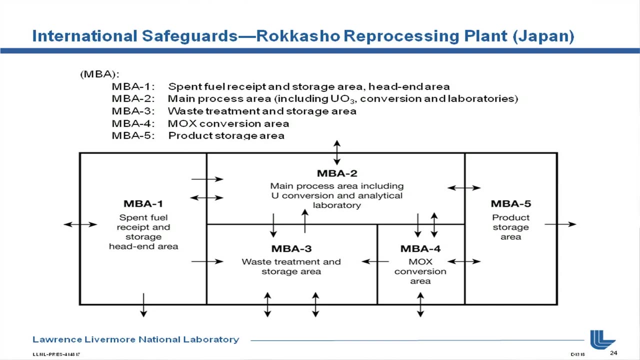 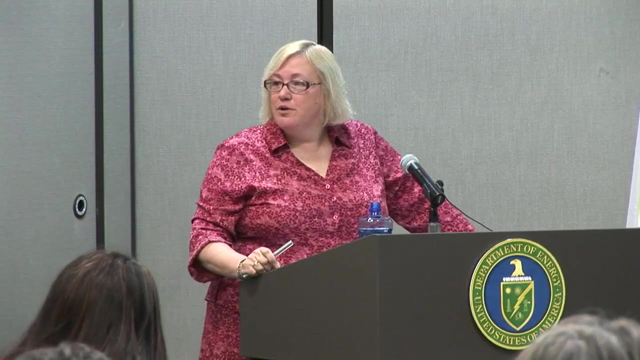 analytical laboratory, waste treatment and storage, conversion to MOX and a production storage area. So you think those are kind of the gross bins of what happens in that facility with those processes And they've defined notionally here you could do five material balance areas. 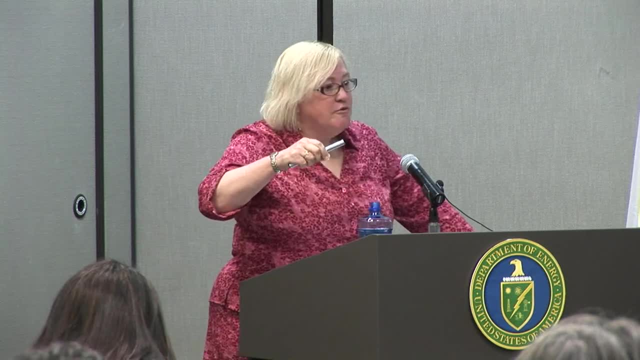 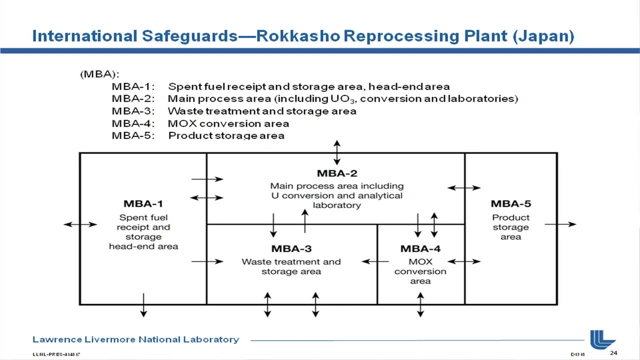 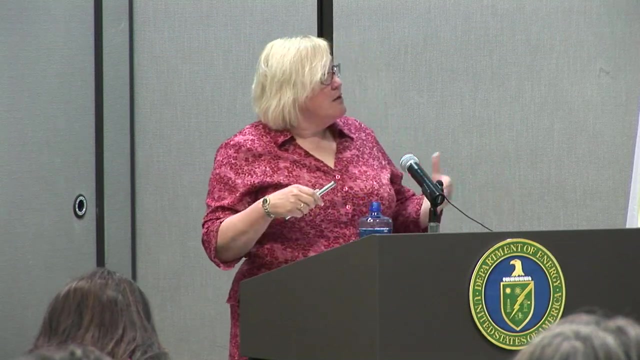 And each one of those arrows represents material flow from one material balance area to another, and a place at which you have to have a key measurement point so that you can validate the amount of material moving from MBA I to MBA II, for example, And at any moment in time you can validate how much material is in each one of those sectors. 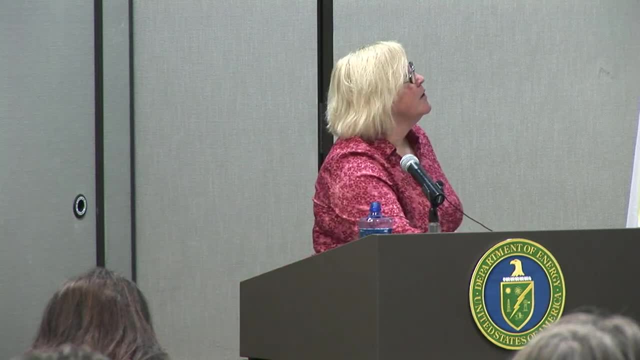 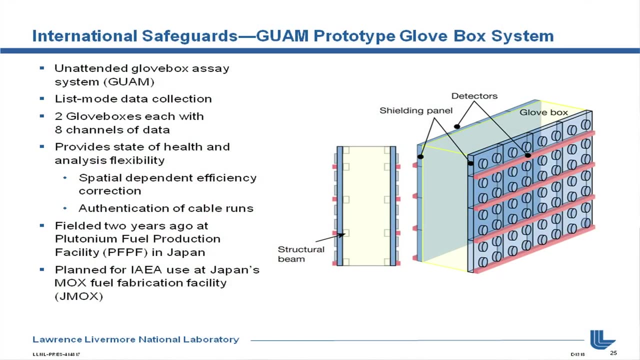 So how do you go about doing that, given the quantities that we've talked about? Here is an unattended glove box system. I believe it's also a Los Alamos design. You can see it's a multi-port glove box. These red channels represent detectors and the shielding is in the dark blue. 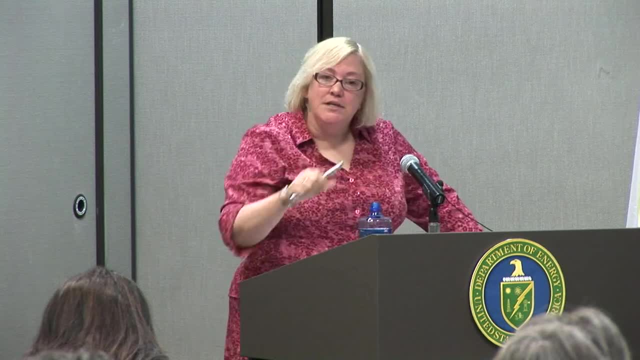 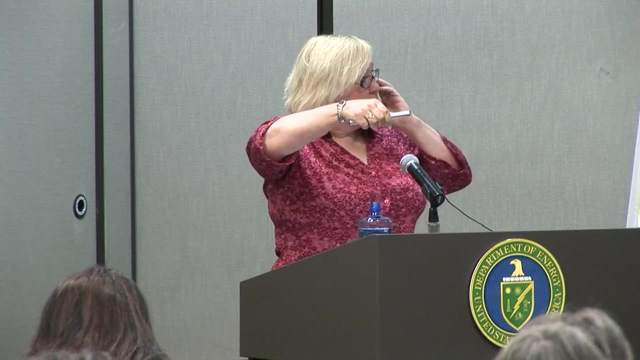 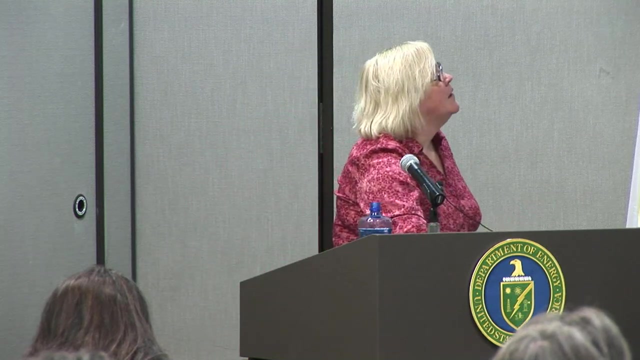 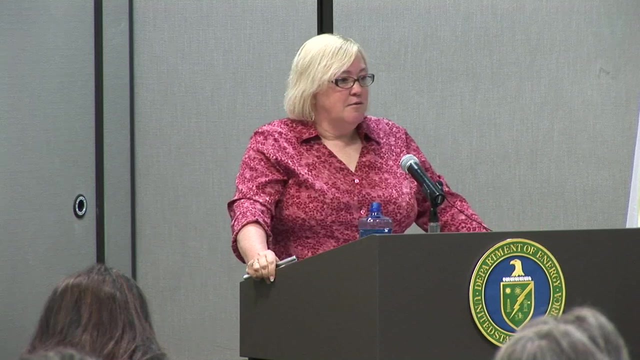 So it's important to go through all the R&D associated with this so that it's calibrated with respect to spatial location of material compared to the detectors, And this is planned for use in Japan. We've really only talked about the one peaceful use of nuclear material, and that was power. 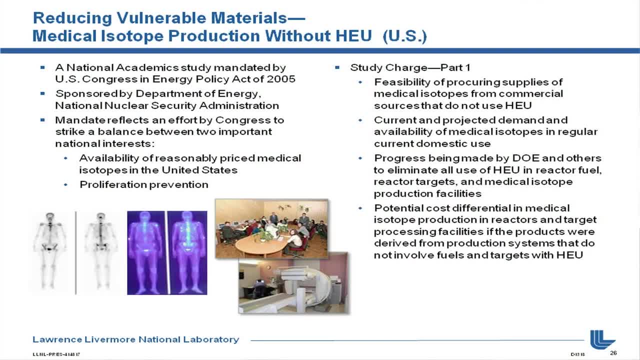 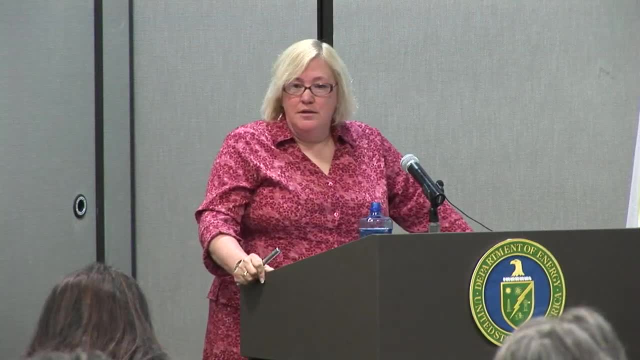 That's not the only peaceful use of nuclear material throughout the world. Here we show another one. This is on medical imaging, nuclear imaging. One of the most widely used isotopes in medical imaging around the world is technetium-99, which is derived from molybdenum-99.. They milk the cow to get the technetium. But you need this sort of continuing source of molybdenum because it has a relatively short half-life. Much of that molybdenum was, at least five years ago, being produced around the world. 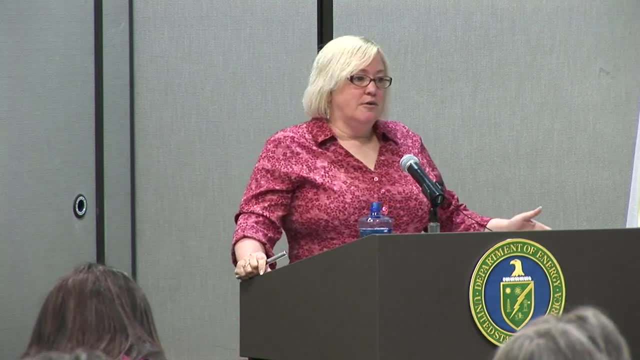 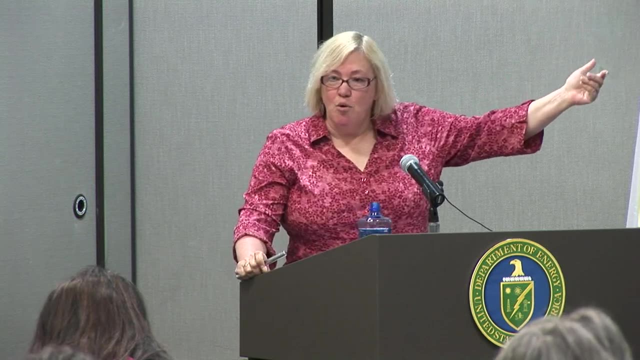 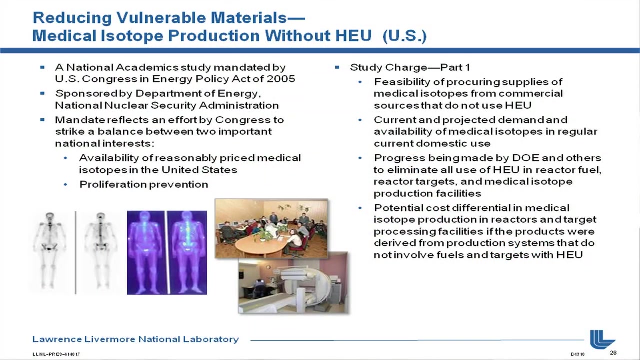 in reactors that had highly enriched uranium fuel and or highly enriched uranium targets. Highly enriched uranium, if you recall, is one of those materials that we like to track at a relatively small quantity in a fairly short time period. So US Congress asked the National Academy of Sciences to undertake a study to evaluate. 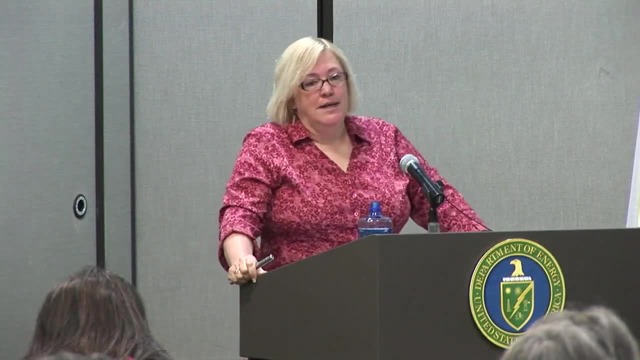 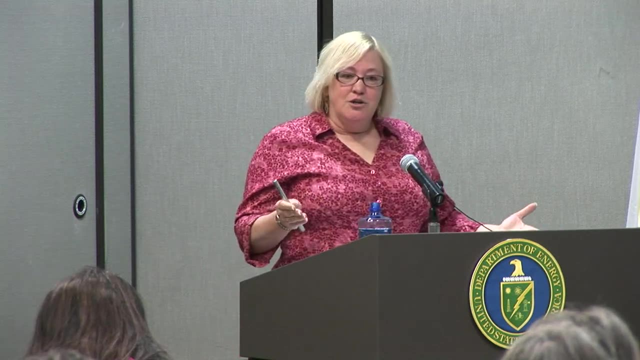 Here's the charter for that group. Ray Weimer and I were on that team And the bottom line question that they really wanted the answer was: without huge cost impact: could the world produce molybdenum for medical imaging using low enriched uranium? 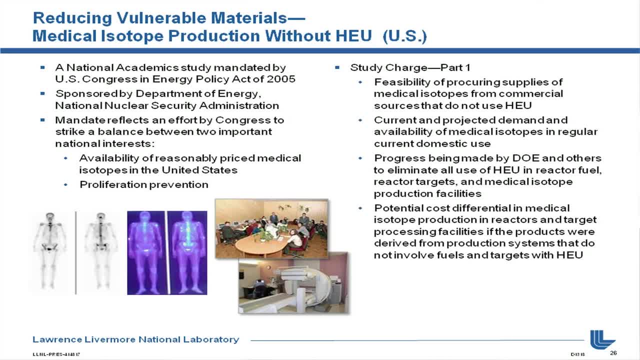 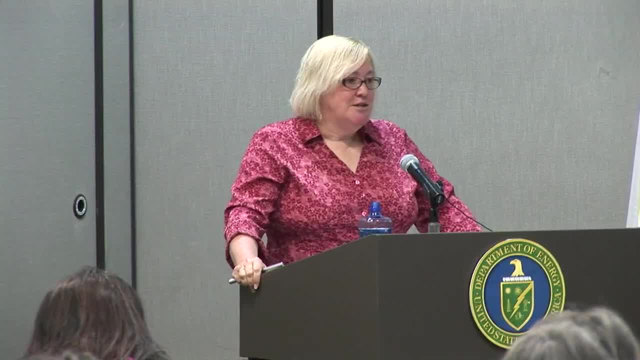 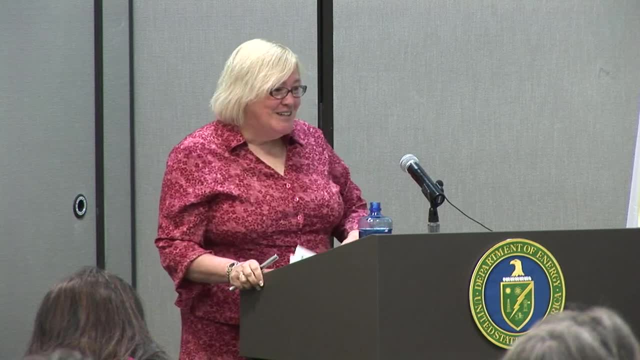 Instead of high enriched uranium. Our conclusion was: yes, they can do that, And in the five years since we finished that, we have seen any number of companies switch from HEU to LEU And stay tuned. It's kind of interesting to watch. 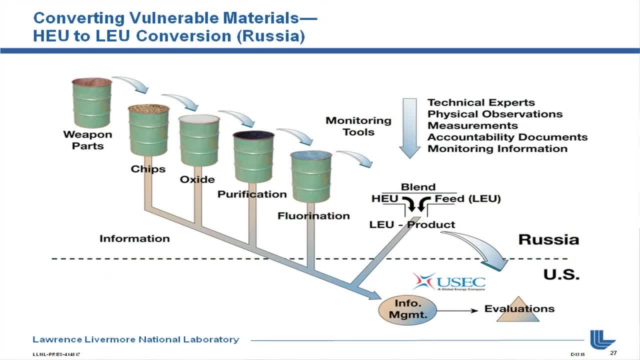 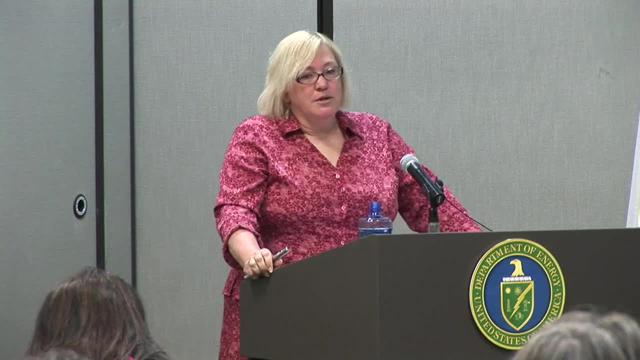 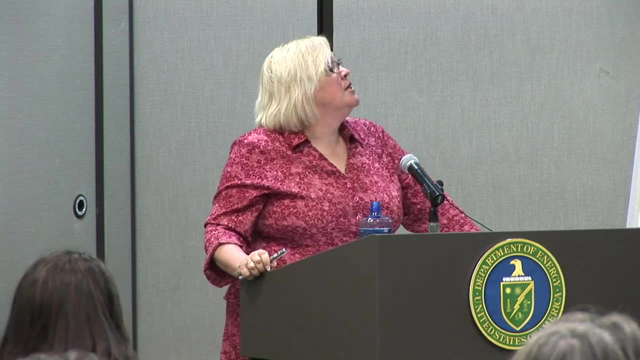 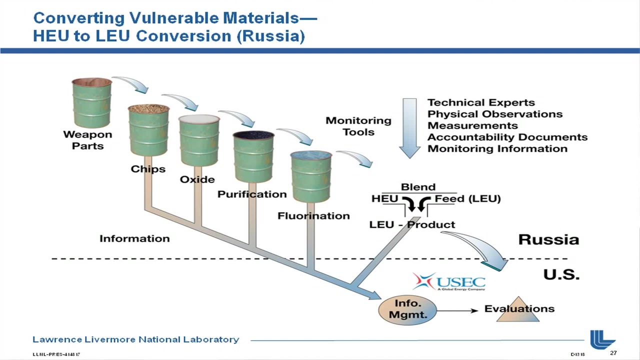 One of the requirements and one of the discussions we've had was that countries would start to build down Nuclear stockpiles And that they would agree to verifiable disarmament. The United States and Russian Federation have an agreement by which the United States buys LEU from Russia. 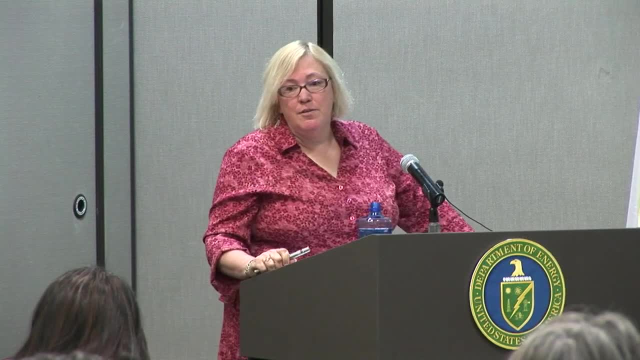 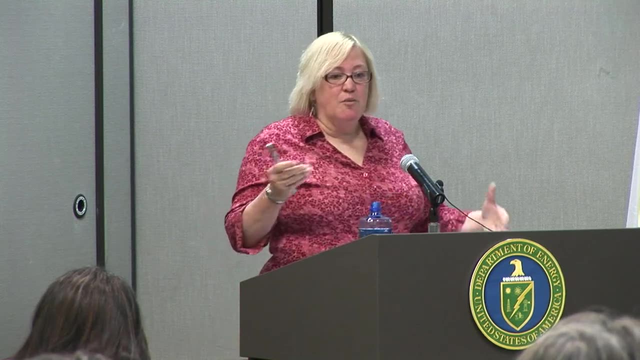 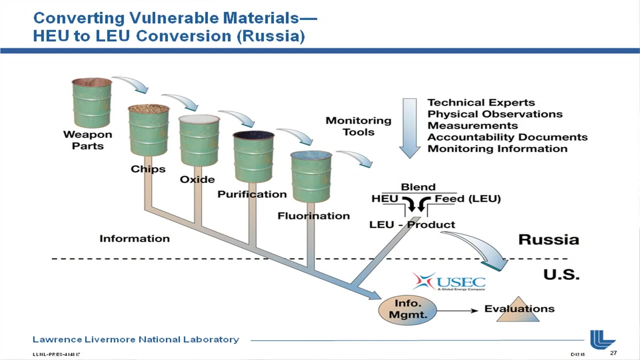 which is from their, from HEU, from their weapons stockpile. So what the to verify the implementation of this? again recalling: we don't, the US is buying this out the end. We do not have access to the complete process. 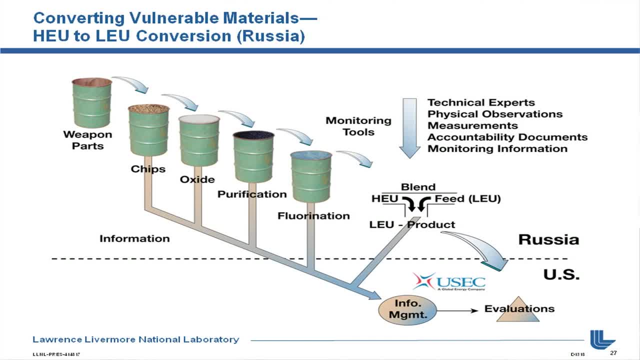 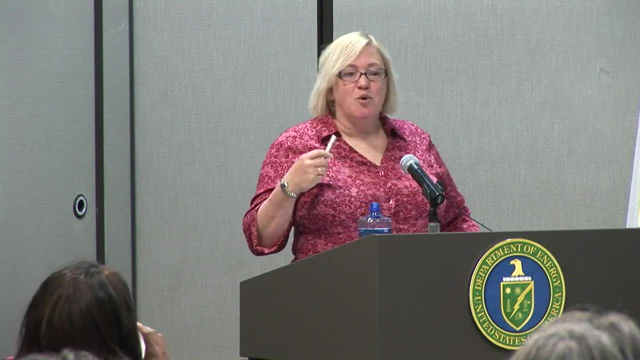 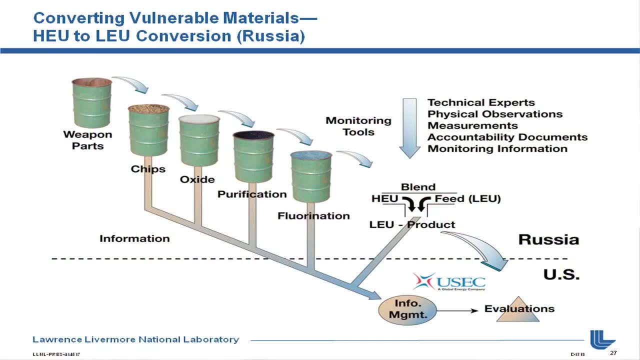 We have access to what the Russians and we have agreed to along that process, And the goal of this program is to assure the United States that what we're buying as LEU at the end process down here and then bring home and use in fact in nuclear power fuel. 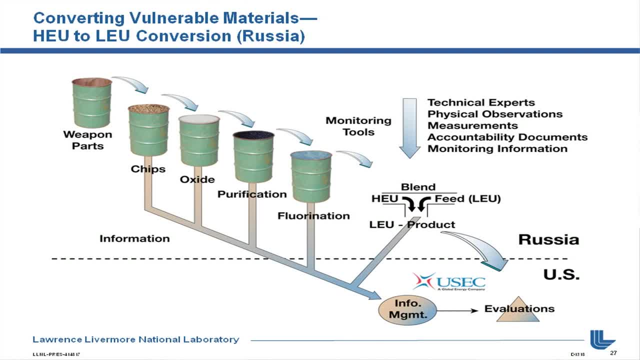 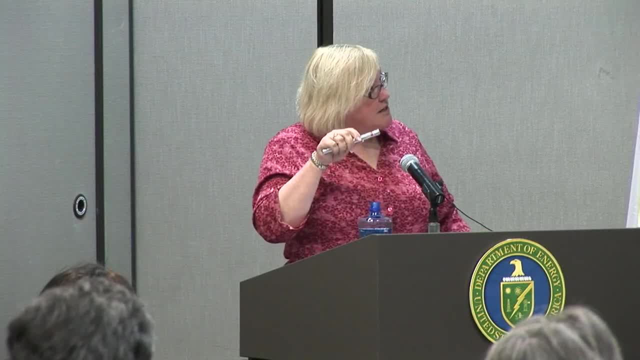 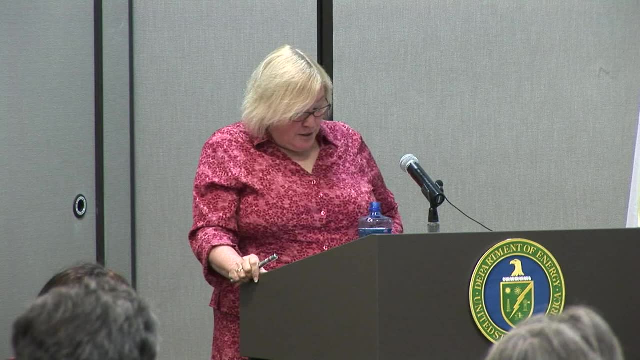 did indeed come from Russian weapons And that it was not being manufactured separately, blended down and the weapons were not being destroyed. That is the nature of the highly enriched uranium transparency project in the United States. You can see here some of the kinds of tools that they're using. 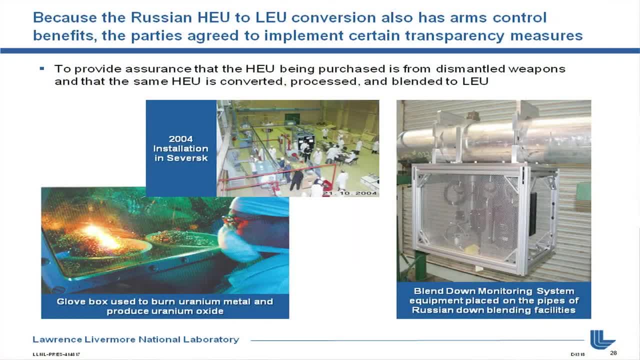 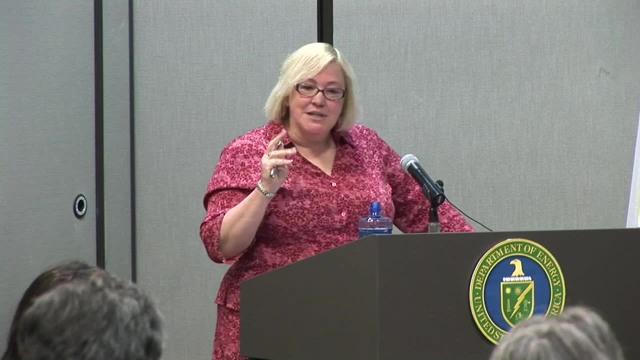 Because they have limited access to the facilities to assure that we are buying what we think we are. As an aside, because of the amount of uranium that we buy from the Russians and where we use it in our fuel cycle. one in, I think it's one in every ten light bulbs that is lit in the United States. 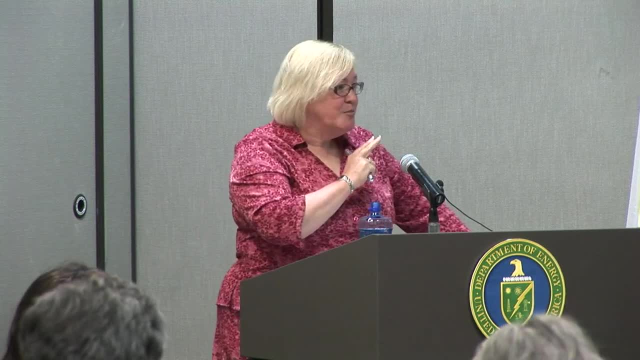 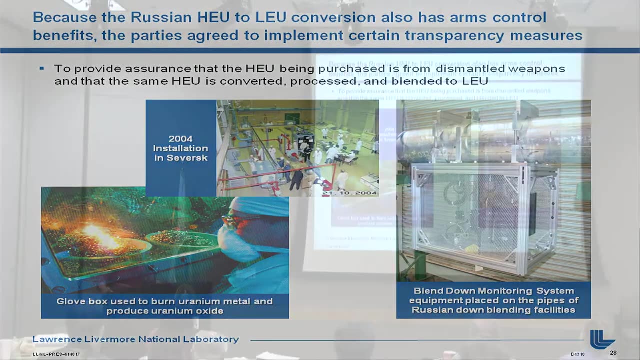 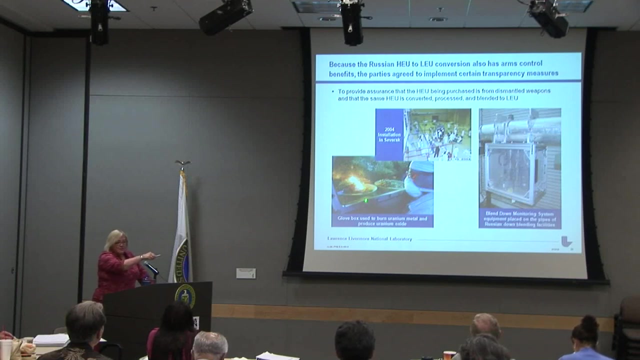 comes from Russian stockpile uranium, So you can see here where they put an installation into Zversk. what are the monitoring activities that this program undertakes? They have access to looking in the windows only of the glove box to watch the uranium metal being burned to perform activities. 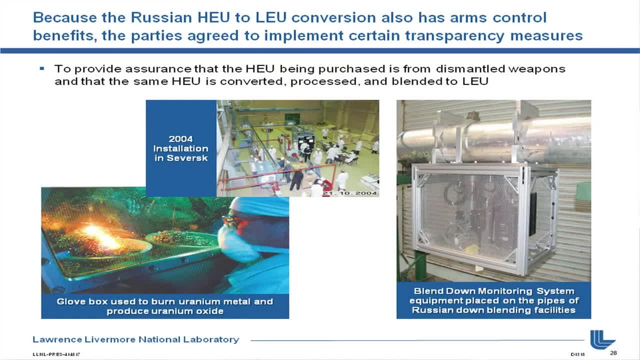 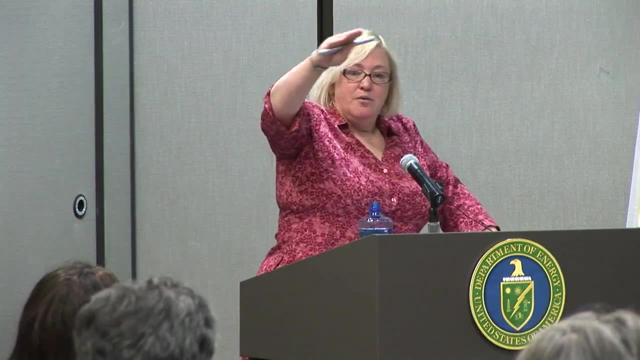 To convert it to the oxide. And then they have this monitor that they're allowed to strap on to the pipe, where that's the most access they have to information of where they're taking the highly enriched uranium feedstock from the weapons. blend down with your low enriched uranium. 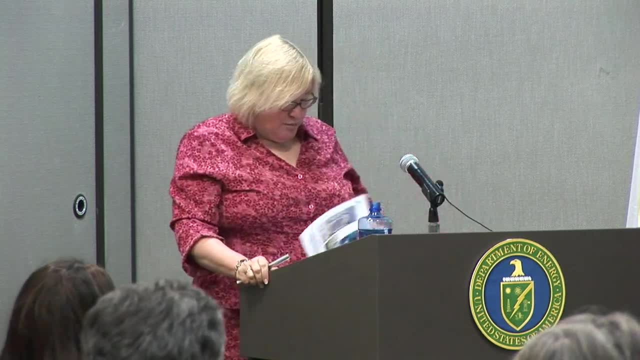 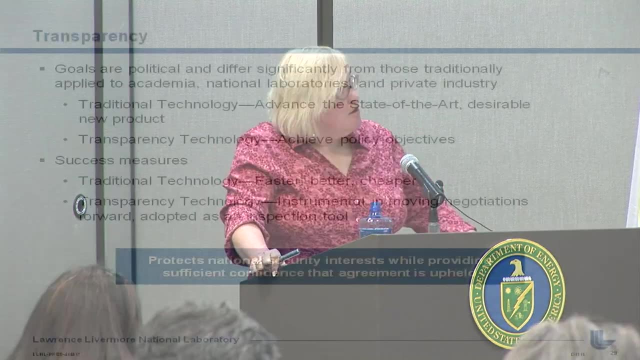 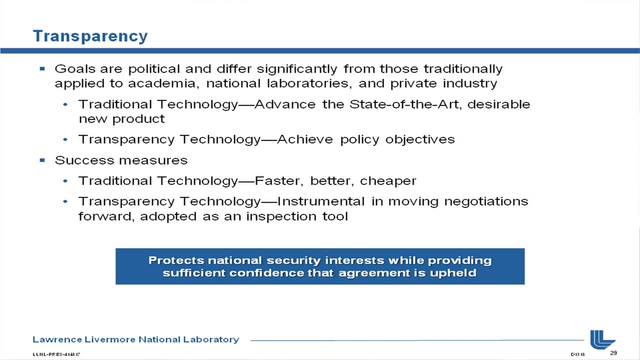 that they have to use to generate the product that the US buys. So we sort of alluded to the concept of transparency, That is, the ability for one country or the IAEA to see into what another country is doing in terms of their processes. 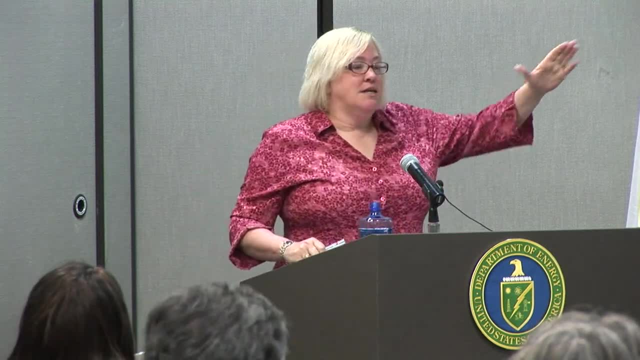 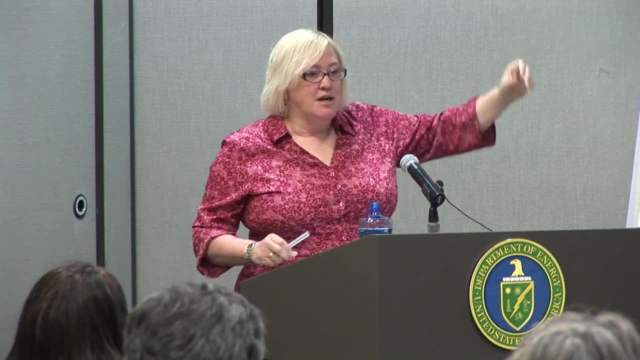 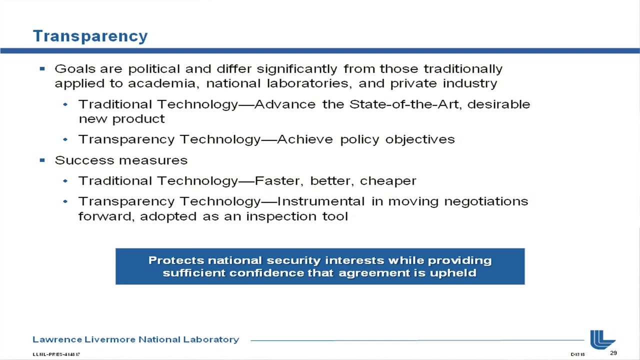 I bring this up here because for the scientists and engineers who work in this field, it has a different set of drivers than for many of the other scientific endeavors that we undertake. As trained scientists, we really like to advance the state of the art. 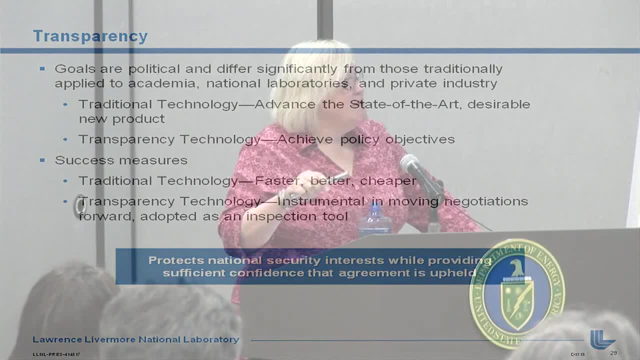 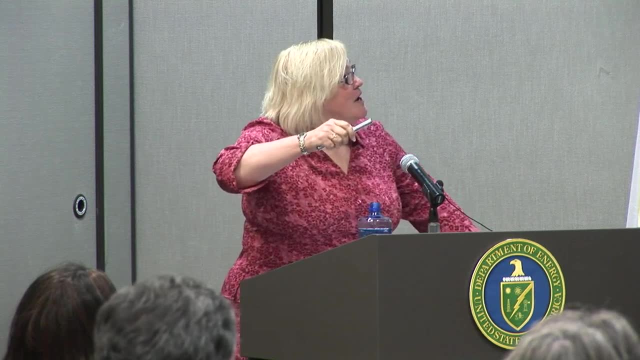 We like new widgets, We like to go faster, We like to go better, We like to go cheaper. That's what we were all trained to do. But in terms of technology, remember that the goal is to achieve the objective of the policy. 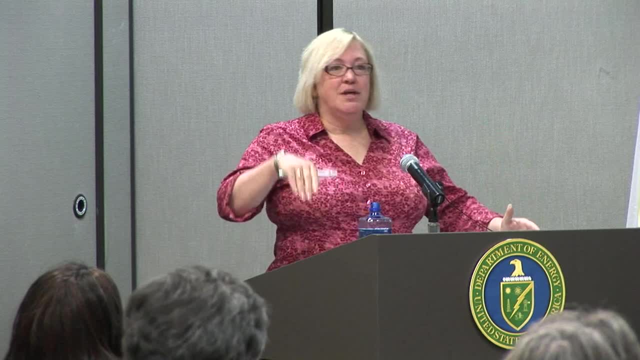 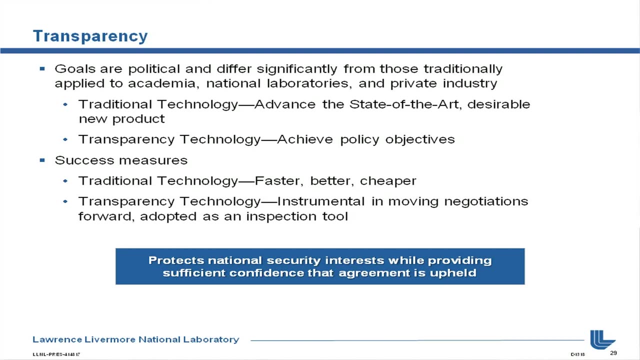 And sometimes that's just a yes or a no. Are they doing something, Are they not doing something? And it may not require all the bells and whistles and all the sophistication that we would like to put with it. Remember that the true purpose of technology. 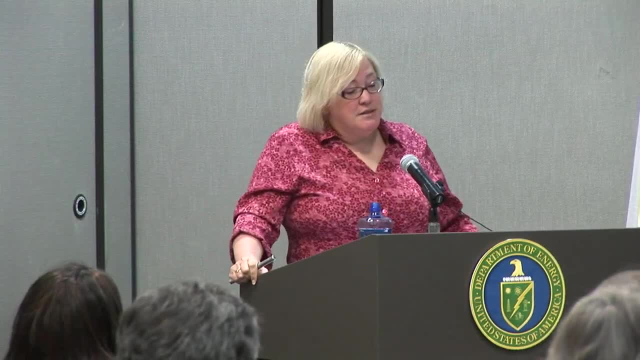 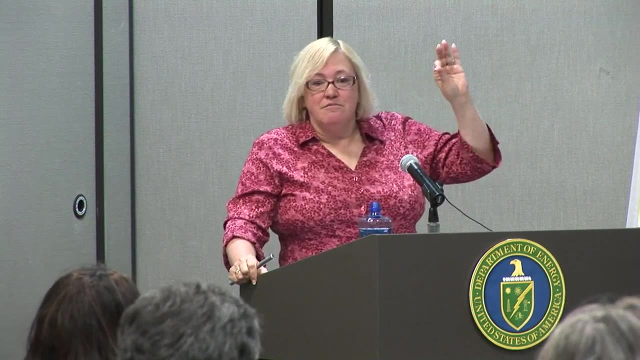 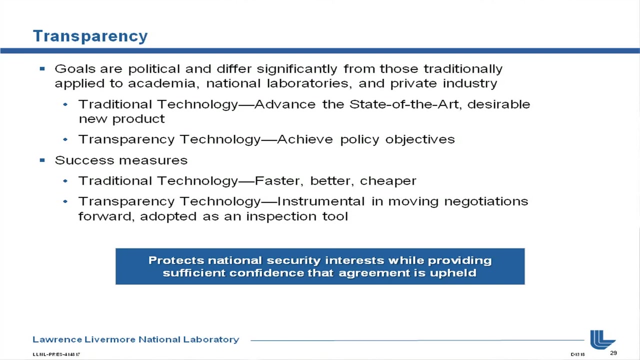 is that the technologies that we use in transparency and in verification are there to move negotiations forward. Negotiations get large discussions on what we're going to look for and what we're not going to look for, where and how we're going to look for it. 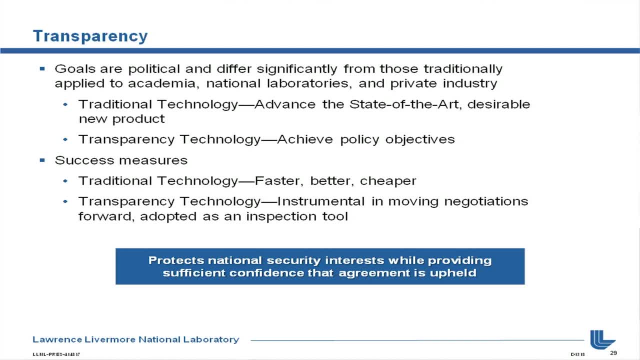 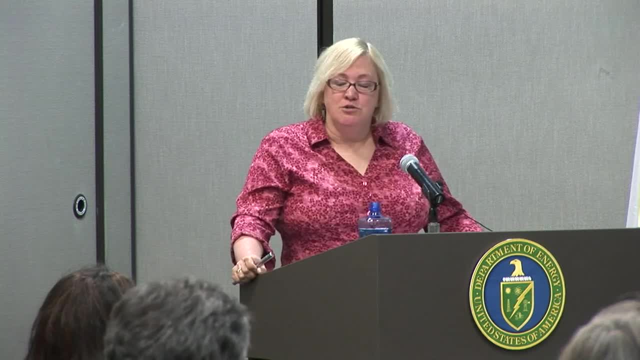 One of the new things that's under discussion with the New START program is: how will we verify what kind of verification regime will go with New START? Are we going to count warheads? Haven't done that before. We've counted delivery vehicles, right. 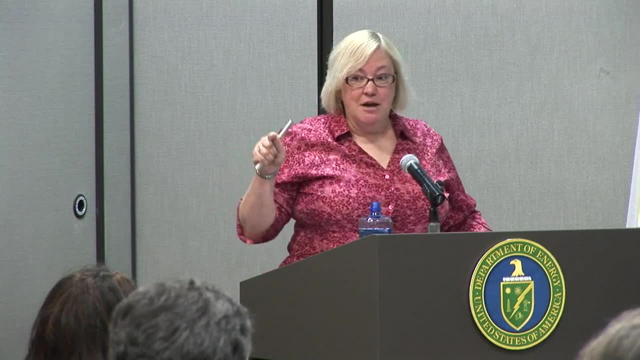 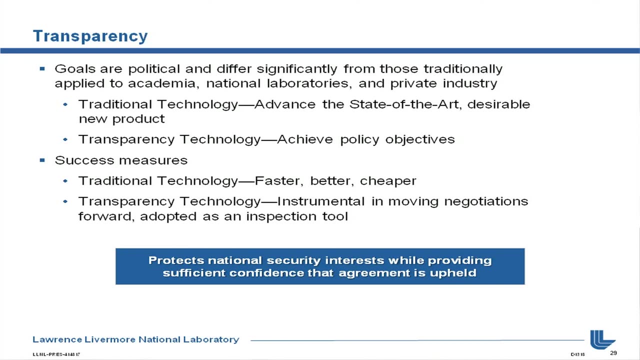 So we might move from counting missiles to counting warheads. Well, I don't think that anyone's going to open up the hood of their missiles so we can count how many warheads there are, because it's likely we wouldn't do that ourselves. 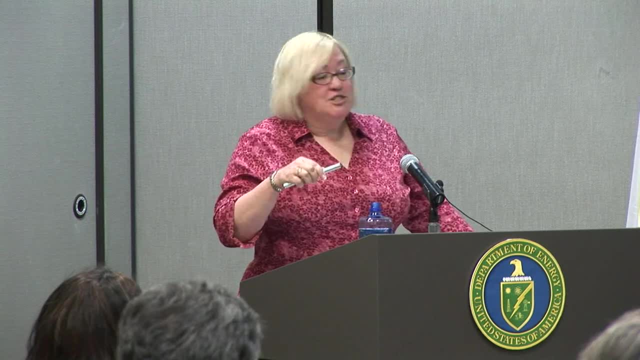 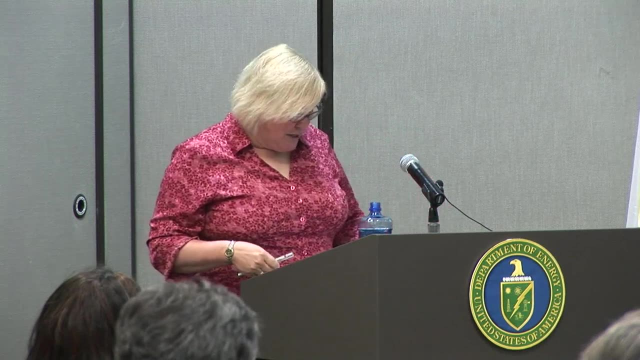 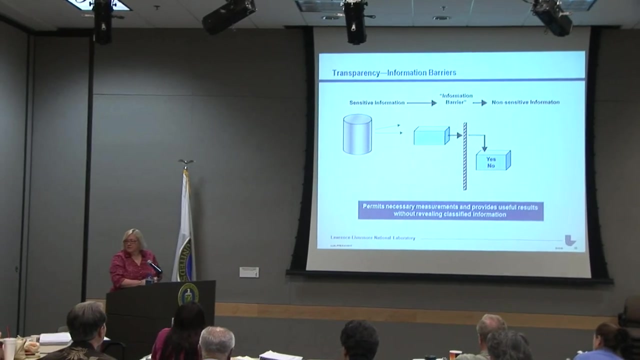 So there's a lot of technology challenge associated with how would you count warheads in a missile and retain- allow the Russians to retain their proprietary information. Excuse me, Yes, From your previous slide, we're buying the LOU from the Russians and paying for it. 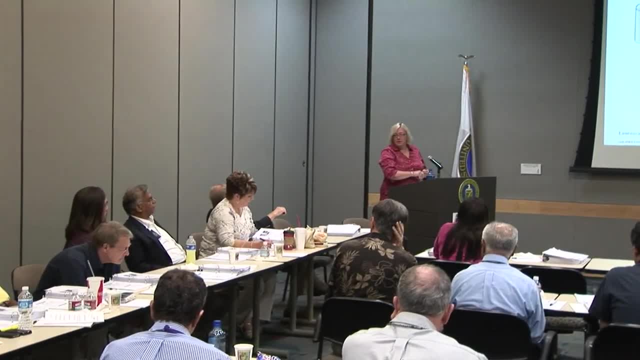 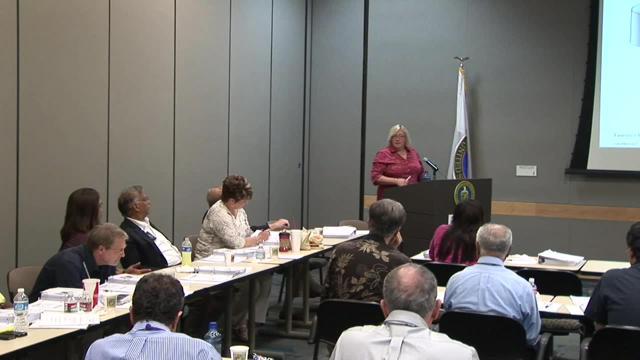 Yes, And then we in the next three years are going to get rid of the DOD stockpile of uranium, right? Yes, Will we make that money on it, Or how much is it costing us? So it depends on what the –, so the price –. 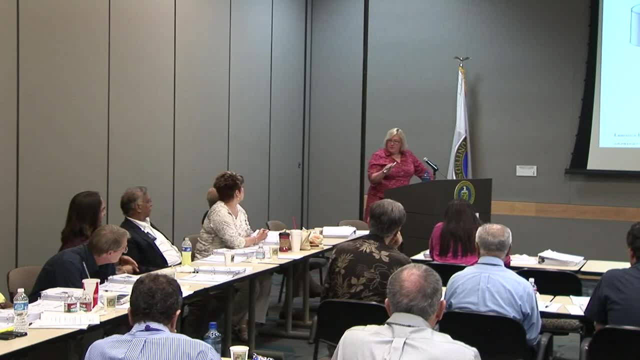 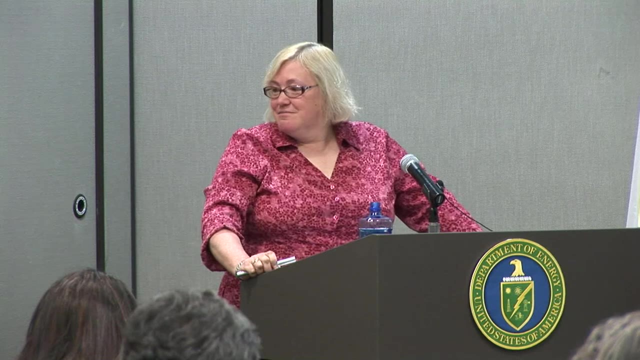 my understanding is the price of the uranium was agreed upon when they negotiated the – the bilateral agreement. The price of uranium goes up and down, So I don't know that there – you know, sometimes it's good news and sometimes it's not. 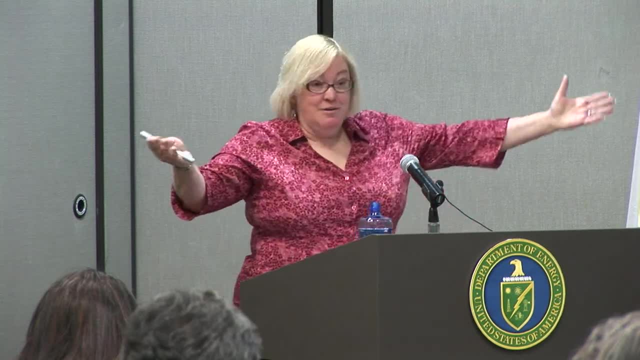 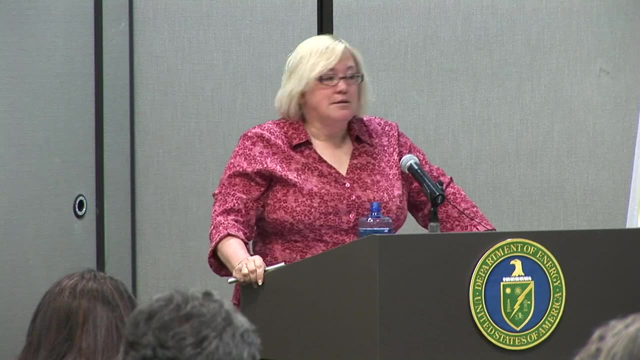 Does GAA know this or does anybody know? It's all – I mean, it's all out in the open what we pay for it and what the agreement was. You know there is – there's a lot of – that by definition. 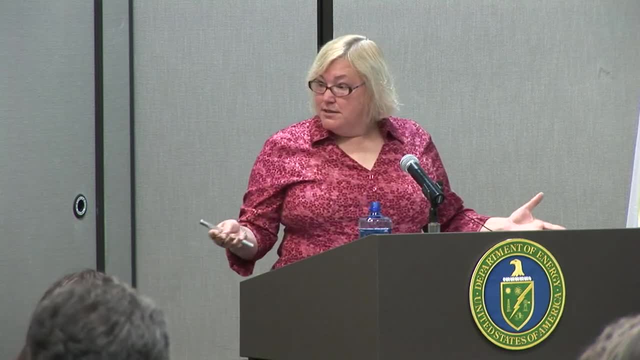 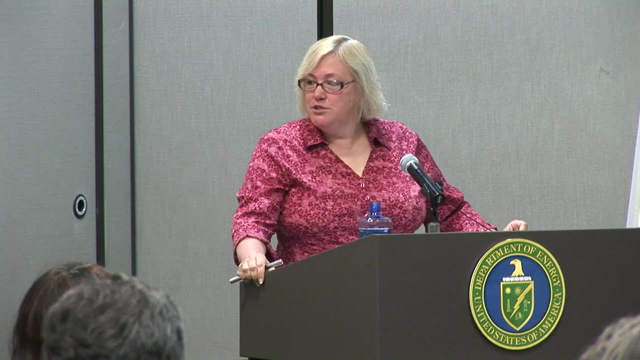 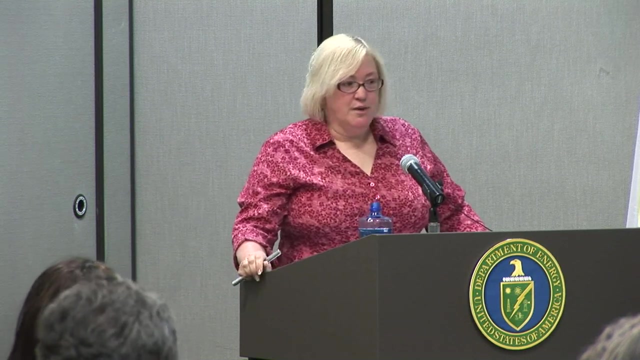 that program ends in 2012.. That was the end of the extent of the agreement And you know. so. there's preliminary discussions about does anyone want to extend it And a lot of the discussion about whether it would get extended, if I understand this correctly. 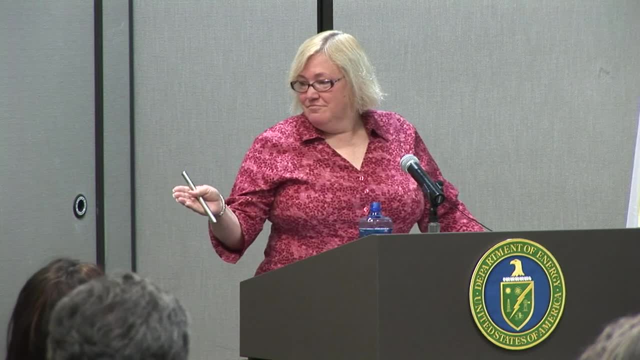 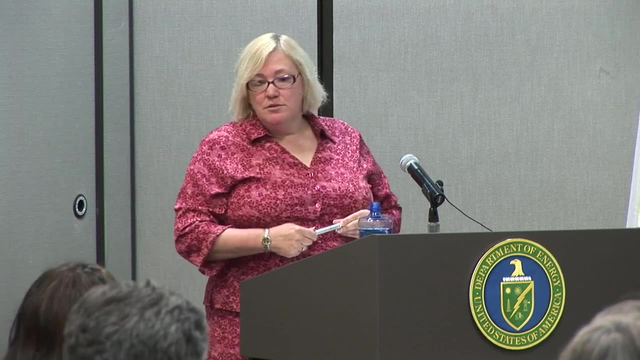 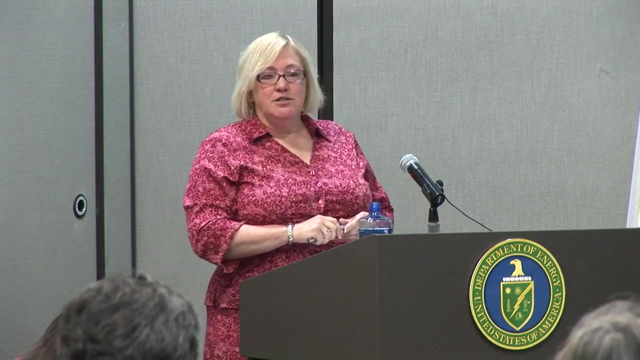 is what the Russians think they could sell the uranium for elsewhere, compliant with all the other treaties. So this is my last slide, and that was just again to talk about the concept of maintaining the safeguards, confidentiality and how you transfer information about a highly sophisticated 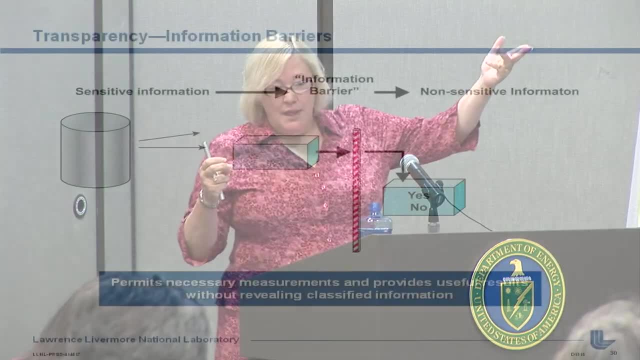 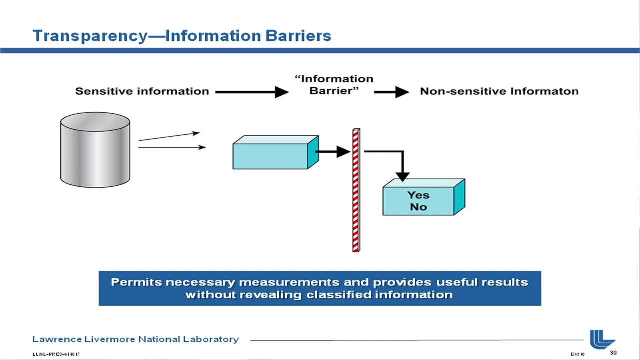 highly complicated process out to the other end through something that's called an information barrier, And that's how do you take all of the information that you have and get a yes or no out the end. We've talked about that in terms of a couple places. 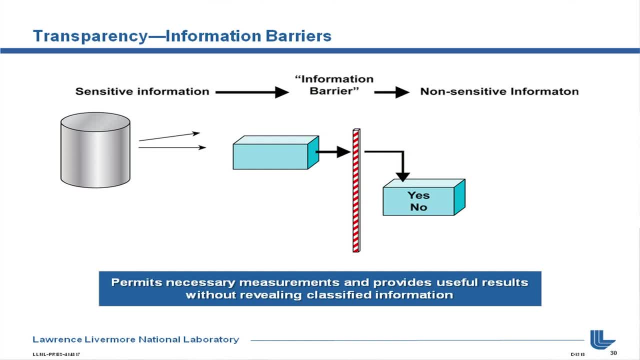 where that's an important thing- This is actually an active area of research- is: what does an information barrier look like and how do you implement it? So that finishes what I had prepared to say. I'll be happy to try to answer any questions anybody might have. 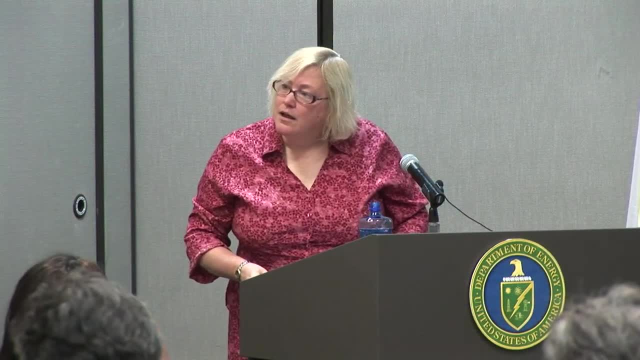 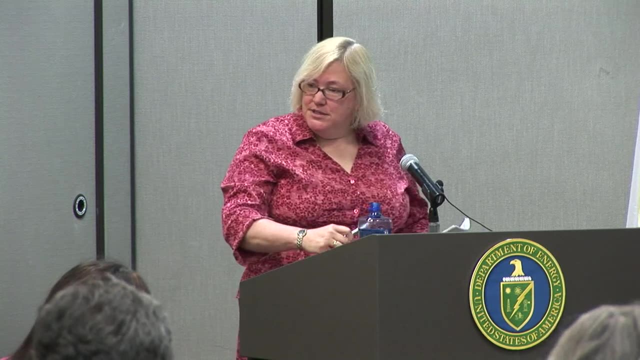 I have a question: Where does the IAEA pay their funding? So, because member nations contribute to it, we pay through our membership. the United States is a member through the State Department in ways similar to the United Nations, But it is used. 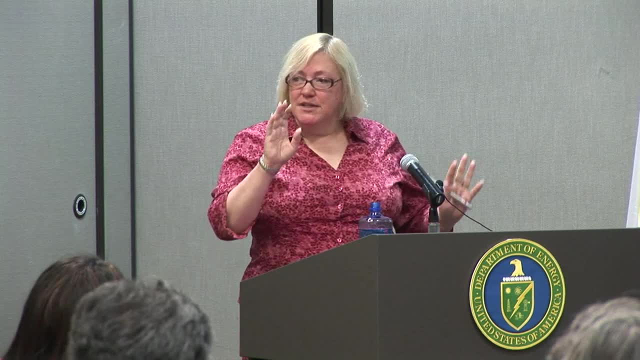 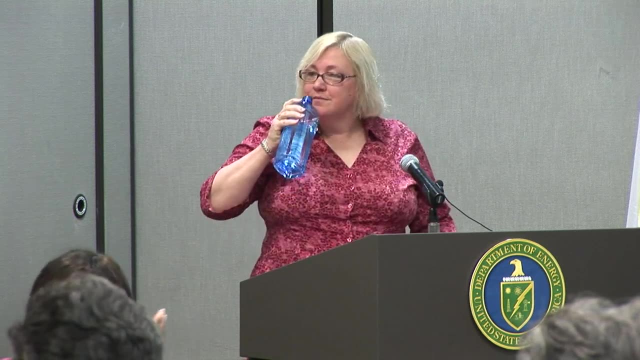 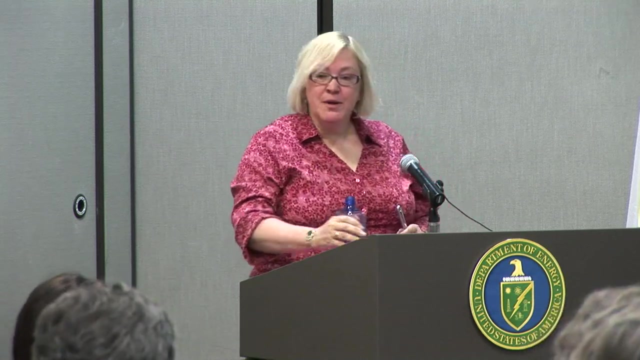 It has a special relationship because I think not everybody is a member of both. Ted Turner pays too, right. Ted Turner pays, right. I don't contribute a bunch of money. Does the IAEA have any jurisdiction over the non-member countries? 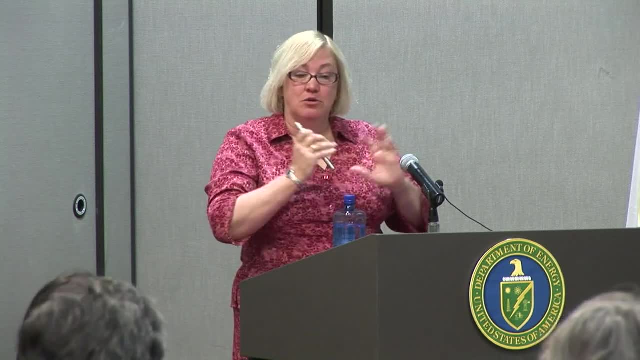 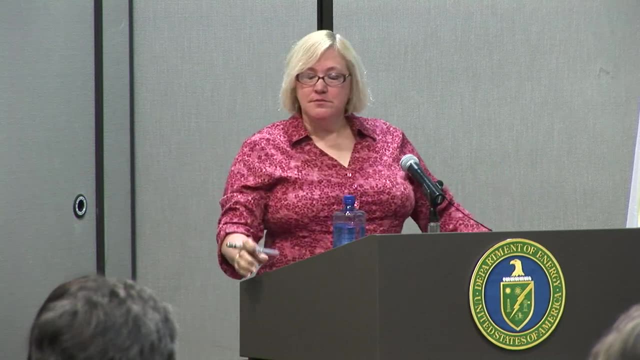 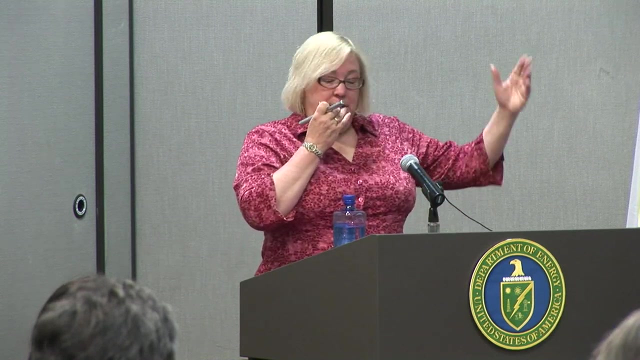 or do they have to make it back to the UN? They have no jurisdiction to take even non-compliance from countries that are not members. They're invisible. They haven't agreed to comply. I mean, you've seen that played out Well. you saw the list of non-compliance. 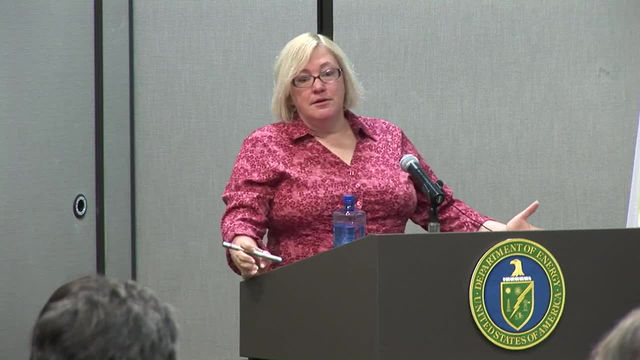 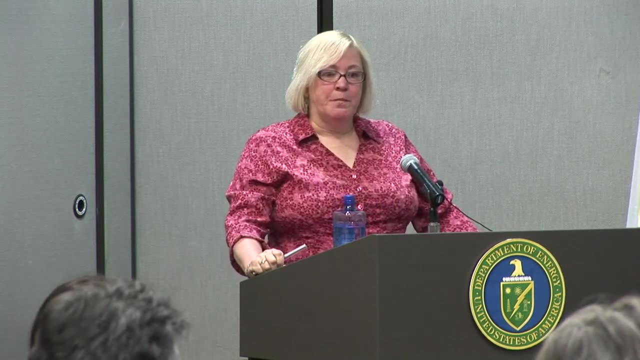 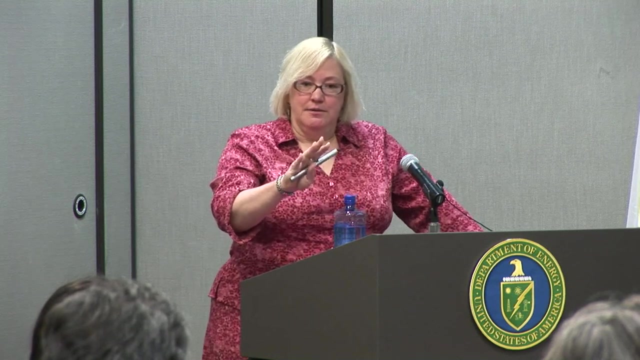 You've seen it probably most visibly in the news in North Korea. But they discuss like North Korea, like their Board of Governors. So, without going into a lot of details, there's questions about whether North Korea can legally come out of the treaty or not.